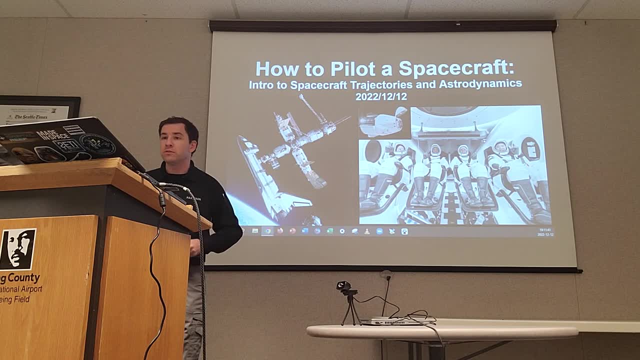 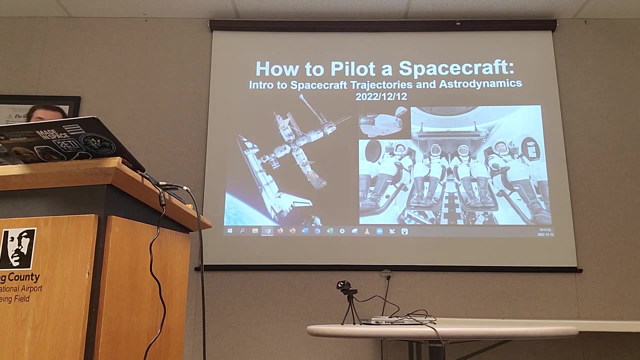 I hope you'll notice some common, some some overlap and some common terminology. It's it's a very interesting discipline because, with the possible exception of propulsion, astrodynamics is really the only branch of aerospace engineering where there isn't really an analog to the other, to the other engineering branches. 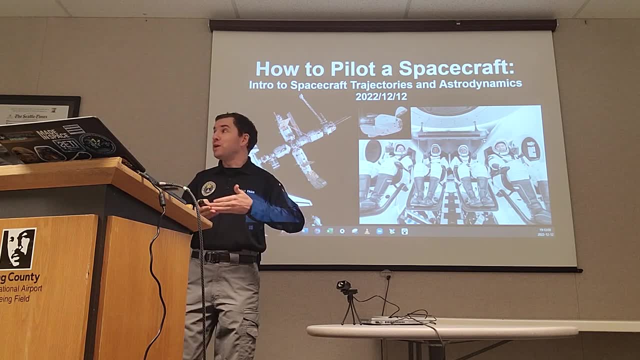 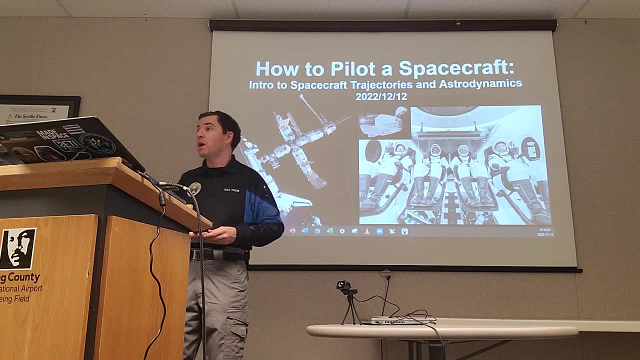 If you are a software engineer, doing aerospace software is pretty similar to doing air, to doing software in another engineering discipline. You're just doing it to a higher quality assurance standard. You're doing structural engineering or vibroacoustic engineering. It's very similar in aerospace as it is in other disciplines. 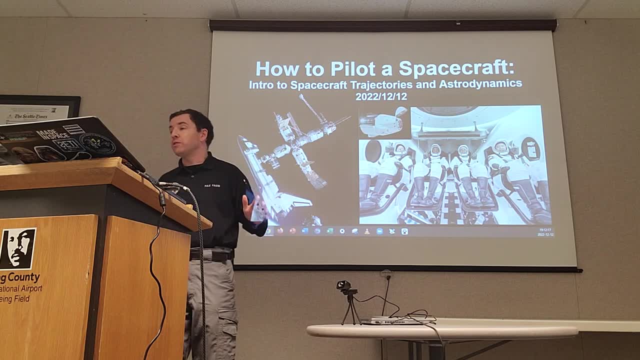 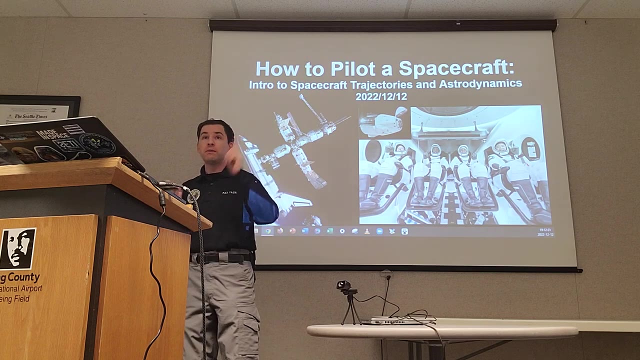 But astrodynamics is its own beast. It's very different. The dynamics of an orbit are completely different from the dynamics of a car or an aircraft or something that we're more familiar with in our everyday study. And most of the critical limits on space missions- payloads, thermal communications, duration, consumables- 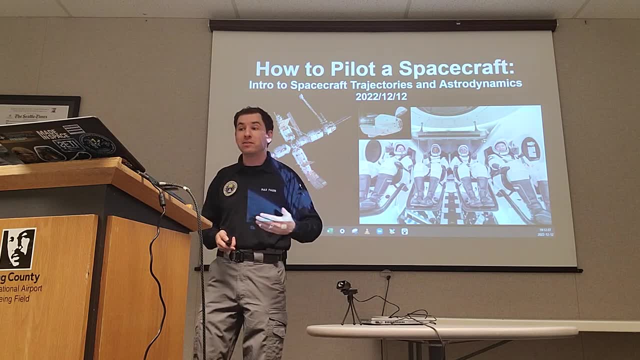 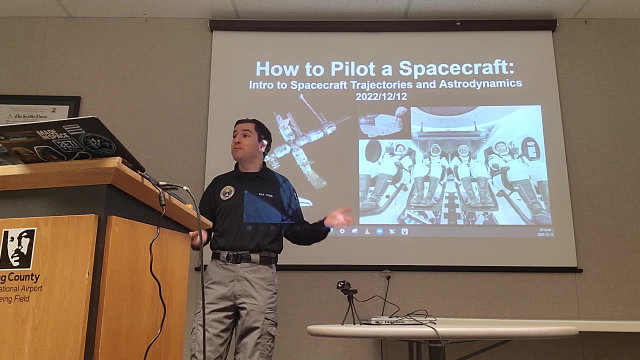 Most of those things can be tied back to an astrodynamics limit, So it's a very important starting place When you're doing the spacecraft design. And unfortunately, most of the terminology that we're going to be covering tonight was invented by the ancient Greeks, with most of the math invented in the 17th century. 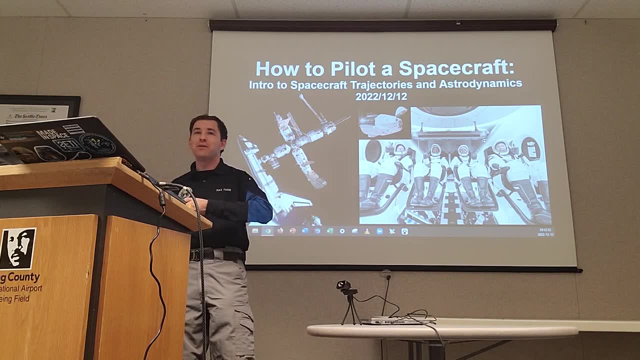 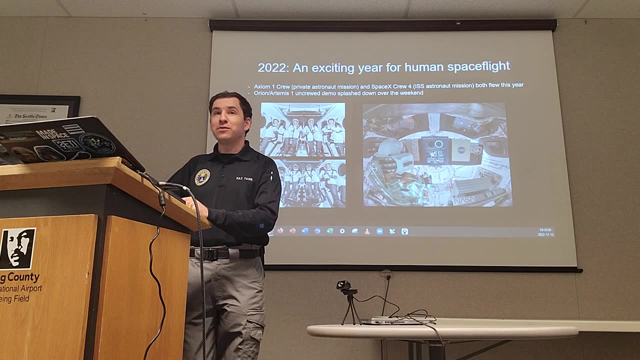 So we're kind of stuck with some anachronisms and some modern terms which kind of make it a very weird thing to talk about. So it's been a very exciting year in spaceflight this year. Every year for the past decade or so has been an exciting one for human spaceflight. There were two crewed SpaceX visits to the International Space Station, The Axiom 1. A private astronaut mission, And the NASA Crew-4.. And just this week, as I'm sure you're aware, the Orion spacecraft, the Artemis 1 mission, came back from its trans-lunar flight around the moon. 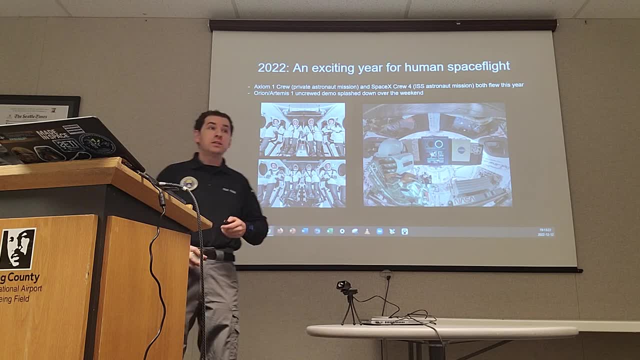 Spending about 25 days in orbit, No pilot on board, But accommodations for four astronauts, including this mannequin right here to demonstrate the viability of the vehicle. For uh, Don't they have two other mannequins? Say again. 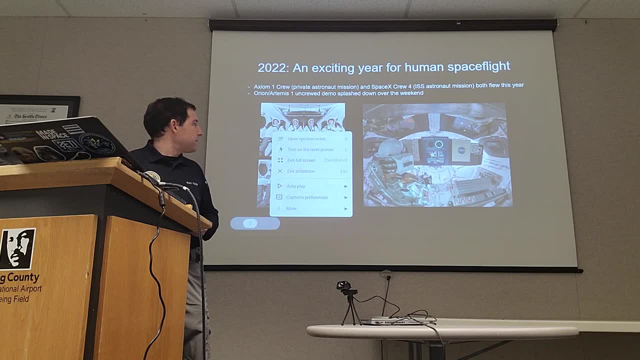 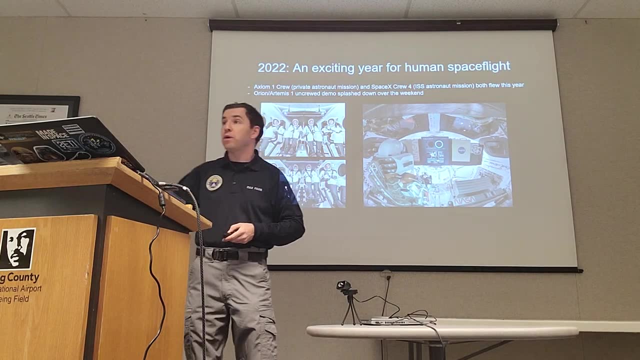 Don't they have two other mannequins? I believe they did So. I think they had an anatomical female and an anatomical male to study radiation dosage throughout the body. What's giant windows? These are windows Right here and right here. 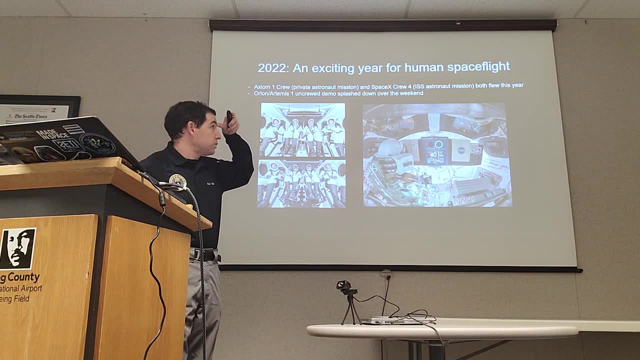 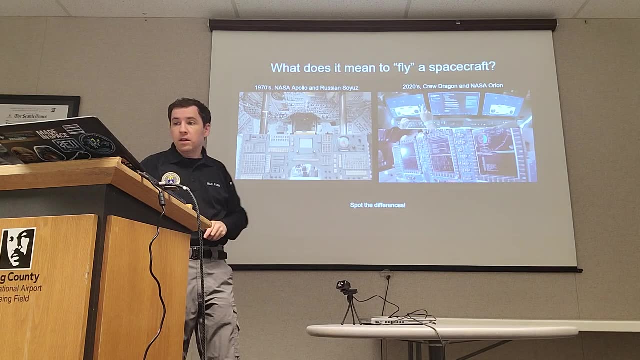 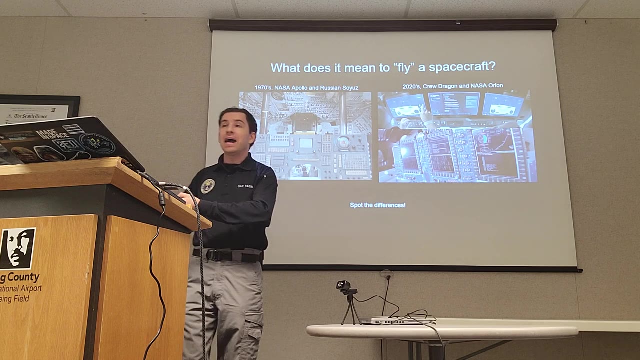 As well as right here, and right here They have different functions for docking and ascent. Yeah, that's what those four are right there. So the, The internal structure And how we interface a pilot with a spacecraft has changed a lot in the last decade. 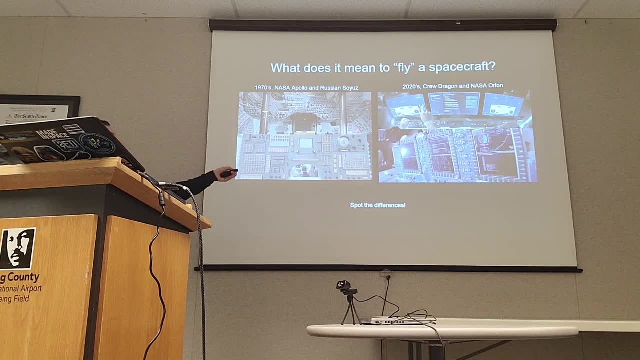 Just here you can spot the difference. Here on the left, this is the Apollo and Russian Soyuz. This is kind of what you see in the Apollo and the Russian Soyuz Analog. There's one button, one function. There's no digital displays. 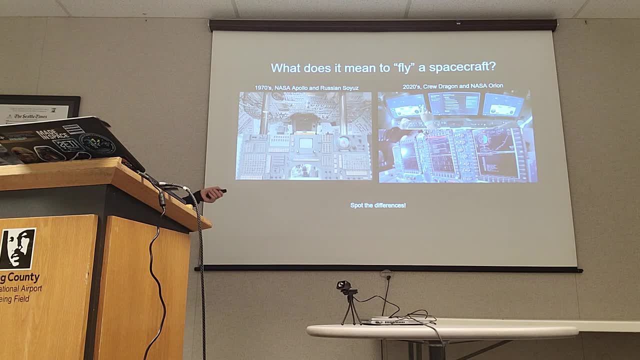 Contrast that with what you're seeing in modern displays. Up here, this is the SpaceX Crew Dragon And down here is the Orion capsule. There's a combination of physical inputs as well as multi-functional inputs, Which can be a lot more information-rich than it could in the past. 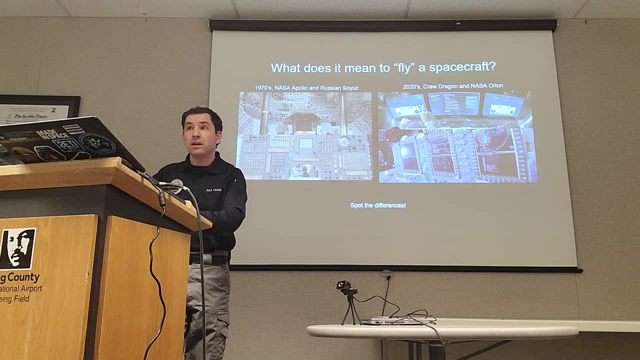 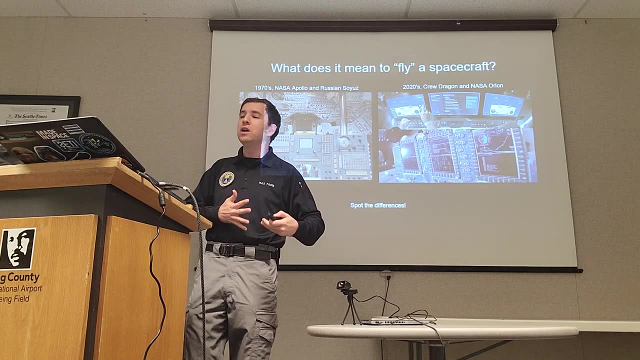 But it also means a lot more of the functionality is automated And a lot more of it has been put between another layer of abstraction, between the human and the vehicle that they are flying. So what does it even really mean to fly a spacecraft anymore in this new world? 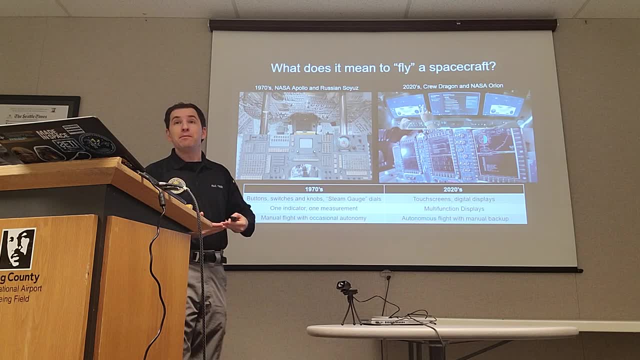 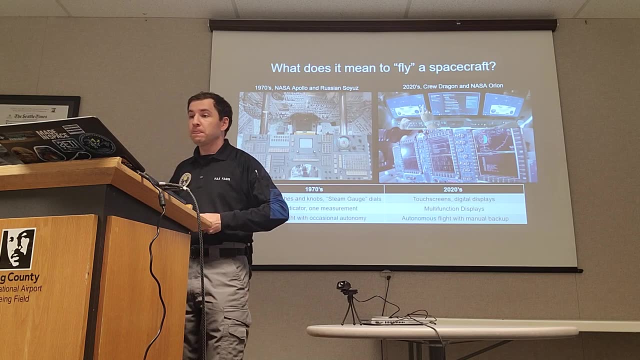 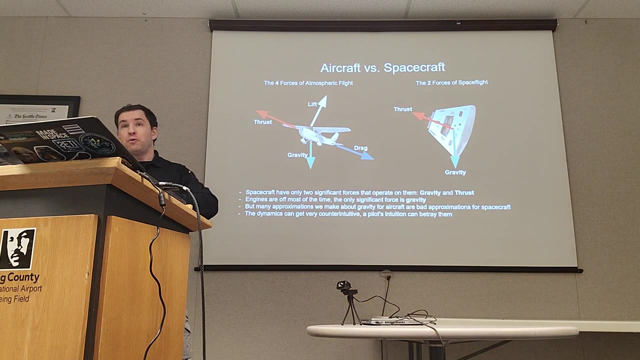 Because it still requires an immense amount of skill, But it's not the kind of seat-of-the-pants airmanship that we're used to thinking about when we're flying a Cessna 182.. The forces that operate on a spacecraft do have some analogs to the forces that we're familiar with thinking about on an aircraft. 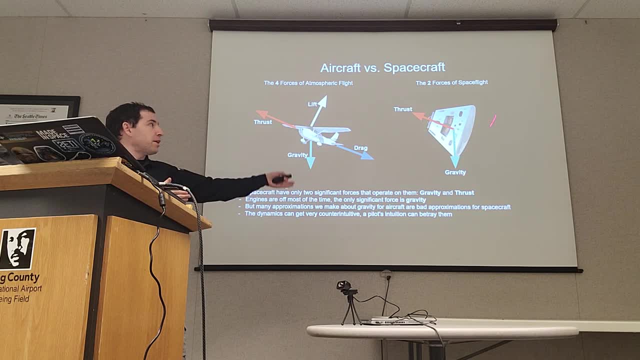 Four forces of flight. Only two of them are ever really present on a spacecraft. that's in orbital motion, Thrust and gravity. There are other forces: Solar radiation pressure, for example, The light pressure from the sun, And aerodynamic drag is still present, even in orbit. But it's measured on the scale of micropascals instead of kilopascals. So the actual dynamic pressure from atmospheric drag in space we tend to ignore. Same thing with light pressure, leaving us with really only these two important forces. Thrust and gravity And most spacecraft. their thrusters are off 99.9% of the time on light and dimensional aircraft, So you can model it as the same force as you would for an aircraft with no air and no engine. That's a considerably simpler, dynamic model. 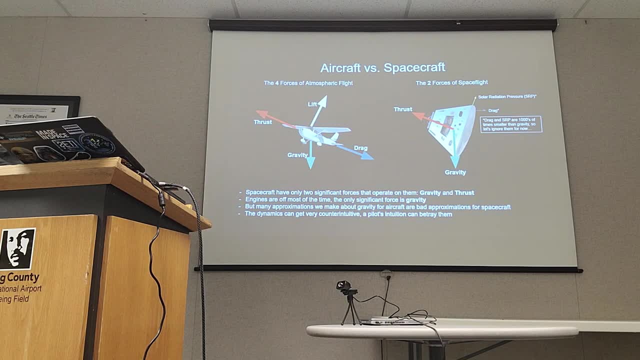 However, the fact that we're not working in a conventional Cartesian space where it's just forward, backward, left, right up down, complicates things. Spacecraft are moving so rapidly that you can't ignore the curvature of the Earth. 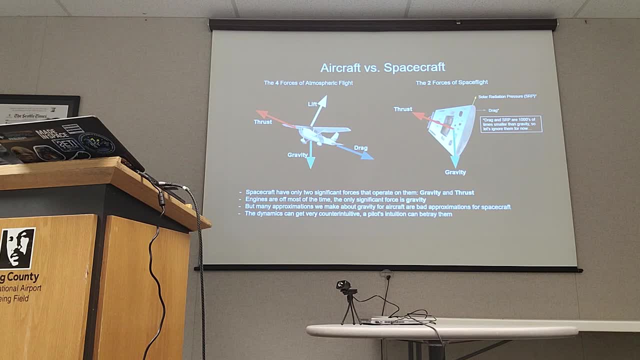 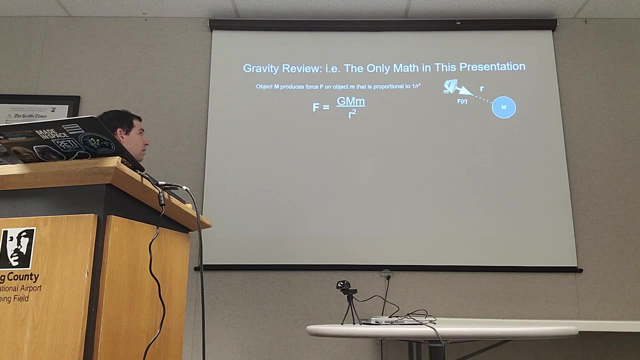 And talking about up and down is a lot more subtle than it is when we're talking about an aircraft, And that leads to different terminology and different ways that we have to handle the dynamics here. So let's go through the math roughly. This is the only math in this presentation, I promise. 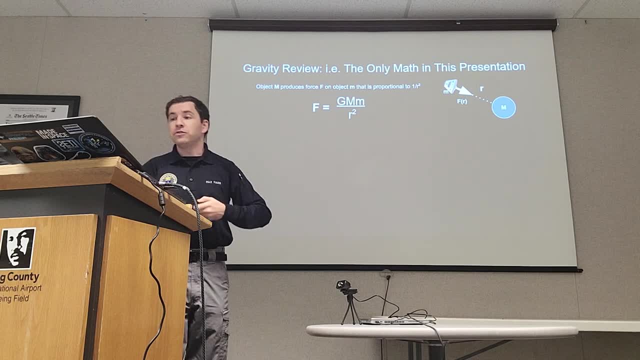 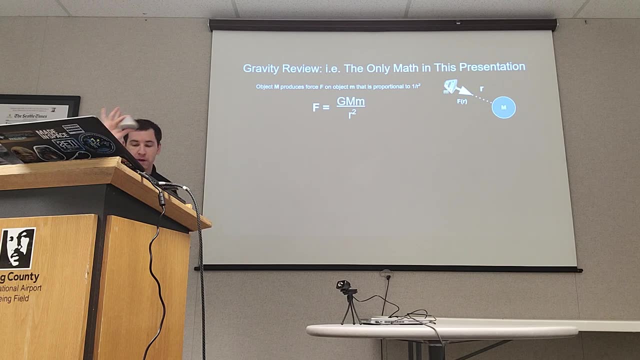 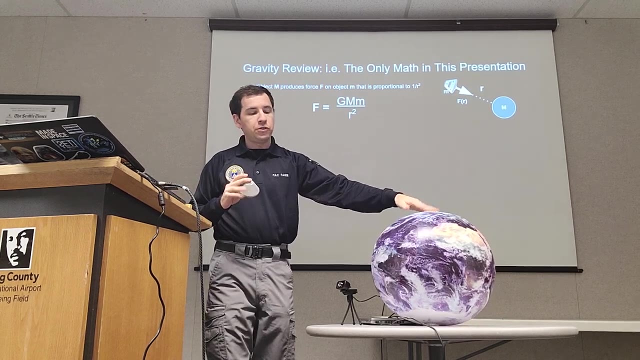 The law of gravity that we're all familiar with from high school states, just that gravity is inversely proportional to the square of the distance, the square of the separation between two bodies, so spacecraft and the planet that it is orbiting. Force of gravity is in direct proportion to the product of the masses of these two objects. 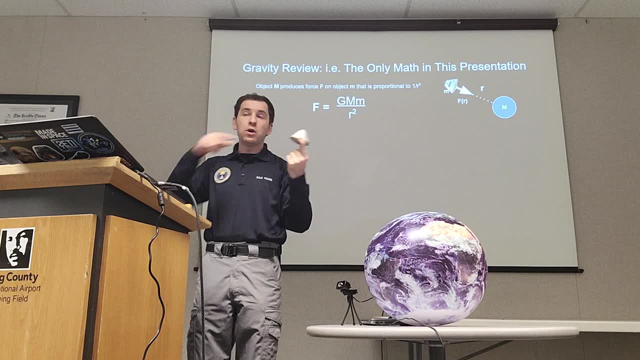 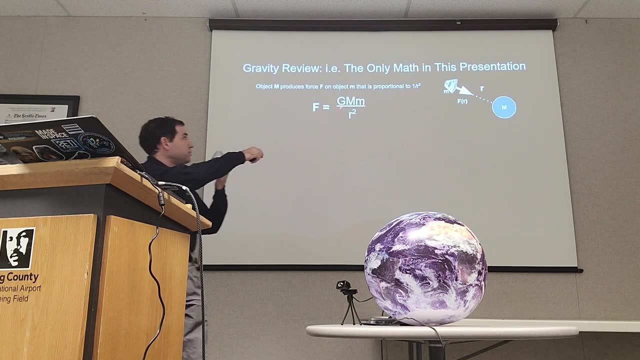 and inversely proportional to the square of the distance between them. That's the only force that's operating on a spacecraft substantially for most of the time that it's really flying. So the force of gravity, Newton's gravitational constant times, the product of the masses over the square of the radius. 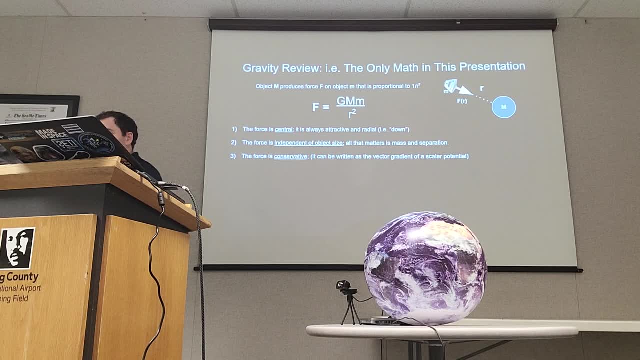 Now there's a couple of important things that can be derived just from this simple law alone. The first one is that the definition of down depends on your physical location. It's always central. Force of gravity is always towards the center of the planet. It's independent of the size of both objects. The mass is important, but if the Earth had the same mass and was just a larger planet without getting more massive, the orbital motion of a spacecraft would be different. A spacecraft around the Earth would still be exactly the same. 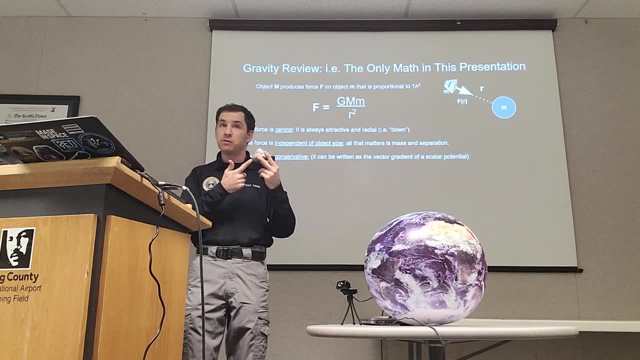 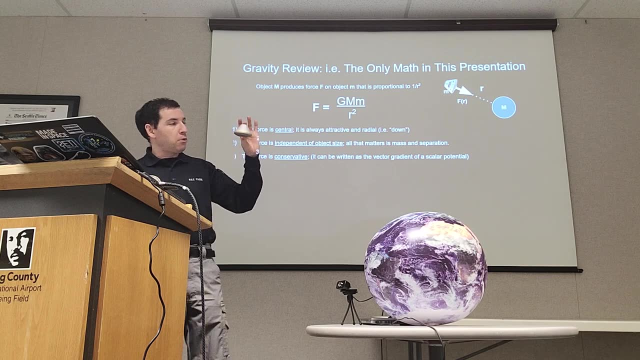 It also doesn't matter what shape your spacecraft is. It only matters what is the mass of the spacecraft. So that's a good simplification that helps simplify a lot of our discussion here. And of equal importance is the fact that the force, the force of gravity, is what we call conservative. 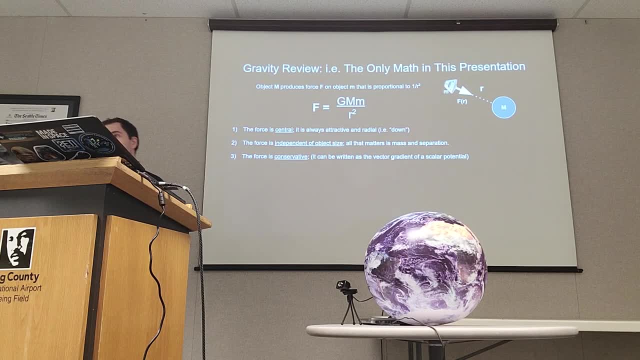 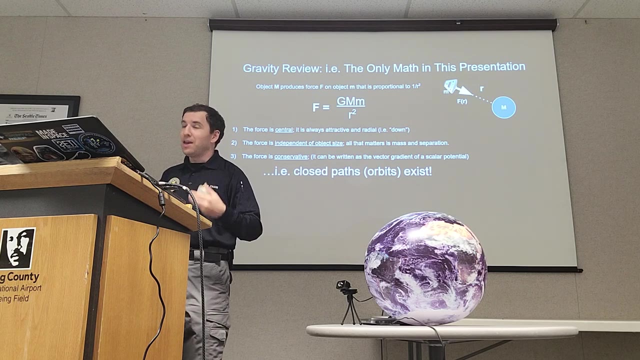 meaning that it's path independent. If you remember your vector calculus, it means we can write gravitational force as the vector gradient of some scalar potential. But the takeaway from that is closed paths exist. Any object that is moving only under the force of a conservative force. where you can write it as the vector gradient of a scalar potential must have closed paths of motion, which, in this case, we already know because we know orbits exist. I mean this is true of any inverse square force. So it's convenient that the universe came down this way. 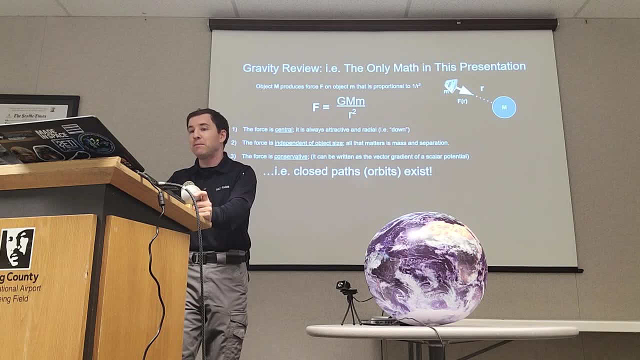 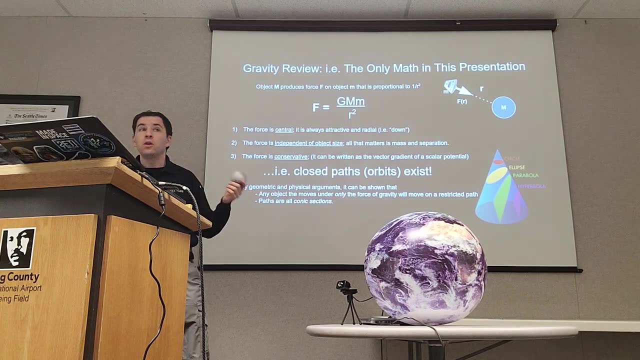 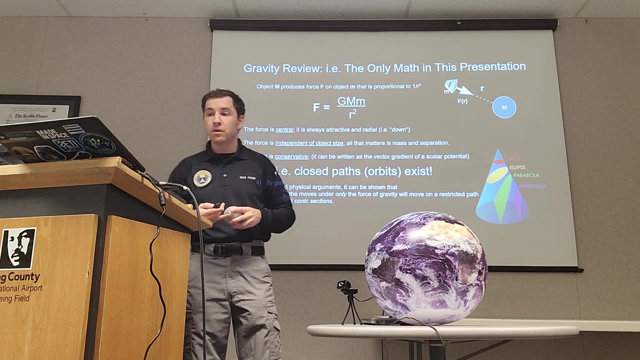 or else there'd be no way to do closed path motions around planets which we find so useful. Yeah, so these closed paths orbits can only take on a certain number of shapes and we capitalize on the uses of these shapes for different applications, depending on the spacecraft. 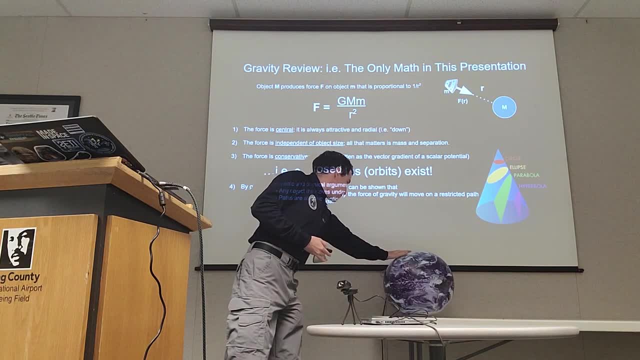 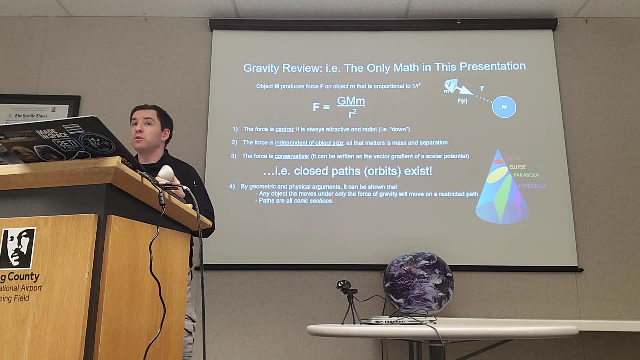 So it was known early in the Renaissance era that these closed paths. if you go through the mathematical derivation using the law of gravity and ask what are these closed paths, It turns out that they can only take the form of what we call conic sections. 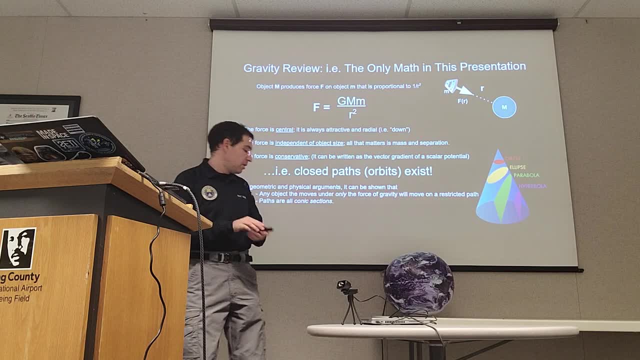 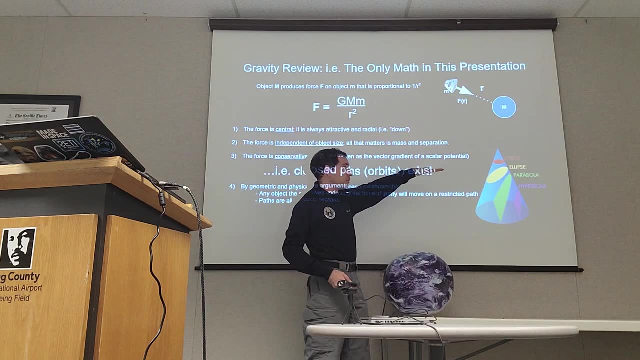 Conic section is what you get if you take a cone, a three-dimensional cone, and you cut with a plane. If the plane is parallel to the cone, like this one cutting straight through the cone, then the cross-sectional surface that you get when you look at what the intersection between the plane and the cone is. 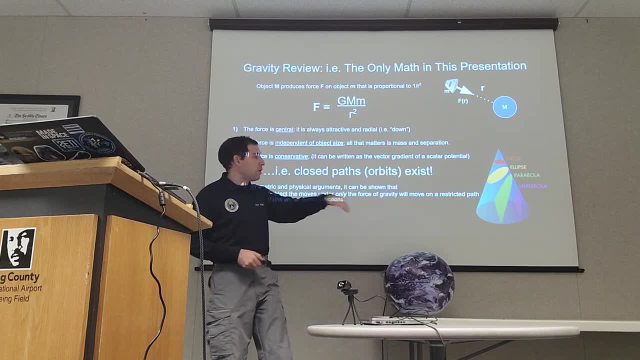 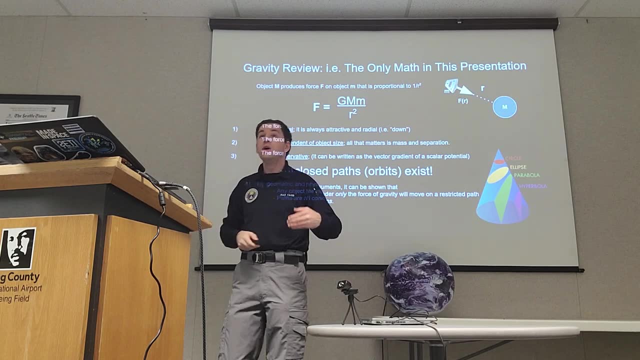 is a circle, a circular orbit, But there's no reason you have to cut the cone in that direction. You can cut it angular, you can cut it sharper, you can cut it vertical. All of those shapes, any of those shapes, are a valid orbit, operating under this assumption. 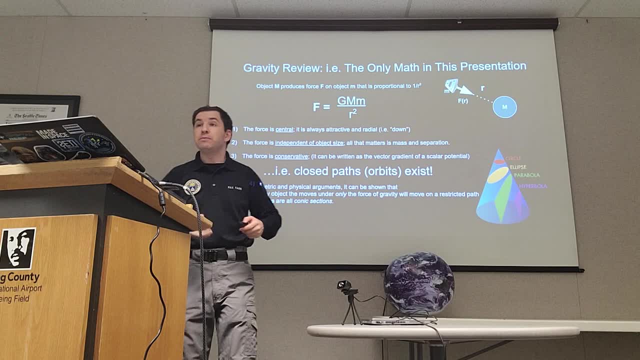 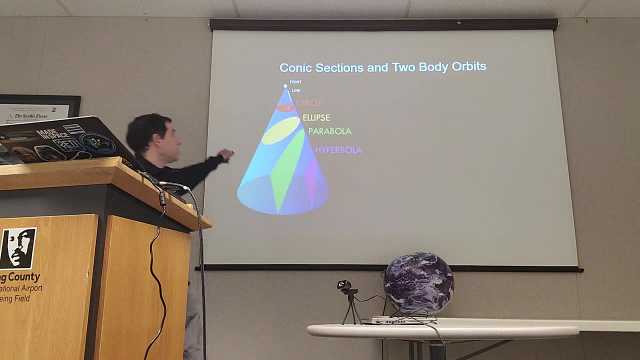 So orbits can't take any shape. they can only take a limited number of shapes, and each of those orbits has different applications depending on the type of spacecraft that we are flying. So the five classical kinds that we talked about are the degenerates. the point and the line. 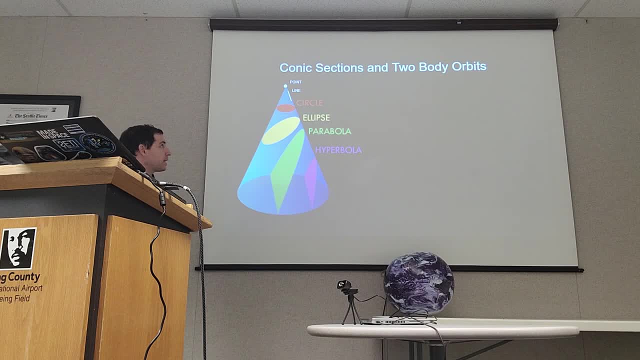 circle, parabola and hyperbola. Those are the categories of orbits that we can typically get. The two degenerate cases here are kind of uninteresting cases If you cut the cone directly, directly at its apex. so the intersection between the cone and the plane is just a point. 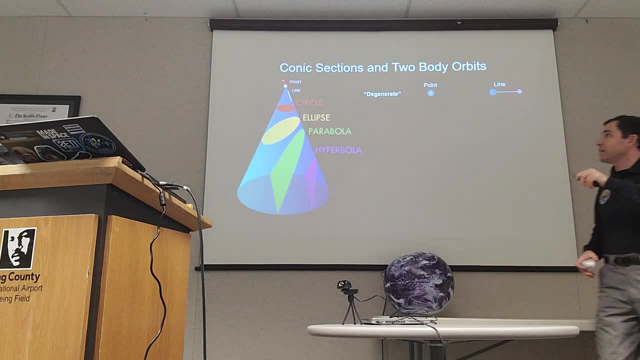 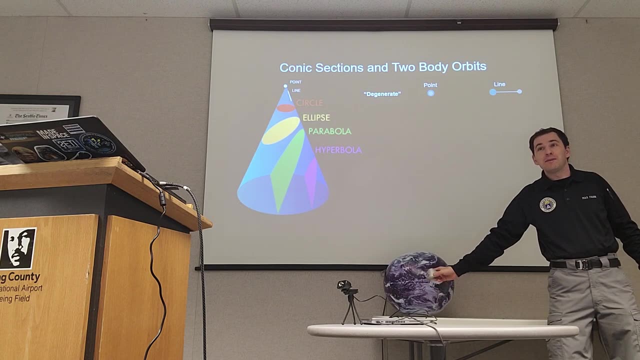 then this itself is technically a valid orbit. What does this represent? Well, this represents a satellite hovering in the middle of the Earth. Newton's law doesn't know anything about the surface of the Earth. It only cares about the masses. And as far as Newton's law, as far as the law of gravity is concerned, 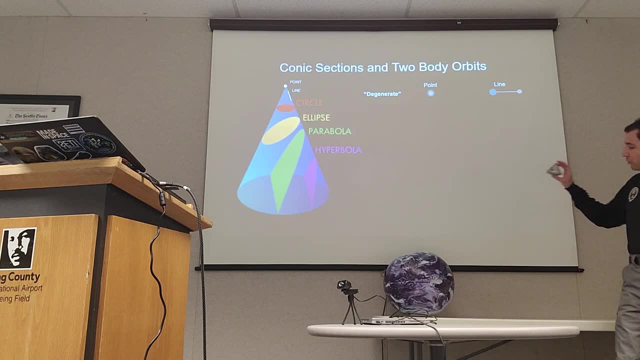 a valid orbit is just hovering right in the center of the Earth, But you can also just be falling straight down towards the planet. Those are what we call the degenerate cases, point and a line. But they're technically valid orbits. There's nothing mathematically invalid about that. 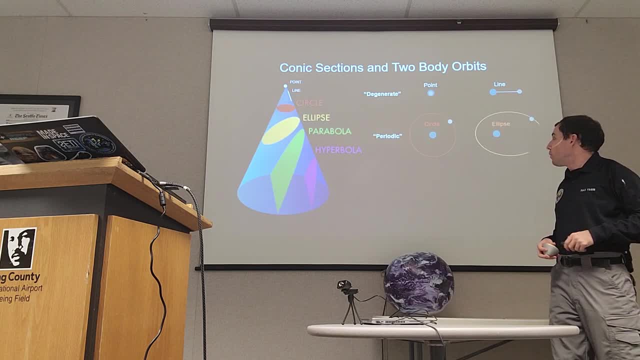 There's just not a lot you can do that's interesting with them. The more interesting ones are what we call the periodic cases. So there's the circular orbit, where you cross through the cone directly parallel to the base of the cone, and the ellipse, where you take a cut at an angle. 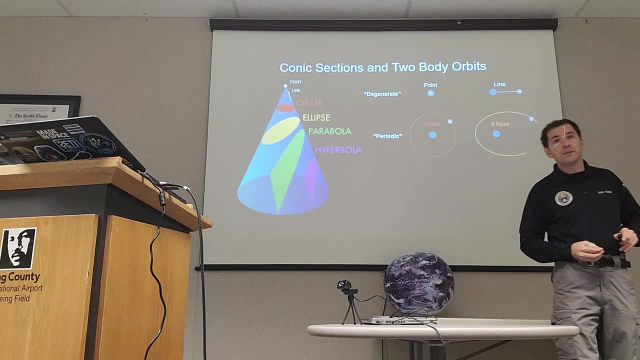 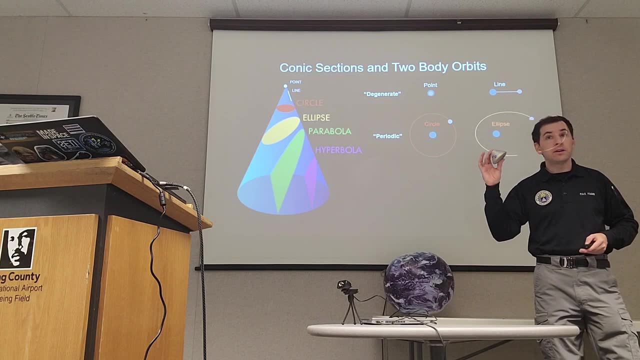 These are going to cover all of the orbits that you're ever going to encounter in a satellite operations context and in most crew spacecraft contexts. Even the Orion orbit that was transiting between the Earth and the Moon was well approximated by an ellipse for the majority of its flight. 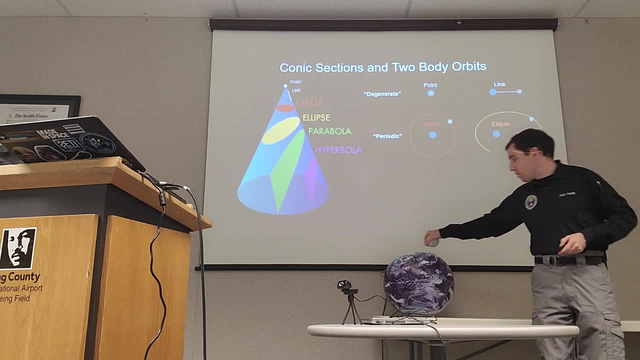 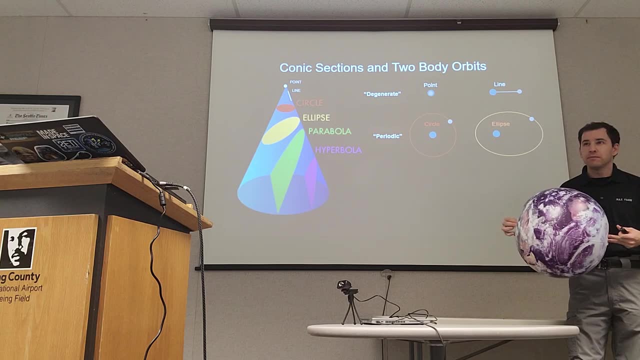 The distances were quite large. If this was the Earth two scale, this is about a 1 to 37 million scale model of the Earth. where about would the Moon be on this scale? I mean terminal building, Terminal building. Any other guesses? 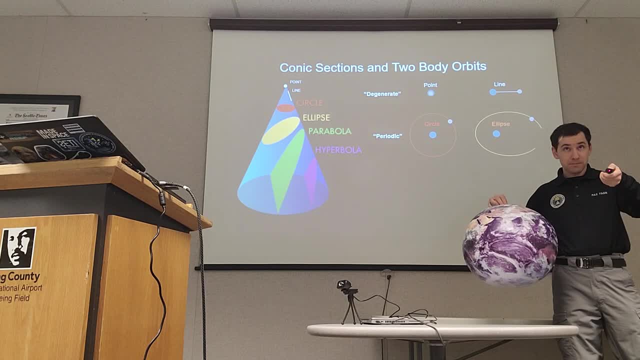 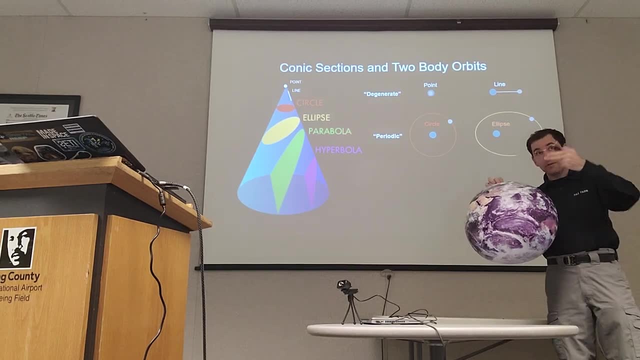 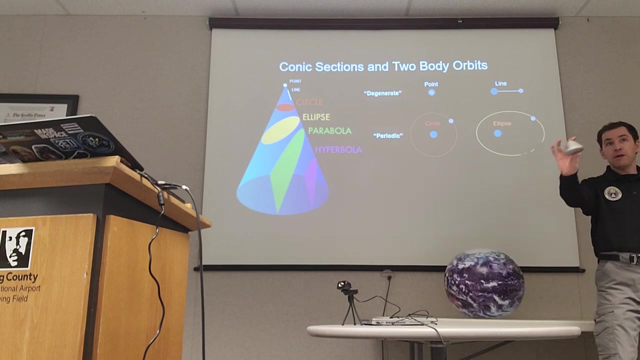 It'd actually be right about there. See Turn around Two scale. That's also about a 1 to 37 million scale model of the Moon. That's about the actual scale between the Earth and the Moon. But still, you can see, that's quite a fair distance compared to the conventional distances of crew spacecraft. 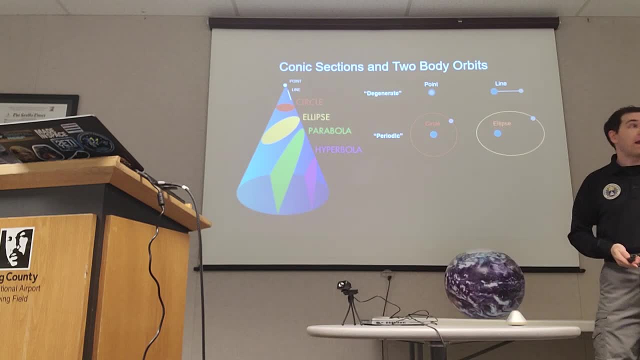 All crew spacecraft operations in low Earth orbit: the Dragon, the International Space Station, the Space Shuttle- none of them ever went more than a finger's distance away from the Earth, Hundreds to a thousand kilometers at most. It's not very far on this scale. 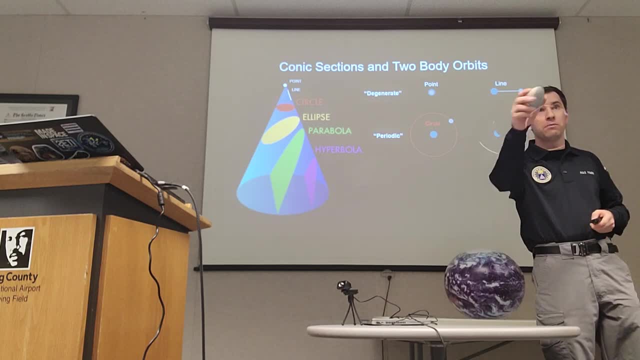 So the Orion really did make quite a fair distance getting to the Moon. But even in that situation, for most of the flight its orbit was well approximated as an ellipse. That approximation breaks down when the gravity of the Moon and the gravity of the Earth are both significant forces. 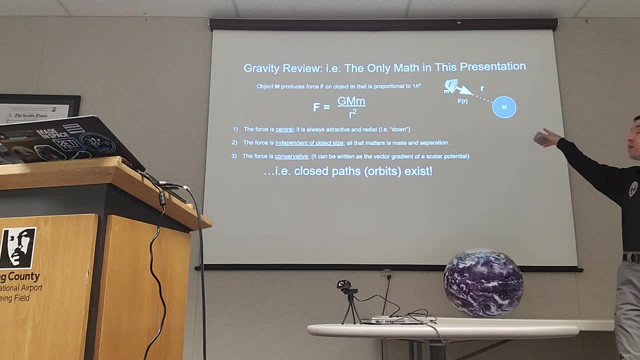 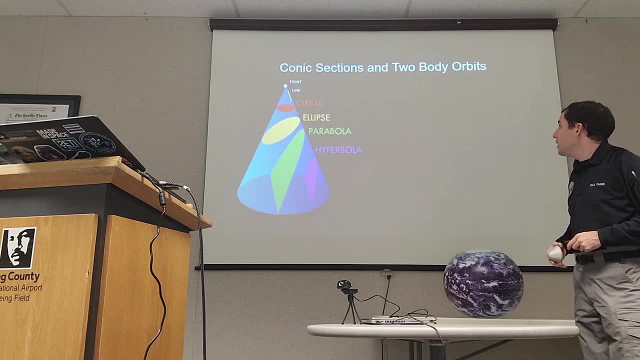 As you can see, this derivation only applies to a single central force. It's not valid when there's two large forces of gravity operating on the vehicle But even on the way out, until it was maybe 50 or 60 thousand kilometers. 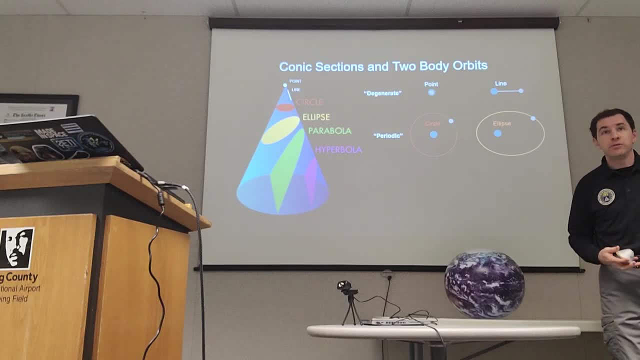 maybe 50 or 60 thousand kilometers away from the Moon. it was still moving on a path that was very well approximated as an ellipse. These two cases- the parabola and the hyperbola- we call open orbits, And really the only times when you're going to encounter these types of orbits. 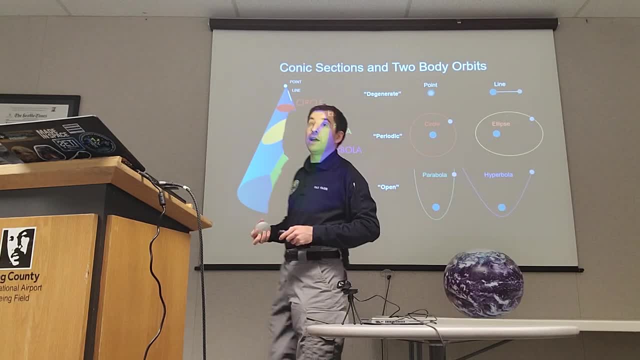 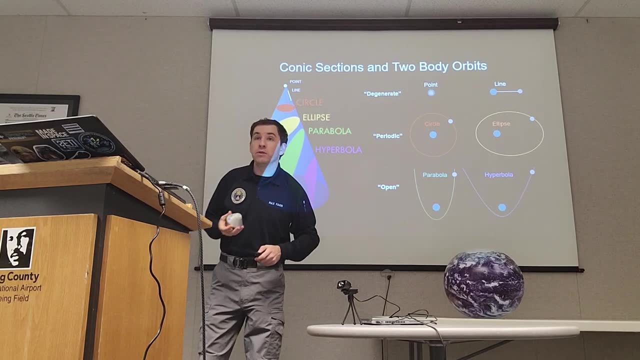 are if you are departing the Earth-Moon system. so if you're flying interplanetary, or if we're not talking about a spacecraft, we're talking about something like a comet, Comet orbits are well approximated by parabolas, The interstellar comet, which we've seen a couple of. 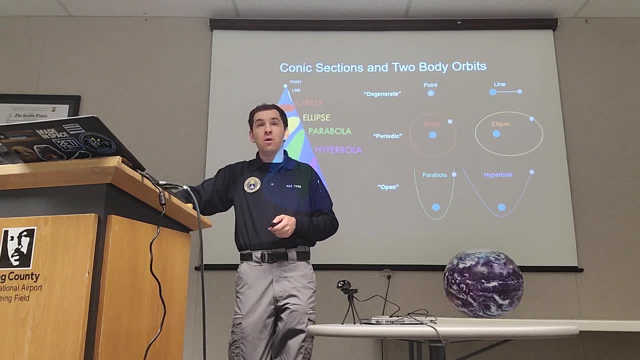 just a couple of years ago, we had a couple of instances of comets, slash, asteroids- we don't really know what to categorize them as- that were passing through our solar system from interstellar space, And those paths are well approximated by hyperbolas. 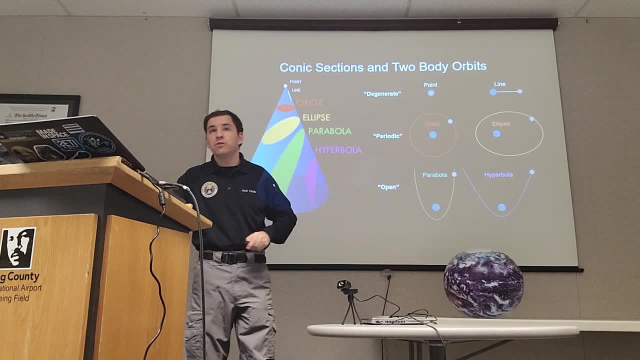 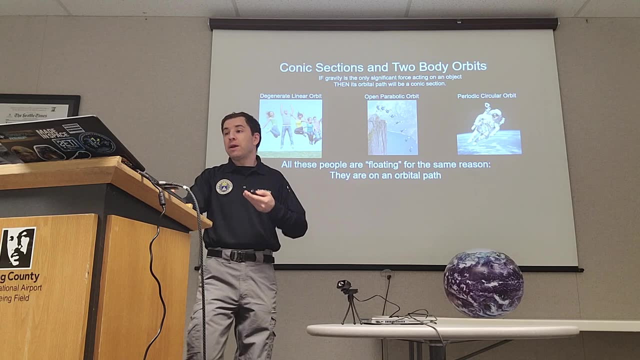 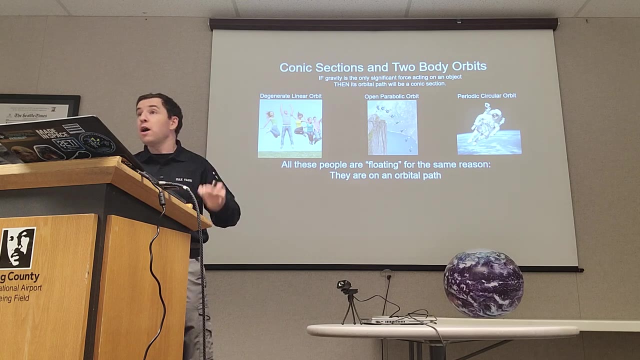 But this doesn't generally apply to crew spacecraft, unless you're visiting interplanetary space. So all five of those orbit categories, they all operate under the same laws of physics. They're all described by the same equations of motion. That's true of us too, here on the surface of the Earth. 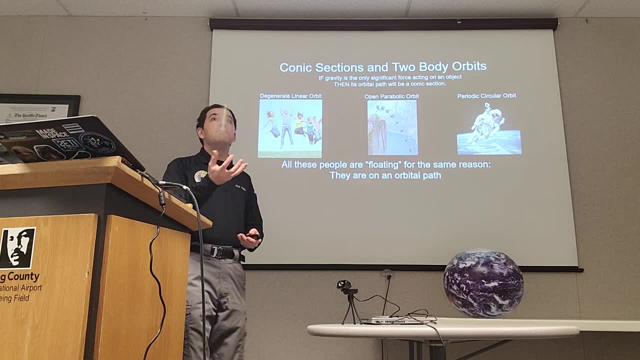 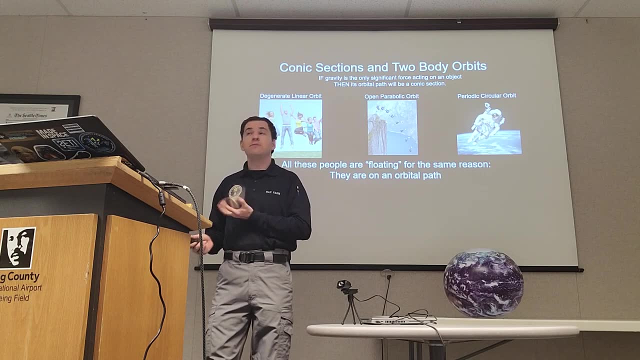 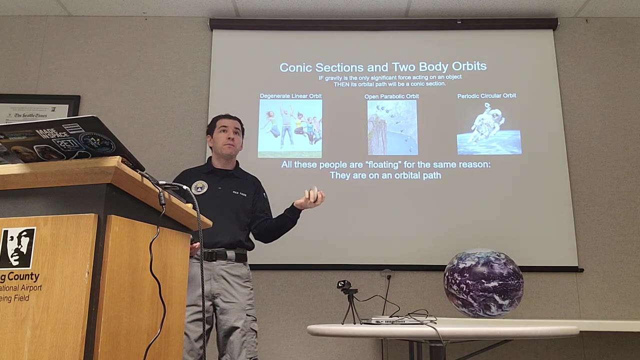 This object. if you do that, it's moving on a ballistic trajectory, It's suborbital. it's going to intersect the ground relatively soon, so it wouldn't be convenient to describe this as an orbit, But technically speaking you could model this as a parabolic orbit. 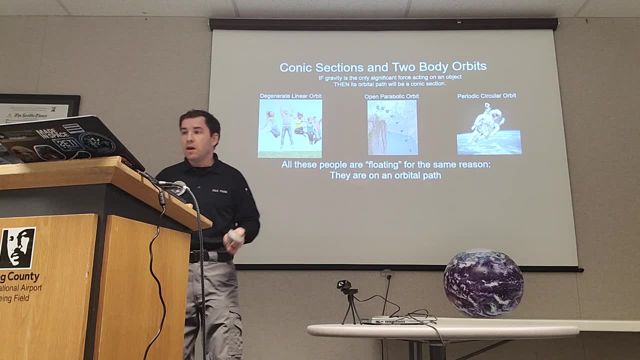 centered with one foci. It's the same. for a human being that's jumping, it's the same as if you were base jumping off a cliff. All three of these objects are in orbit, it's just two of them are suborbital. 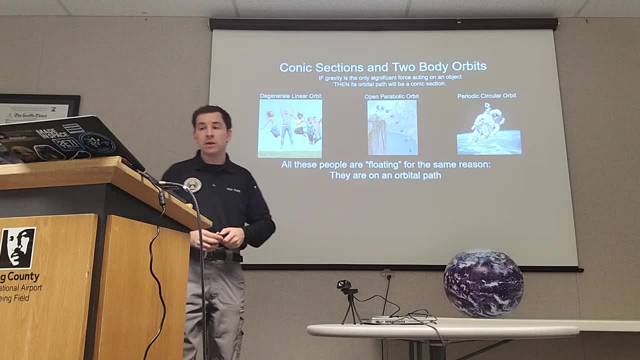 They're going to strike the Earth relatively soon, so we don't usually talk about that as being in orbit. But, as I'm sure you are all aware, if you're in an aircraft and you dive down, you go into freefall for a period of time. 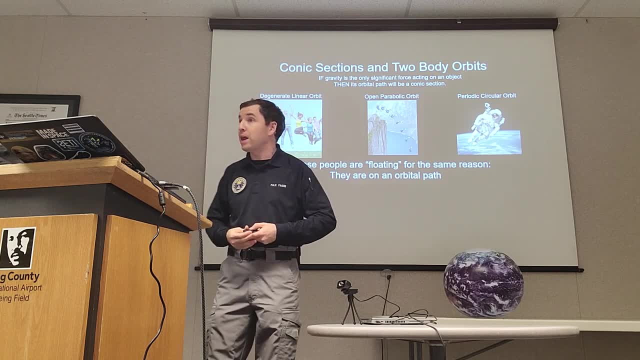 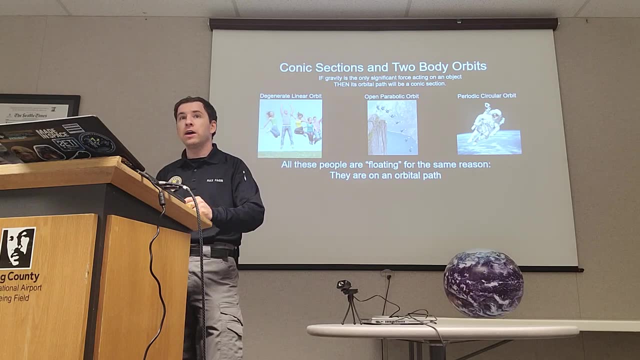 you are going to feel the exact same zero gravity as an astronaut on orbit, and for exactly the same reason. Freefall is weightlessness, in exactly the same way that astronauts in the ISS are. It's all the exact same reason. It's just much easier to sustain weightlessness. when you're going around the Earth than when you're in an airplane diving for the Earth at 300 knots. But it's exactly the same phenomena of weightlessness. That's why astronauts are weightless. it's because they are in freefall. 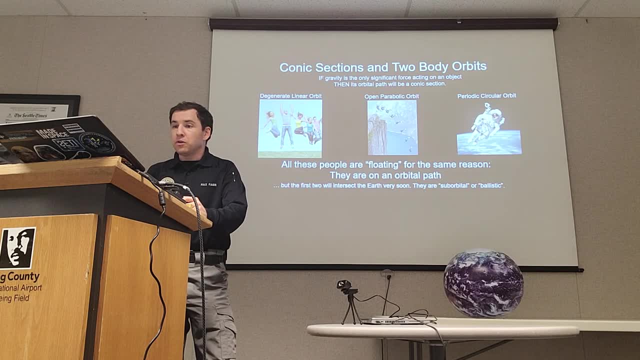 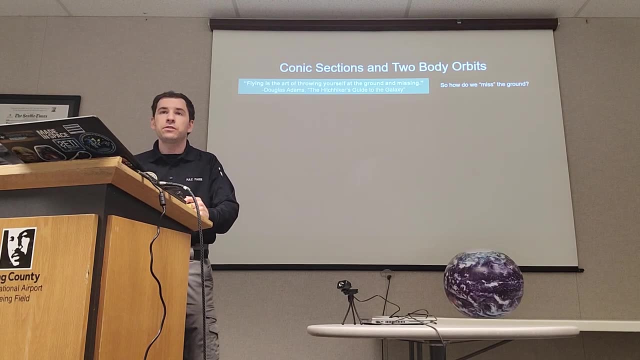 The exact same reason as when we're diving an aircraft. So the intention of, So the intention of all this is really just to get across the point that it's the same laws of physics that govern objects in free flight here on the ground as it is the objects in space. 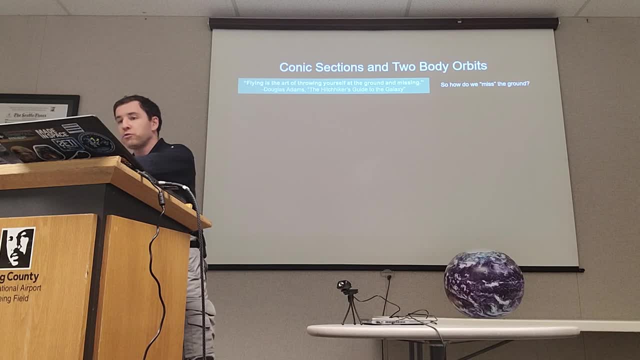 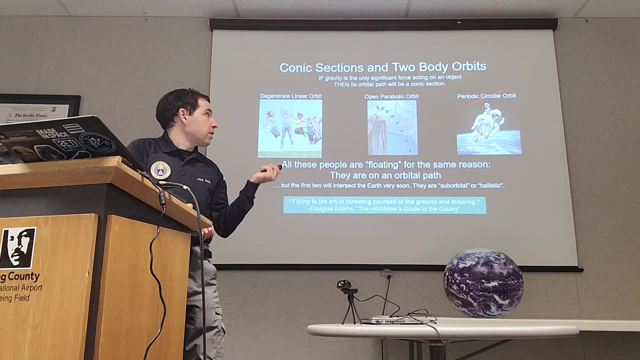 It's just objects on the ground. you can't usually ignore air dragon objects. in space you can. It's also important to remember that space itself, this astronaut, this astronaut right here, is not terribly far away. Space itself is closer to us. 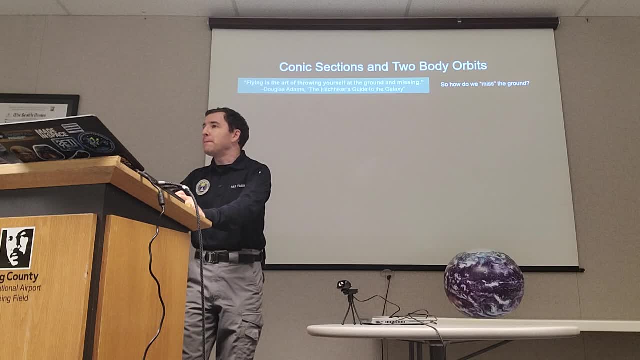 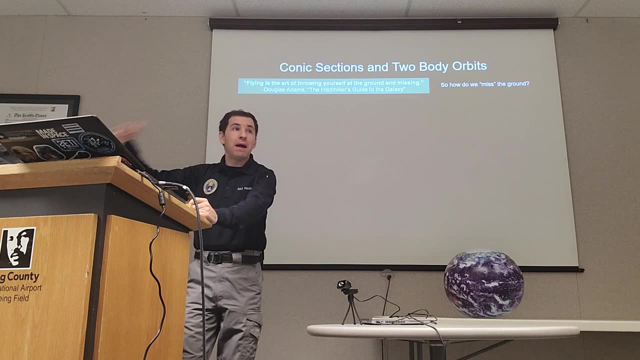 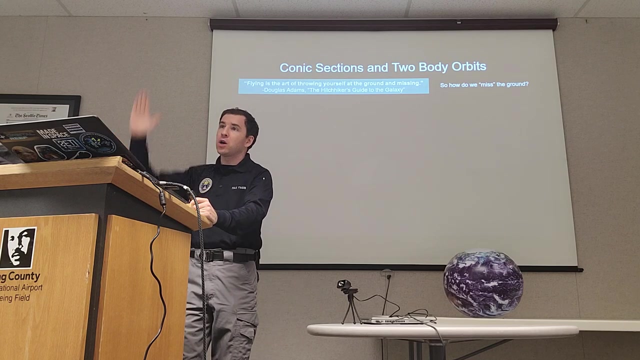 than South Dakota. We're closer to space right now than we are to Canada. Space is not very far away. The official boundary space is only 100 kilometers up. There are particularly powerful rocket-powered aircraft that can go on a ballistic hop to that altitude. 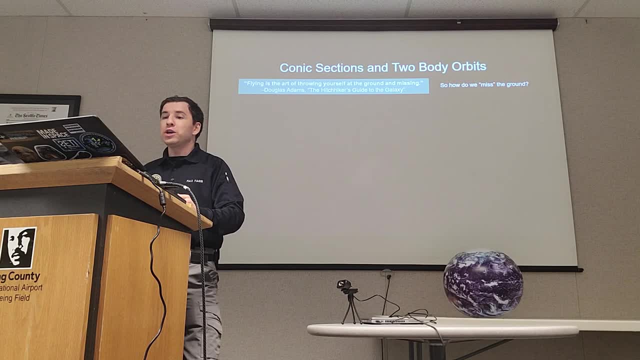 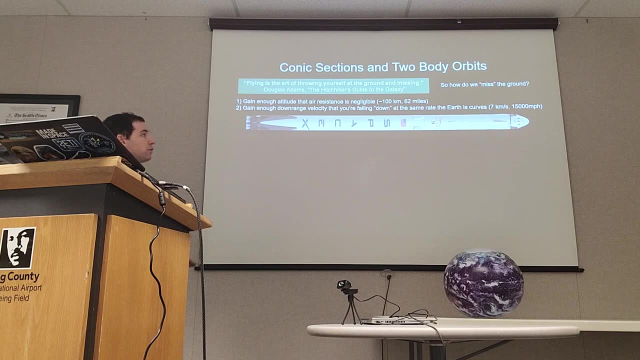 It's not terribly far away. The majority of propellant that is in a launch vehicle like you can take a look at the SpaceX Falcon 9 right here. the majority of propellant that is in a launch vehicle like this is not about getting high and getting to space. 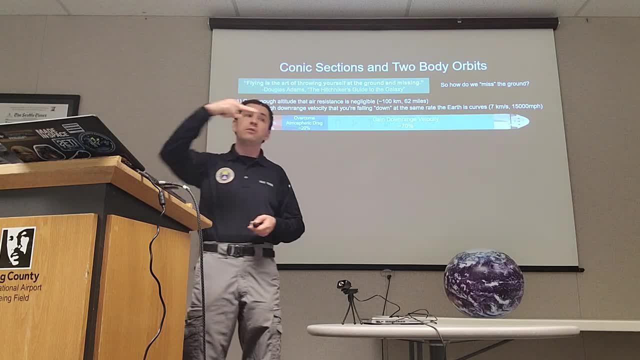 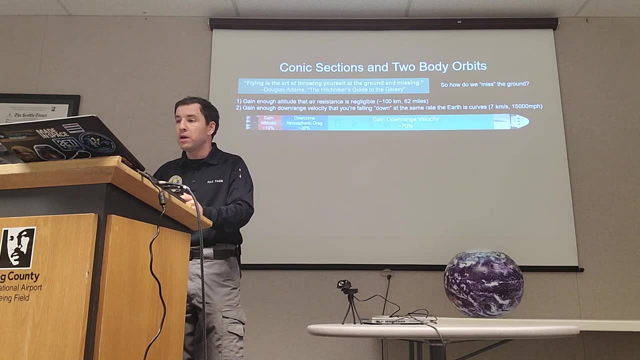 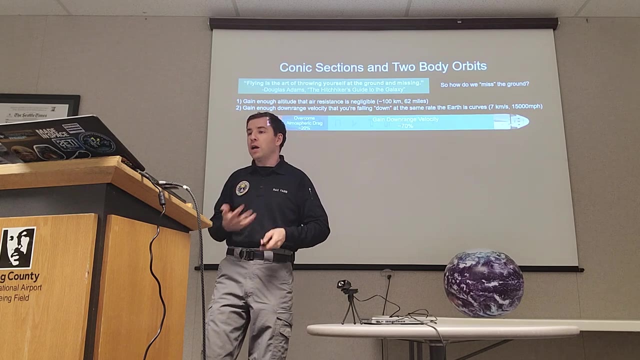 It's about going fast enough to achieve the critical velocity where you can enter free fall around the Earth, where you're going to miss the Earth as the Earth curves away from you. If we make some simplifying assumptions about this, then the optimal way to accomplish this 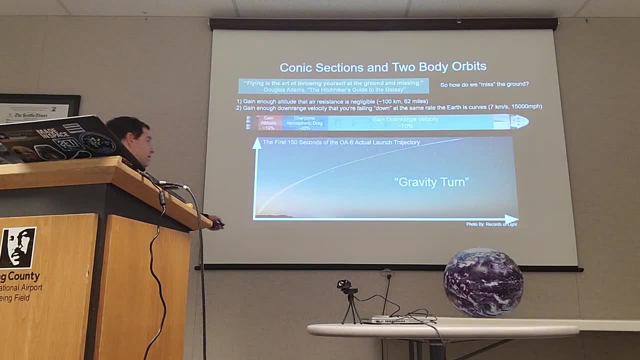 is what we call a gravity turn. This is a time-lapse photo taken of a launch trajectory out of Cape, and you can see the vehicle starts its ascent nearly vertical, but then very rapidly tips over into the horizontal. The reason for that is because, again, it does not need to get very high. It needs to go fast. seven kilometers per second, about 15,000 miles per hour, in order to achieve an orbital state. Minor note to make us kind of proud of our humanity from this: 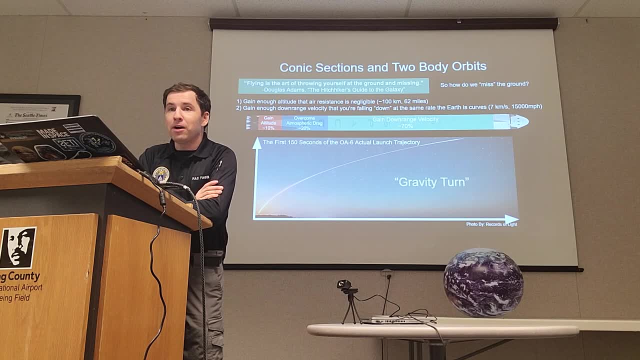 There are a lot of places in the solar system where intelligent life could have evolved, but because of Earth's atmosphere and mass, we humans, we have evolved in pretty much the hardest place in the solar system to launch a space program from where life could have evolved. It's conceivable that we could have life evolving on a much hotter place, like, say, Jupiter or the Sun, but if we assume that intelligent life like us has to evolve on a rocky planet with a relatively cool surface and little water, we evolved in the hardest spot in the solar system. 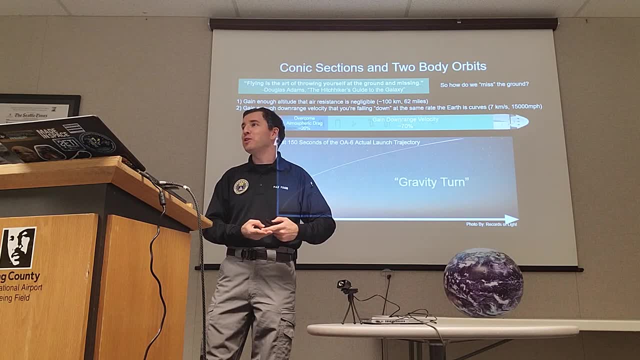 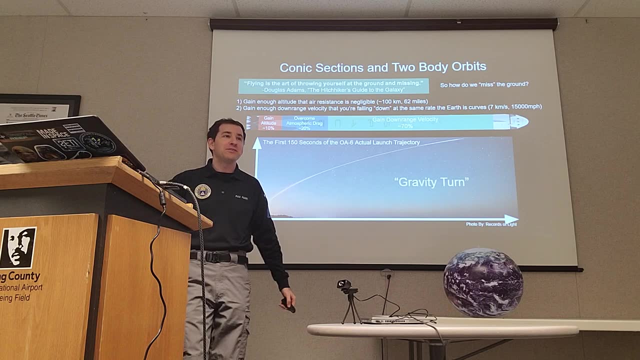 to launch a space program from. So whenever you see a rocket launch successfully to orbit, you can take some serious pride in your humanity for that. we are doing this. we are doing this from the hardest place in the solar system where it could happen. 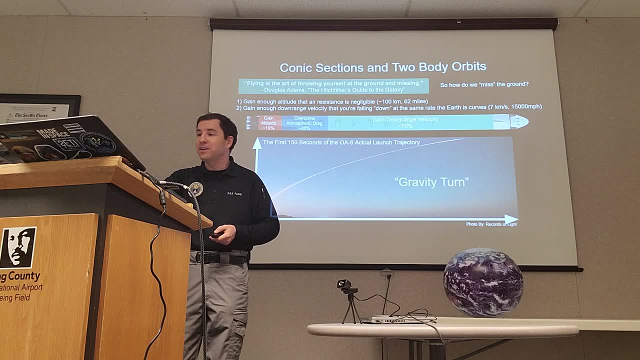 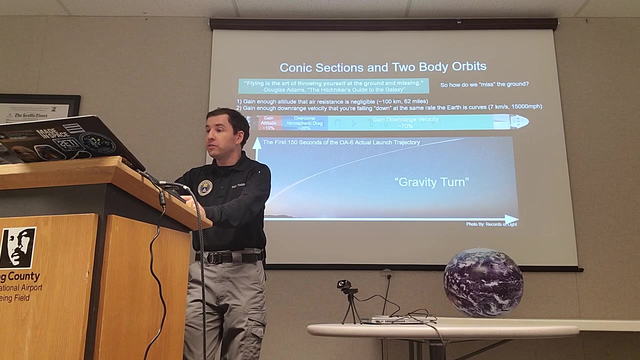 If we ever encounter intelligent space-faring aliens, we will probably have a significant boasting point on this fact, because we have evolved from a. you think your space program was hard to get out of the ground? wait until you see our planet. Yeah, if we had evolved on a place like Mars or Titan or Enceladus. getting to orbit would be five to ten times easier or cheaper. You know we could have gone to the moon with the size of the rockets that we usually fly than we first took humans up into space on in the Mercury and Gemini days. So yeah, be proud of your humanity for that. 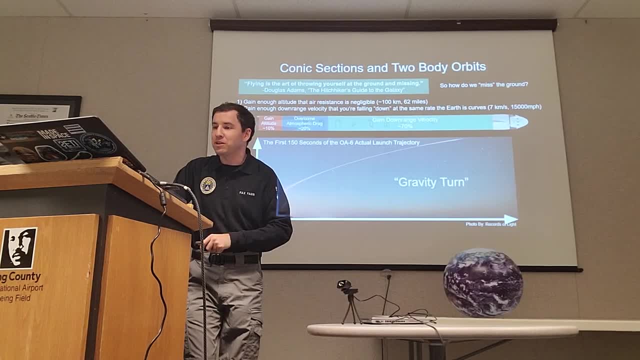 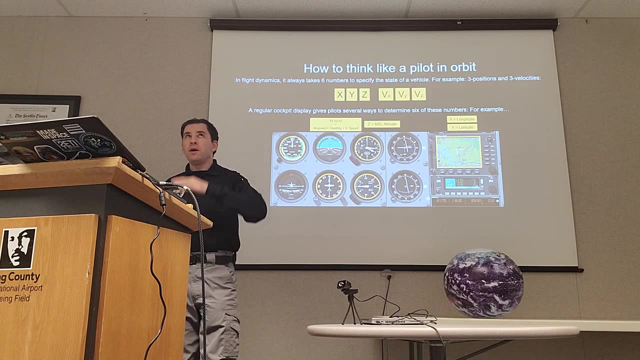 because the universe has stacked the deck against us pretty difficultly, Alright. so how does our pilot intuition kind of wrap to this? So we don't usually teach aviation skills in terms of coordinates, but it's important to remember that all of these instruments 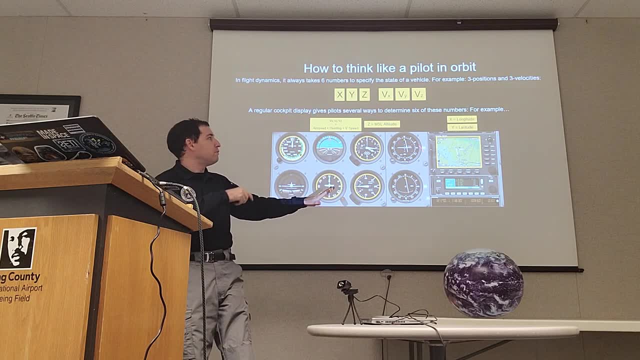 on a mathematical basis. all of these instruments are about conveying to us really six numbers. We need to know our position, which is a three-coordinate information, and we need to know our velocity, which is a three-state vector. We don't think about it that way, because we're not computers. 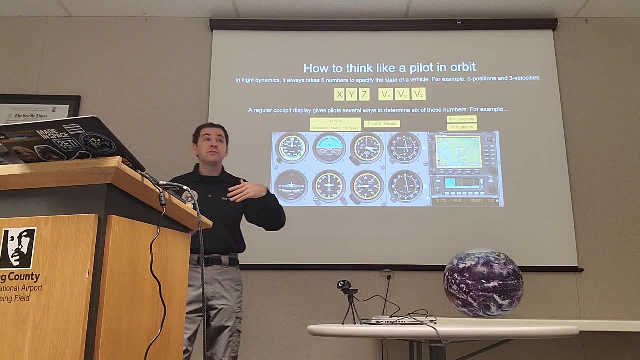 We find it much more easy to think about our state vector, as we would say, the combination of these three numbers. We find much more convenient ways to talk about it. You know, we think about, we don't care about, our distance from the center of the Earth. 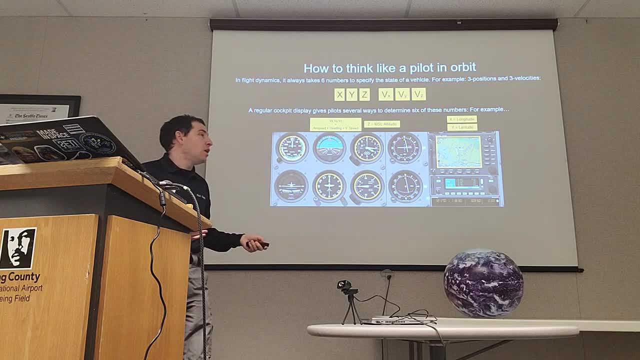 we care about our MSL altitude. We don't care about our latitude and longitude. We care about how far away are we from the airport, how far east and how far north, But fundamentally, what really matters as a pilot is we have to have an understanding of six numbers. 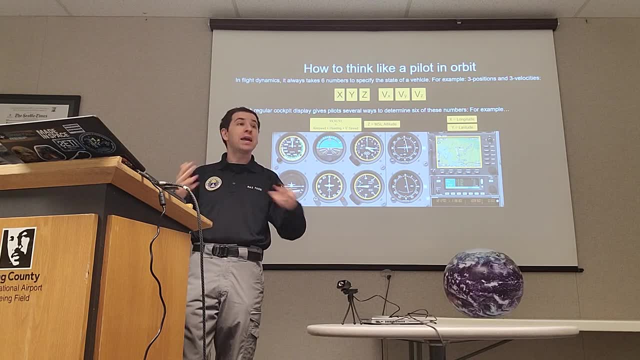 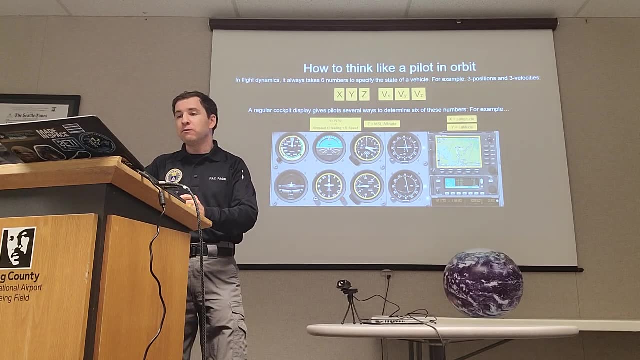 that uniquely define our state vector of the aircraft, And we're free to pick which of those six numbers are most convenient for us at any one moment. But it really is about getting those six numbers which define our state vector, And the same thing applies to spacecraft. 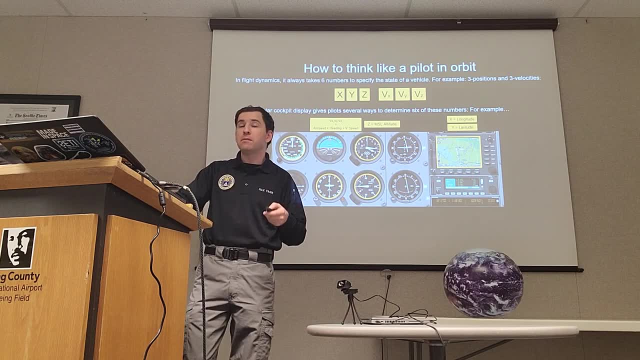 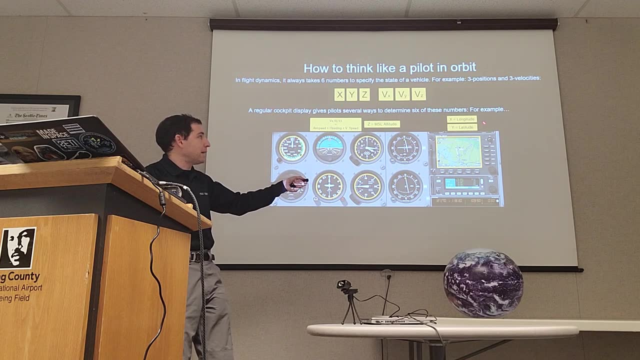 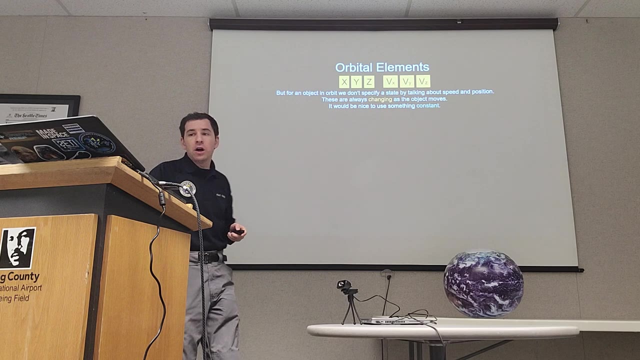 Spacecraft require an understanding of six numbers to define the state vector, But we don't use the same six numbers that we're used to using as pilots, because these numbers turn out to not be very useful. The way we usually do it is by talking about what we call orbital elements. 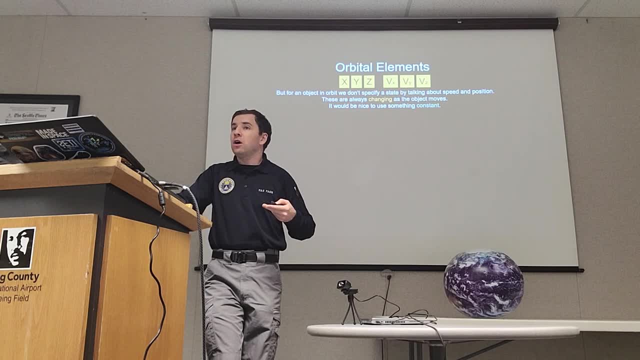 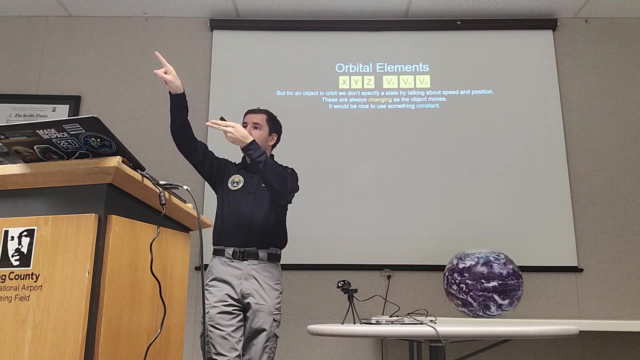 So, if you think about the aviation analog of altitude, latitude, longitude, vertical speed, heading and airspeed, those might be six numbers that we care about in order to specify our state. The six elements, the six numbers that we care about, 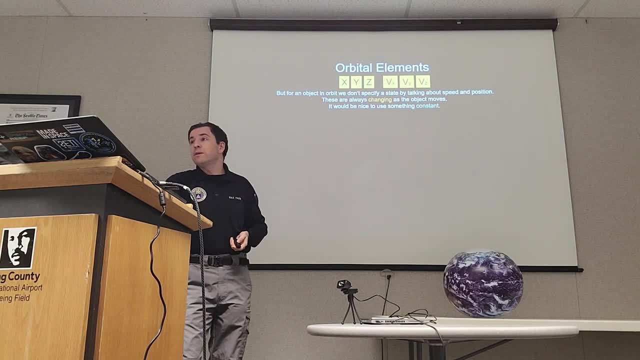 as astrodynamicists, those six numbers would not be useful. The first reason being is because all six of those numbers would be constantly changing. If we talk about our altitude as one of our six numbers- and we're in an elliptical orbit- our altitude is going to be constantly changing. 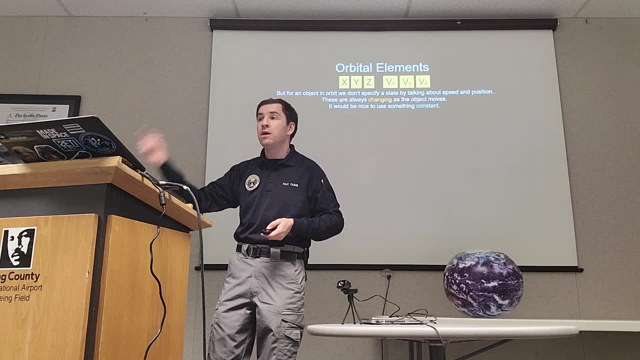 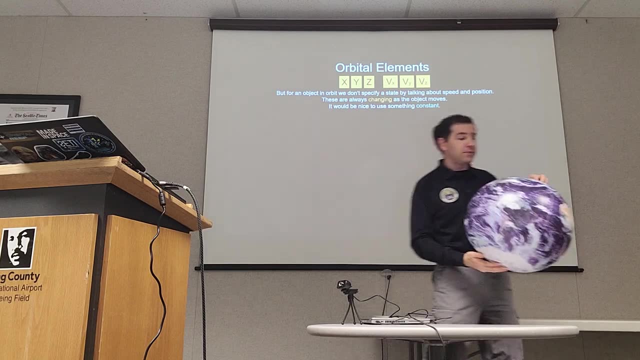 There's no analog to straight and level flight when you're in an elliptical orbit. If we talk about our heading, it makes sense to talk about heading for seconds to minutes in an aircraft. but if you ever fly transoceanic, you know if you start here in New York. 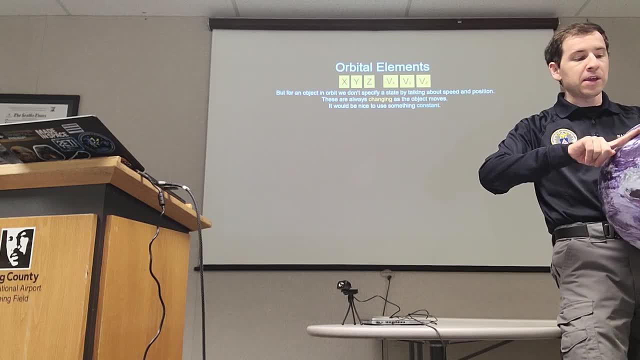 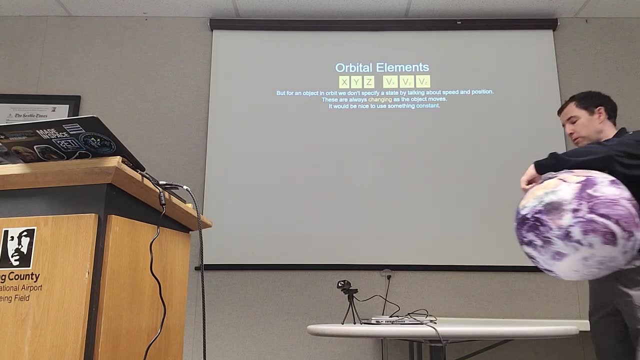 and you set a heading vector to due northeast and then you just keep flying due northeast. you're going to take a curved path If you wanted to fly from one point on Earth to the other. you can't fly a constant heading or a constant bearing. 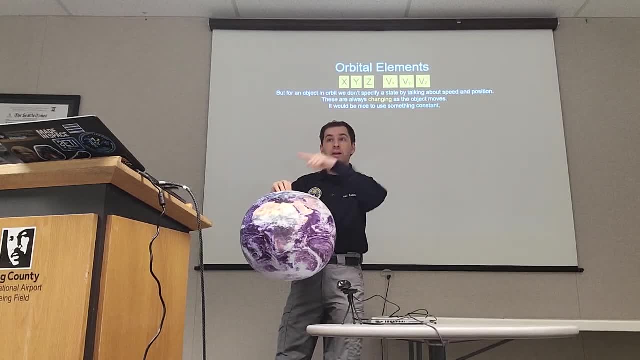 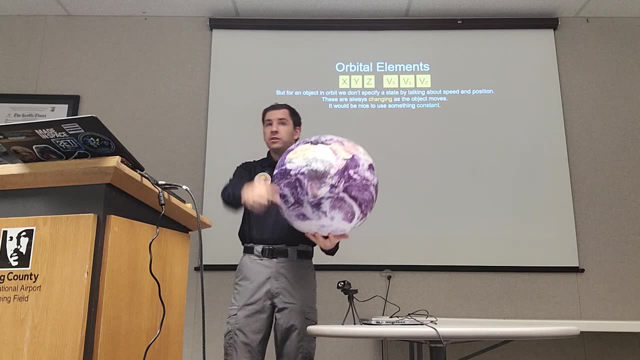 You're going to miss your target. Well, imagine if you're going around the Earth once every 90 minutes. The angle is going to be constantly changing. It's the same problem, with your latitude and longitude constantly changing and in ways that are very unintuitive to understand. 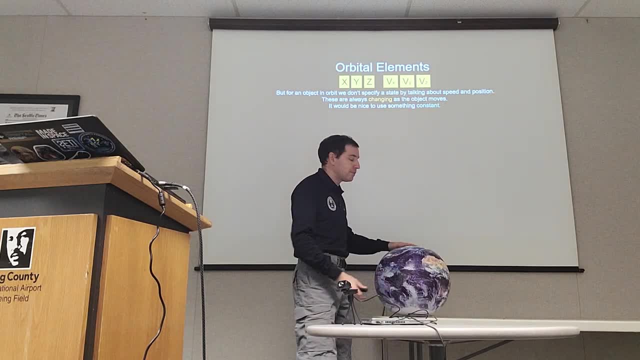 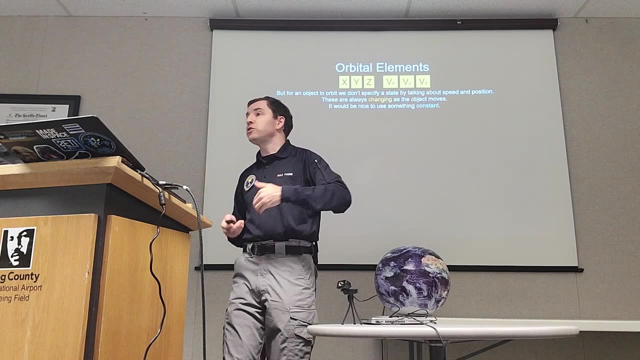 So, as astrodynamicists, it would be really nice if we could pick six numbers where the majority of those numbers were constant, where they would only change if we intentionally changed something about the way our spacecraft was flying, And through a process of trial and error. 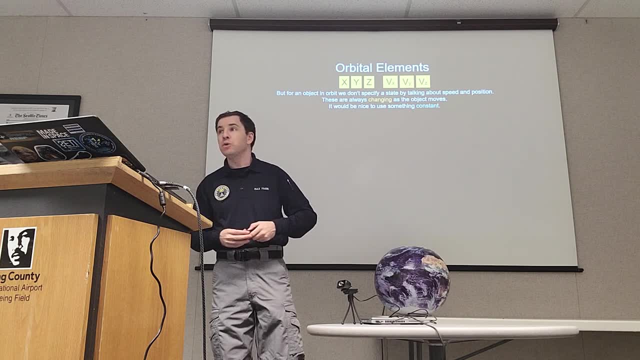 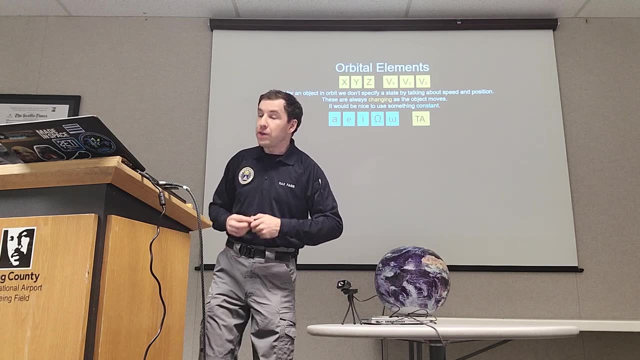 over a century or so, we have kind of come down to a combination of six numbers that are very convenient to work with, which we call the classical Keplerian orbit elements, And these six numbers are what we talk about, in the same way that pilots talk about. 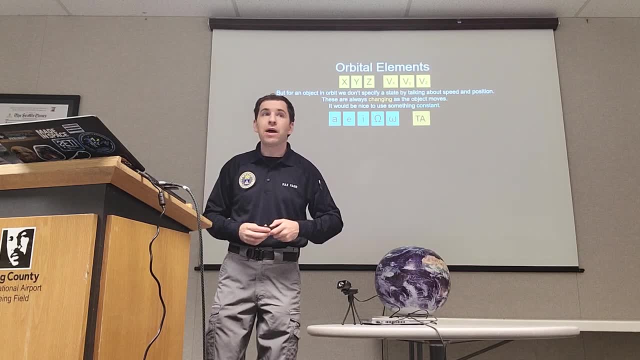 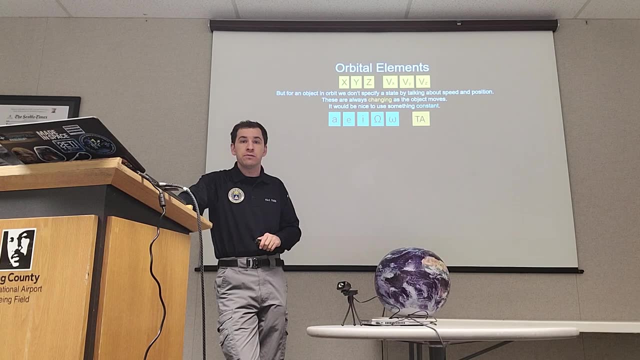 airspeed, altitude and heading. You will hear astrodynamicists talk about these numbers. Let's talk a little bit about what these six numbers are, because they're important for getting a good intuition about how a spacecraft is flying. So the first two numbers here: A and E. 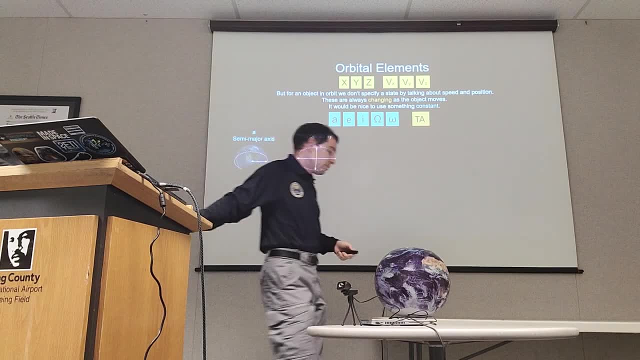 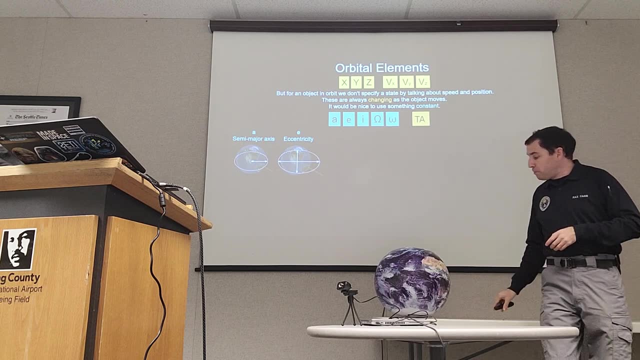 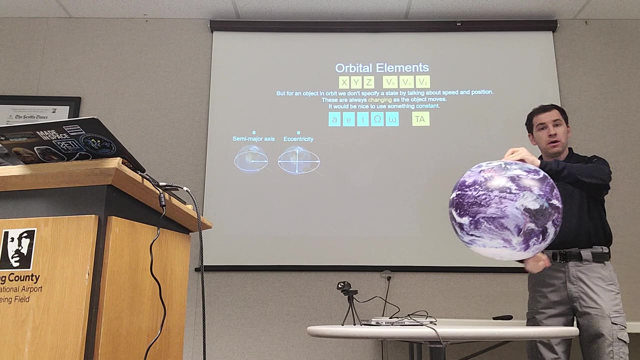 are what we call the semi-major axis and the eccentricity. The semi-major axis you can think of as the equivalent of your altitude. The semi-major axis tells you how big is the orbit around the planet. A low-altitude circular orbit has a very small semi-major axis. 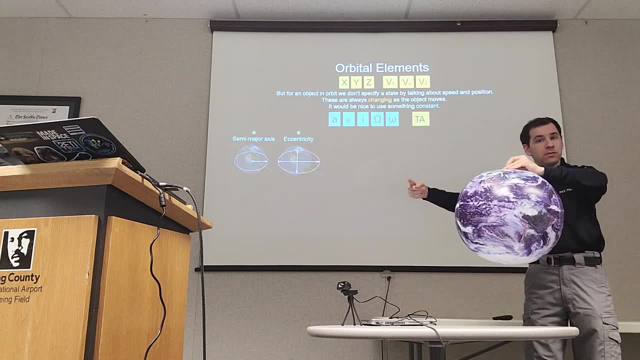 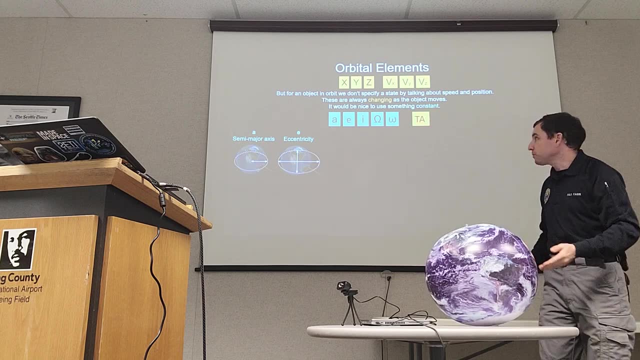 A large orbit has a large semi-major axis, And what it is is. it's just half the distance from the center of the Earth to your orbit. if you're in a circular orbit, That's the semi-major axis. The eccentricity describes. 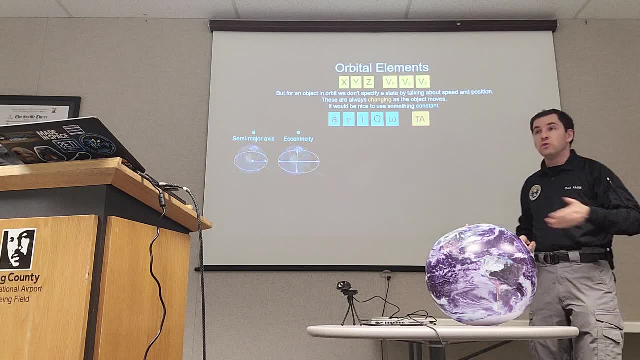 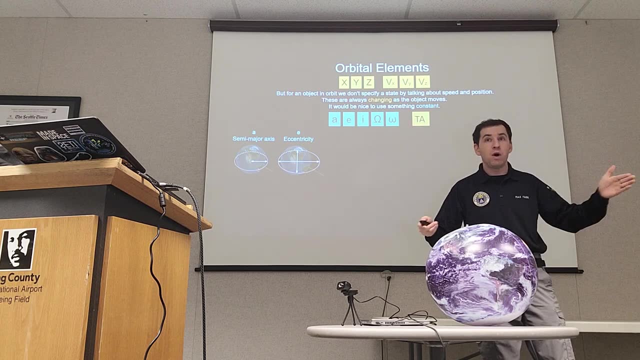 how oblate is the orbit, how elliptical is the orbit. So an orbit with zero eccentricity is just a circle. An orbit with an eccentricity of one is a parabola. Anything between one and zero is an ellipse, with one being the more elliptical side. 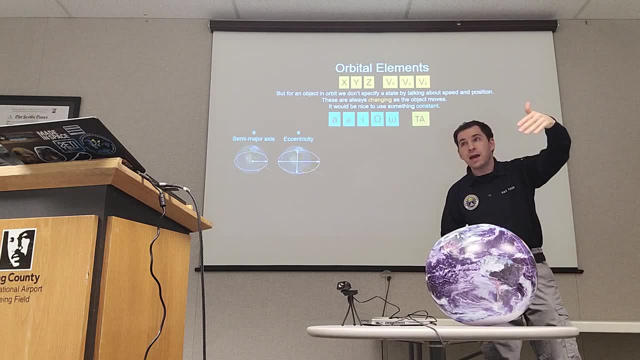 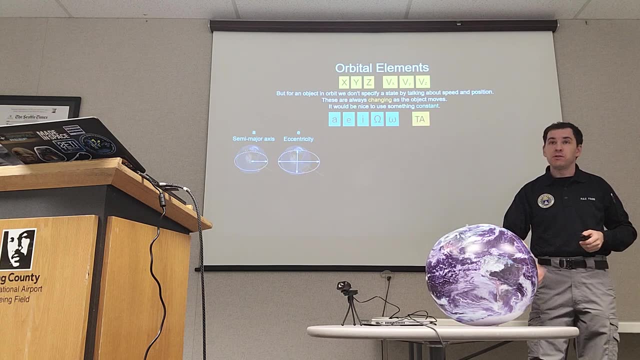 Translunar orbits that go between Earth and the Moon tend to have eccentricities on the order of 0.9, 0.95 or so, whereas the low-Earth orbits that are nearly circular will have eccentricities of 0.0001 or so. 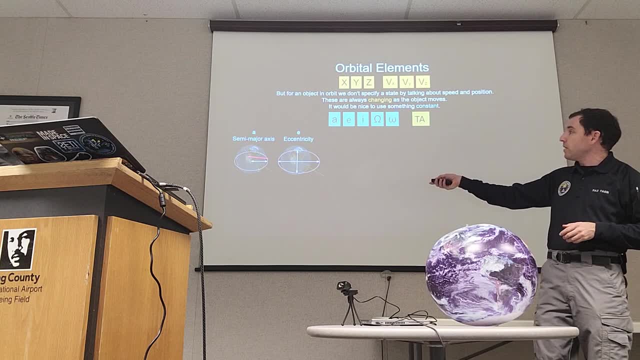 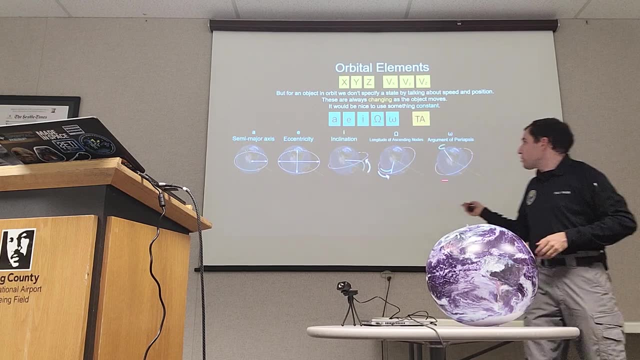 So these two orbits describe the size and the shape of the orbit. Semi-major axis: How big is the orbit? Eccentricity, How elliptical is the orbit? These three numbers, the inclination, the longitude of ascending nodes and the argument of periapsis. 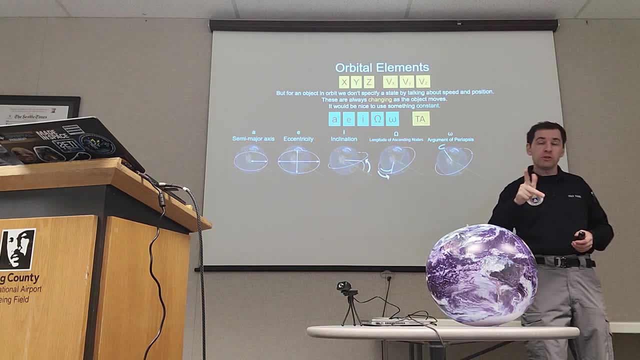 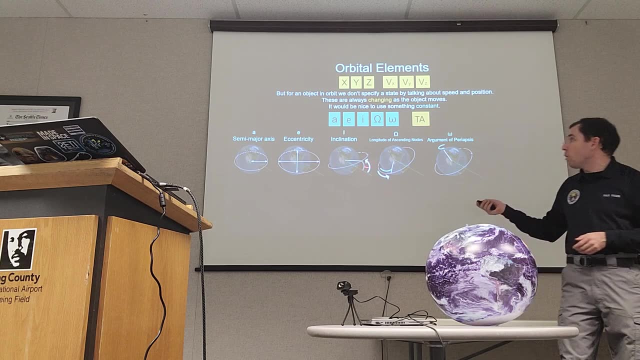 are the Euler angles. They're the analog to pitch, roll and yaw, But they're not describing the attitude of the vehicle. They're describing the attitude of the orbit. So inclination describes how tilted is the orbit from the plane of the equator. 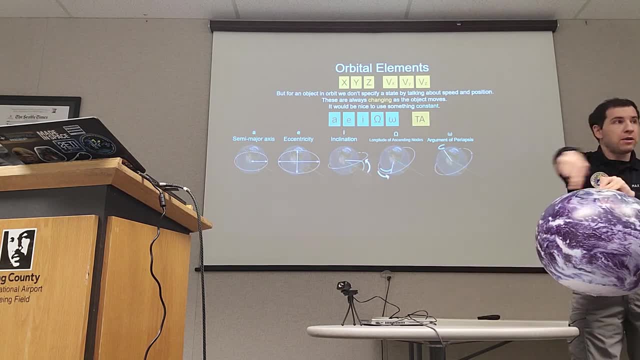 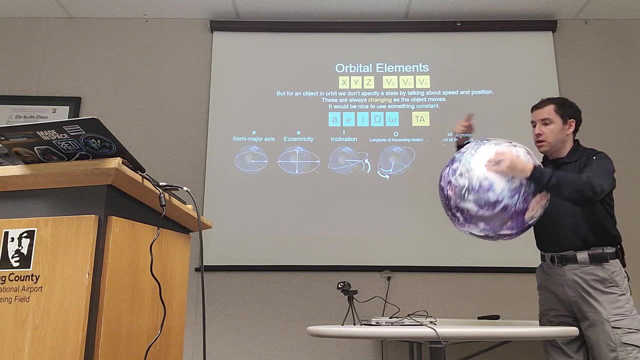 An object that is orbiting the Earth in the plane of the equator, so like this: if my left hand is on the north pole, this has an inclination of 0 degrees. If it's going around the Earth like this, that's an inclination of 90 degrees. 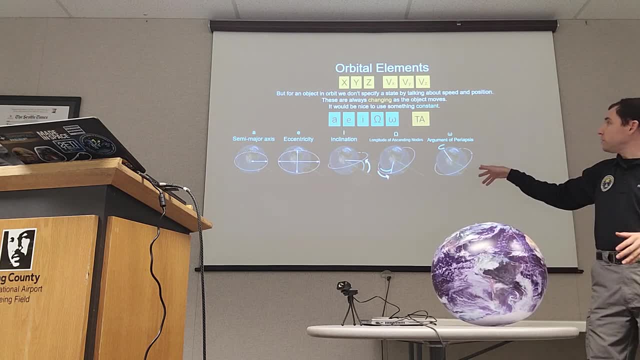 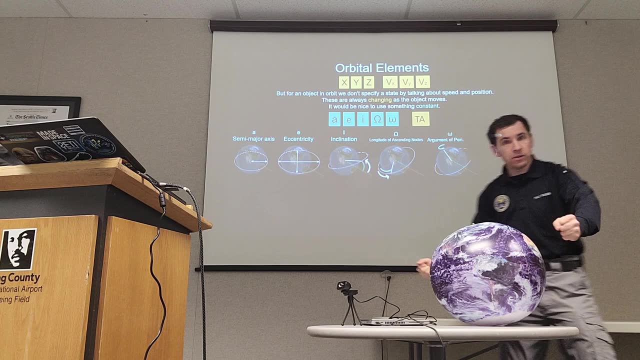 So that's one of the Euler angles. The other two Euler angles, the longitude of ascending nodes and the argument of periapsis tells you how is the orbit rotated in the other two directions. So those combination of three orbits gives you a specification of the orientation. 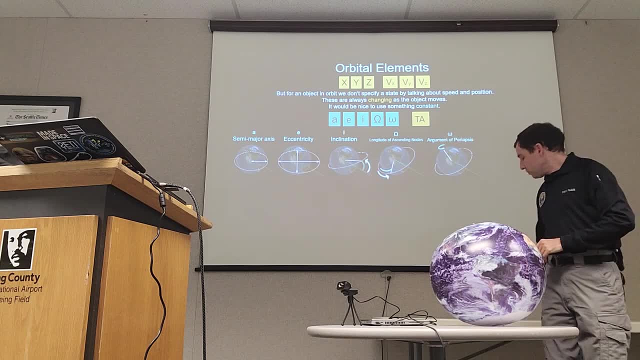 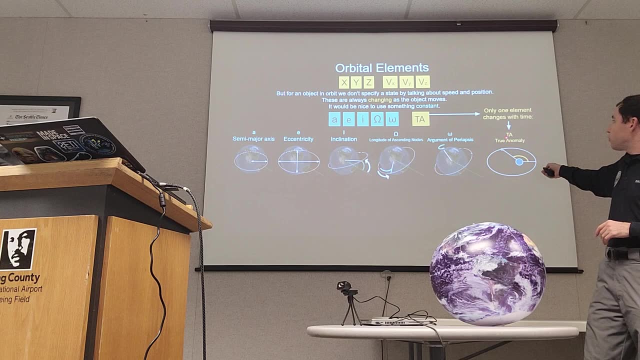 of your orbital plane in inertial space. So two elements for the size and shape, three elements for the orientation of the orbit And then the final one. what we call the true anomaly, is the only element that changes with time. for the most part, 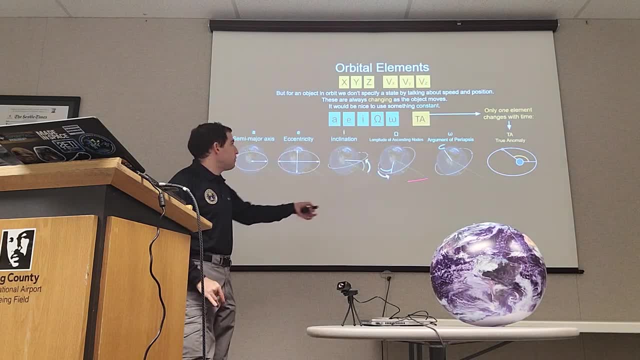 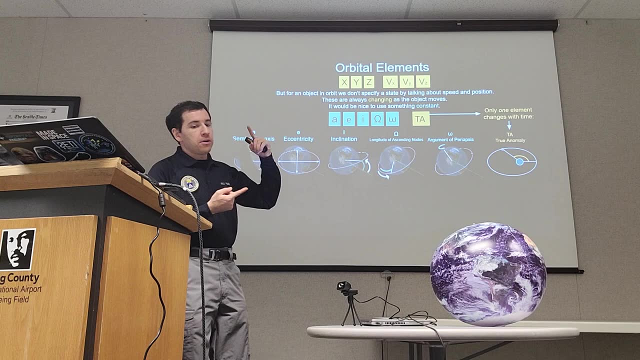 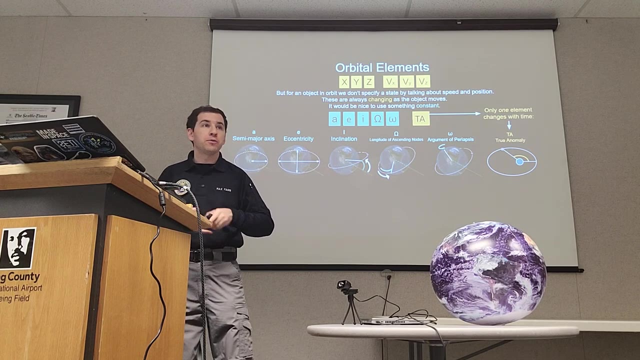 So the first five elements right here. because of the way we picked them, these can be made analogous to what is your air speed, your vertical speed, your heading and your altitude. If you're in straight and level flight, They're constant. 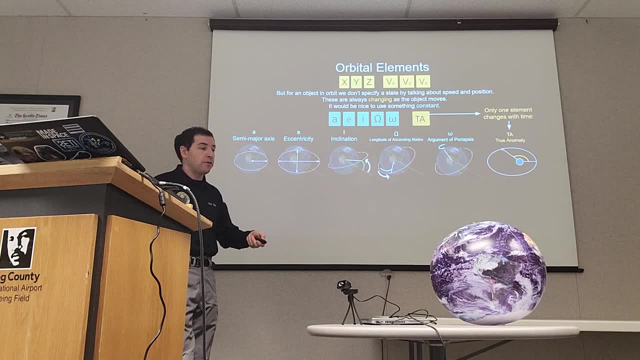 Those four numbers are constant And for an object in orbit around the Earth, not thrusting, not subjected to any perturbing forces, these first five elements are constant And it's only this one that all the change has been backed into. 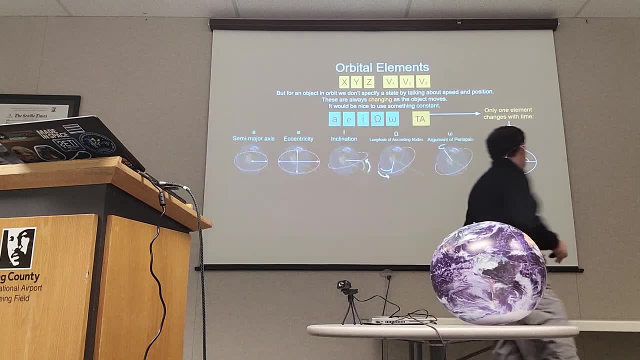 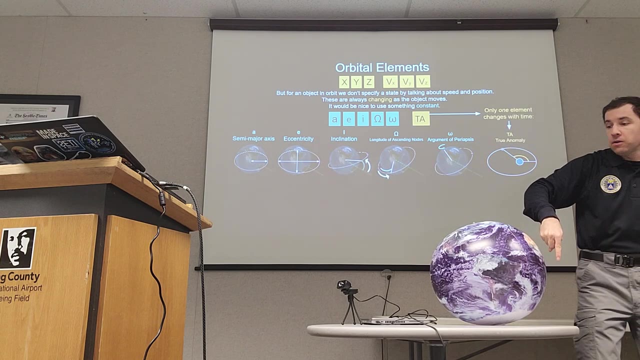 So true anomaly refers to the angle between the spacecraft's current location and the most recent perigee, perigee being the point of closest approach, So that's constantly changing. An object in a in an elliptical orbit like this will have a true anomaly of zero degrees here. 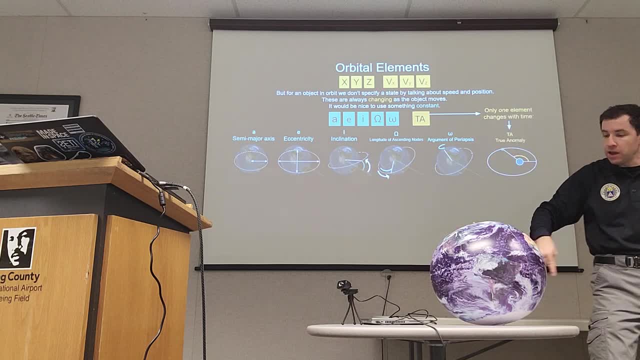 90 degrees, 180 degrees, 270, and zero. So an object in an elliptical orbit like this, its true anomaly will be constantly changing, but all other five elements will remain constant, Unlike if we were to use the five numbers. 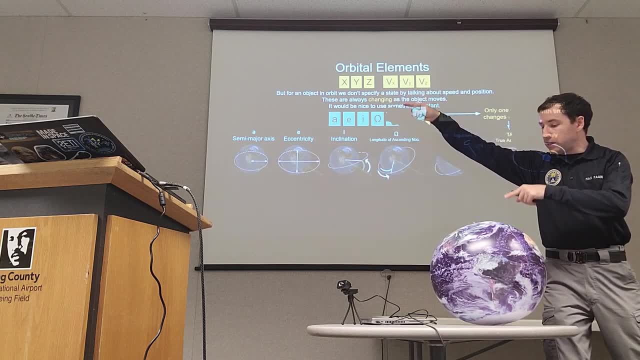 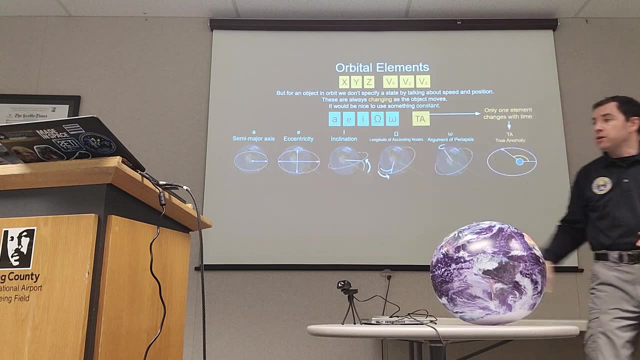 like latitude and longitude. Latitude and longitude, high latitude, low latitude. they would be constantly changing. It would be very difficult to talk about the state space of the spacecraft if we use those numbers, But with this combination of these six classic Keplerian elements, 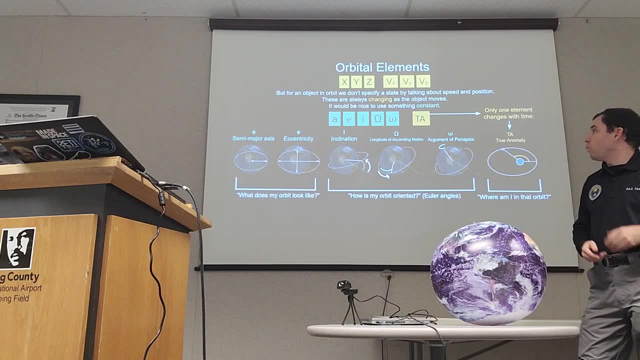 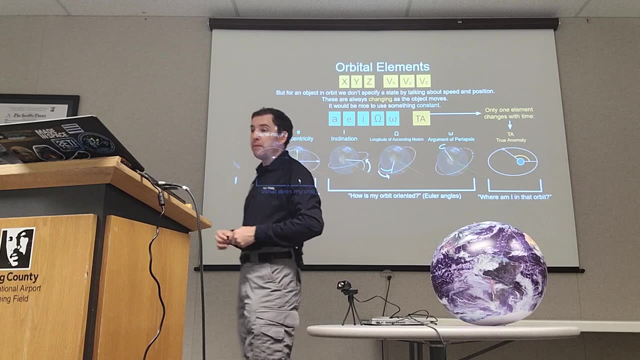 it becomes a lot easier to talk about what our spacecraft is doing at any one point. So, yeah, so these are the classical Keplerian elements and it's important to have a good sense for them, in the same way as a pilot does with we do for altitude. 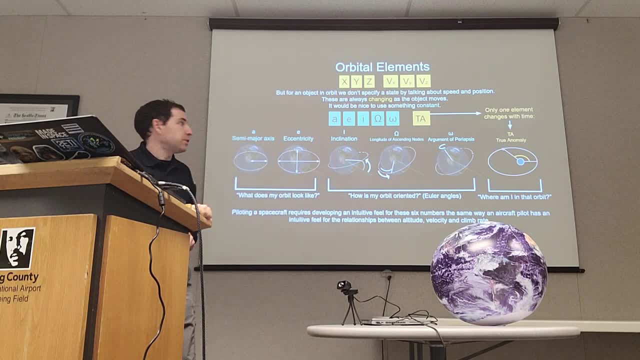 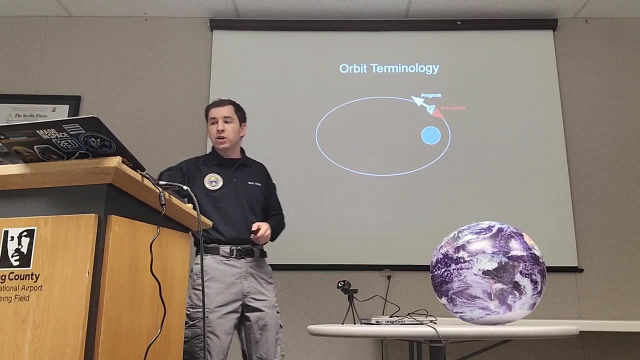 airspeed heading, all of the conventional things that we're used to getting out of our instrument. now A little bit of terminology. So we refer to the direction of motion as prograde and retrograde. So if a spacecraft is going about the planet, 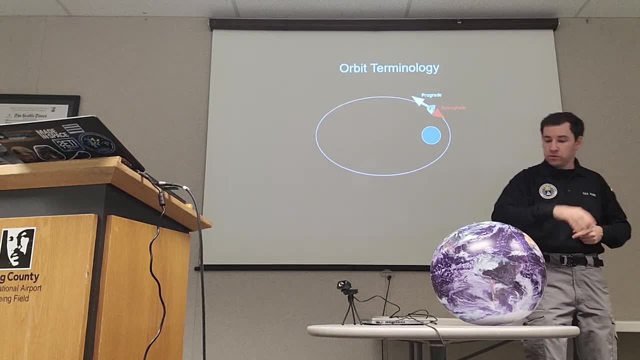 in the same direction as the planet is rotating, so west to east. in this case we say it's a prograde orbit. If it's going around west to east or east to west, that's a retrograde orbit. We define the point of closest approach. 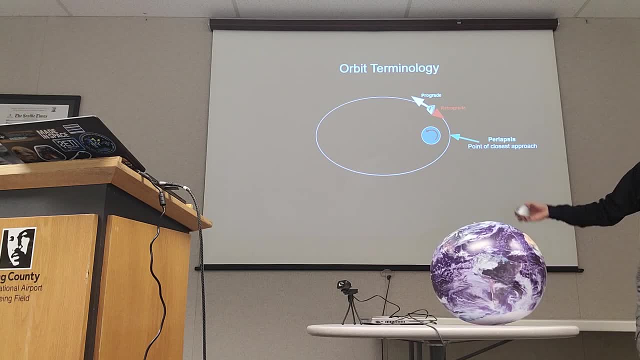 as the periapsis, or sometimes we will change the last term, the last few letters of this to refer to the specific body. So periapsis and apoapsis, the closest and the furthest point, and we will refer to. 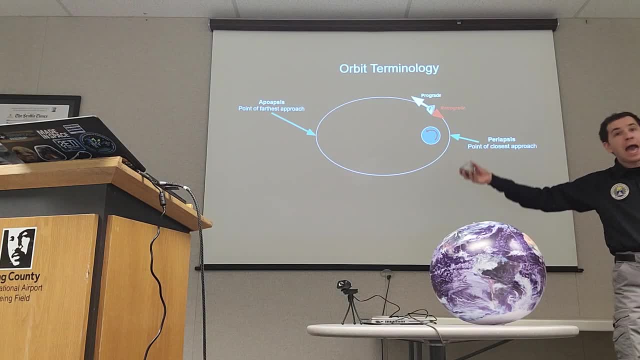 if we're orbiting the Earth, for example, we'll sometimes call this the peri-g and the apo-g, g meaning Earth. The eccentricity refers to how eccentric the orbit is and the terminology depending on the central planet. So perihelion and epihelion for the Sun. 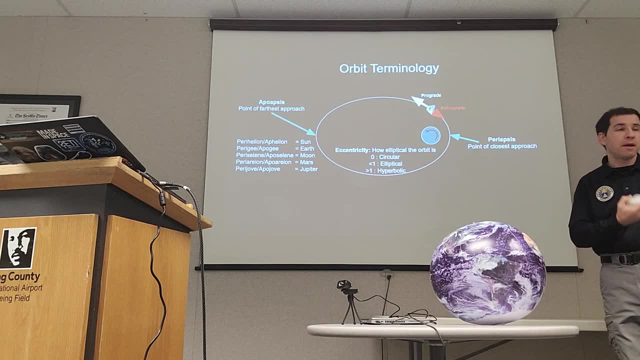 peri-g and apo-g for the Earth, apo-selene and peri-selene for the Moon, selene being the lunar goddess. apo-aerion- peri-aerion for Mars, apogeo- perigeo for Jupiter. 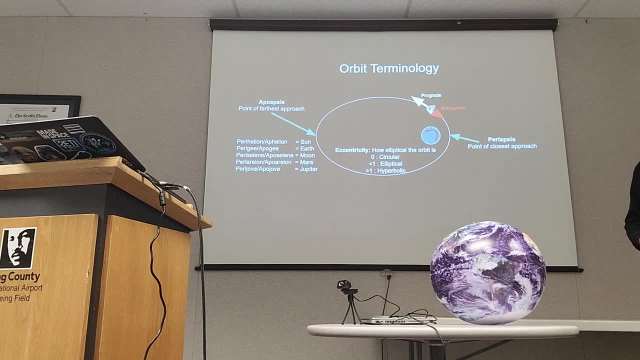 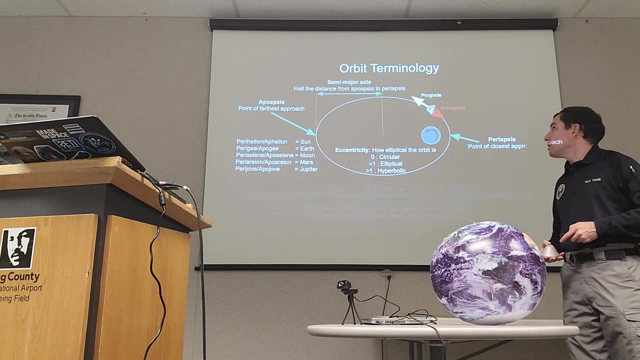 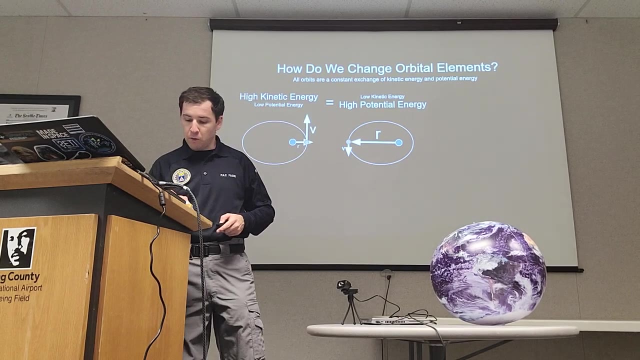 et cetera, et cetera. So this is useful in a mission planning context, because you might have multiple objects that you visit in the course of your flight. So yeah, that's the basics of orbital terminology and orbital elements. Now it's important to talk about. 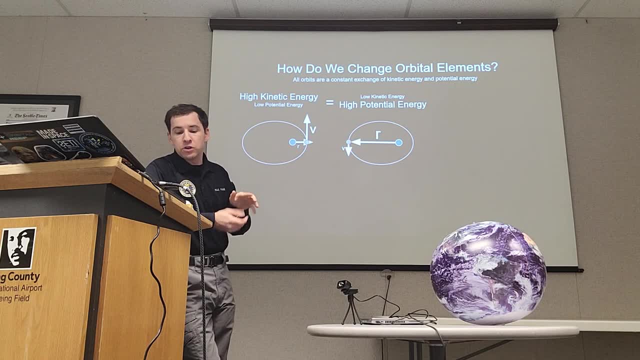 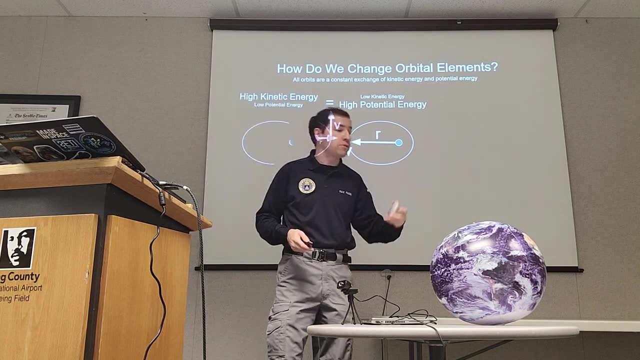 how do we change these orbital elements? because a mission profile where you're just stuck in one orbit all the time isn't terribly useful. It's useful. it isn't terribly useful for a crew spacecraft. It's very useful if you're a GPS satellite. 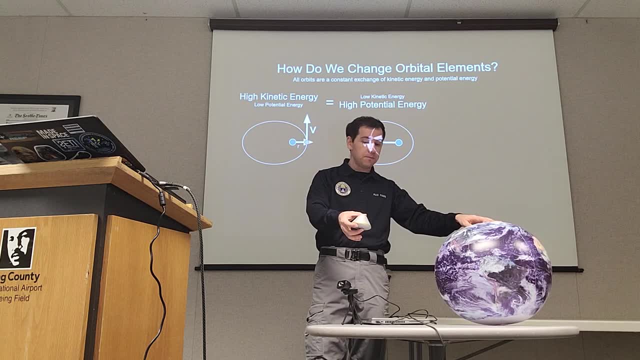 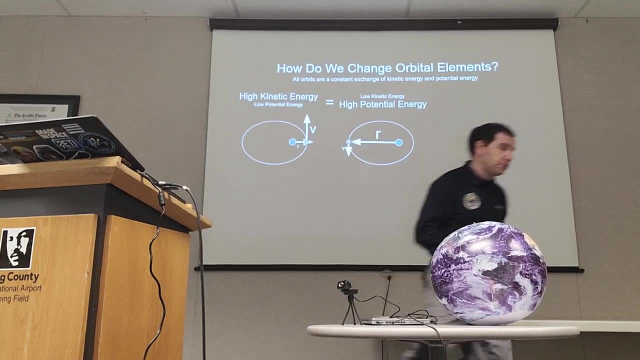 for example, the GPS satellites are in Middle Earth orbit. they're like about this high or so a few tens of thousands of kilometers. Or if you are in a geosynchronous orbit, a weather satellite, a geosync, something like 35,000 kilometers. 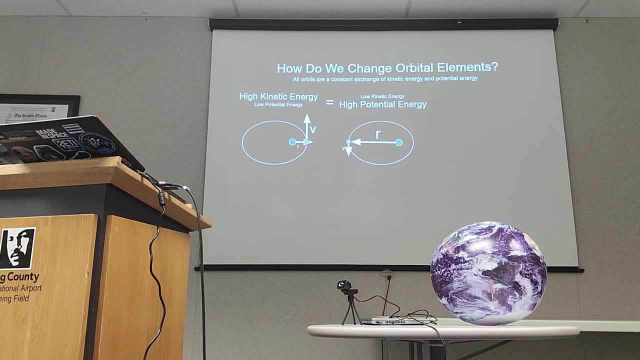 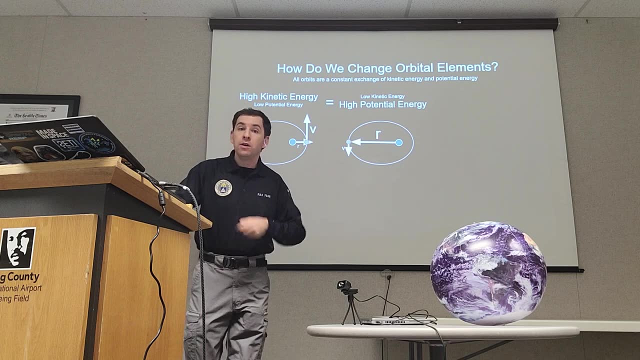 like maybe this high. it's useful to be in one orbit all the time, But for a crew spacecraft, where you're going to be traveling from one destination to another, it's important to be able to change our orbit. So how do we do that? 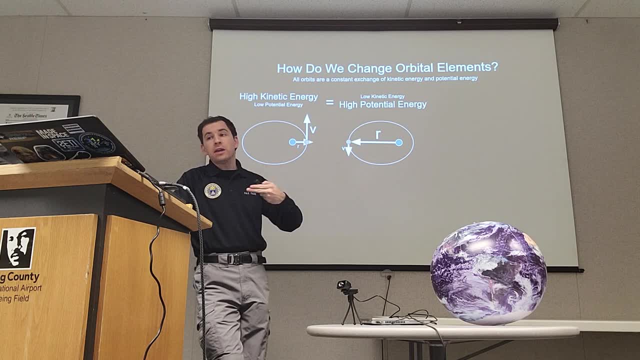 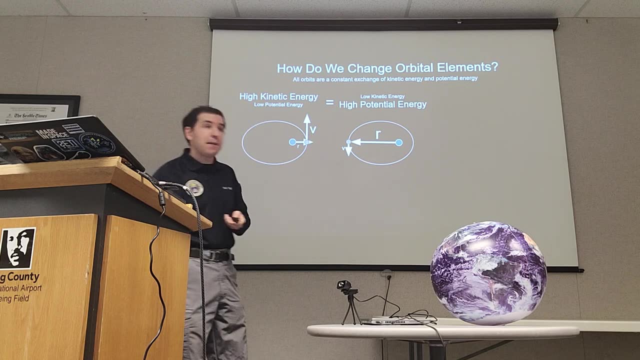 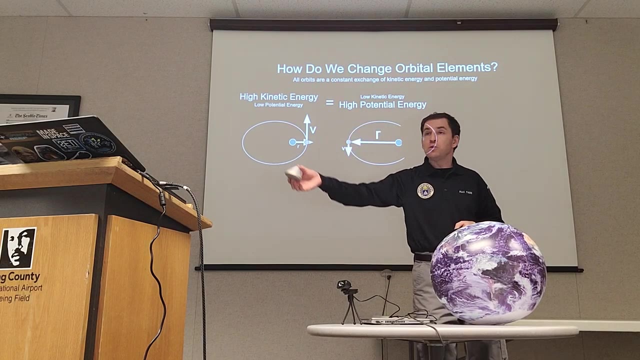 Well, we change orbital parameters by exchanging kinetic energy for the energy in our propellant system. Now this exchange of energy is happening all the time in a conventional orbit, even when the engine is not firing. If you remember from high school physics, there's two conventional mechanical types of energy. 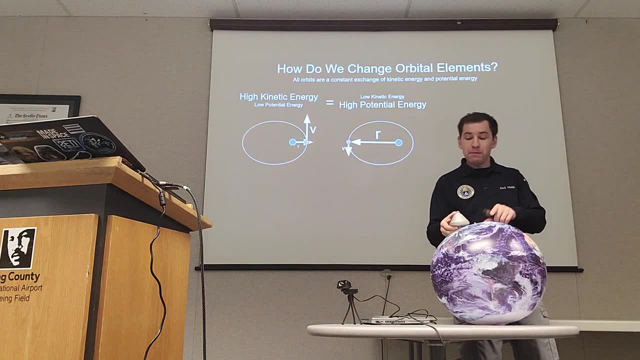 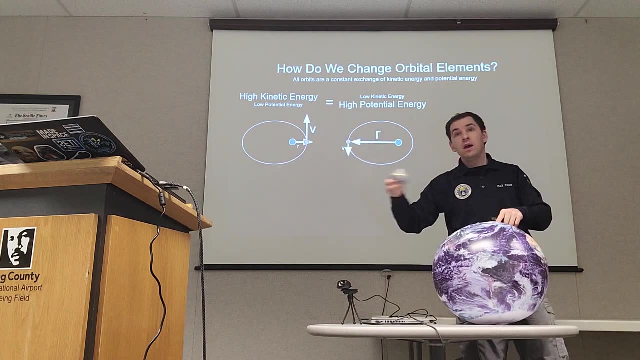 There's potential energy and kinetic energy, Potential energy being the kind of energy that's associated with something that's high up and can be dropped. Kinetic energy associated with something that is moving rapidly. A conventional Keplerian elliptical orbit is a constant exchange between these two. 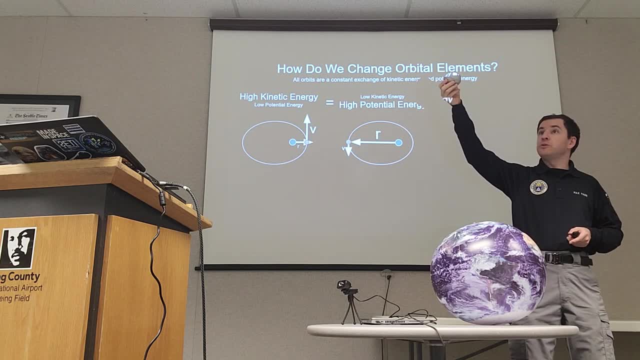 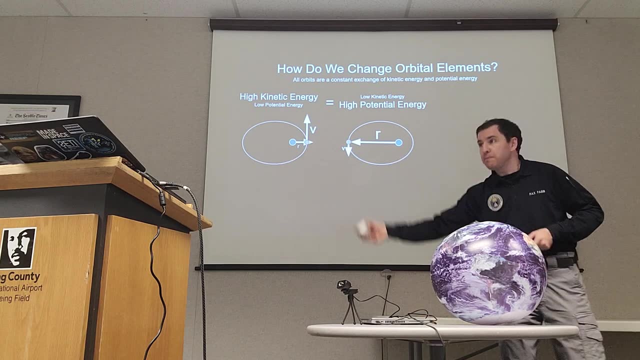 So an object in an elliptical orbit at high altitude has a lot of potential energy, but not a lot of kinetic energy. It's moving slowly And then, as it swings around perigee, it speeds up and slows down, speeds up and slows down. 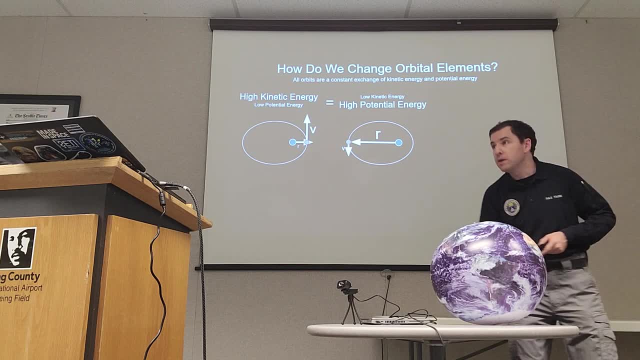 So low, near perigee, it has a lot of kinetic energy but not a lot of potential energy. High up in its elliptical orbit, it has a lot of potential energy but not a lot of kinetic energy. And it's this constant exchange. 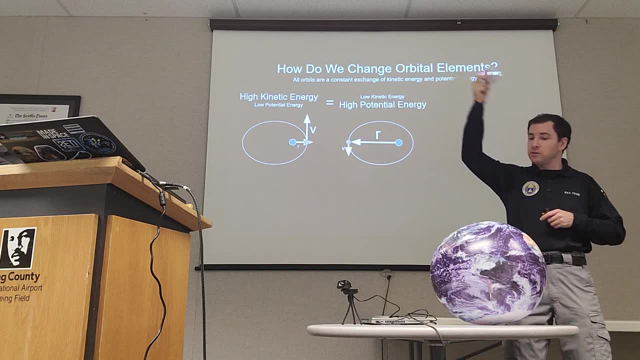 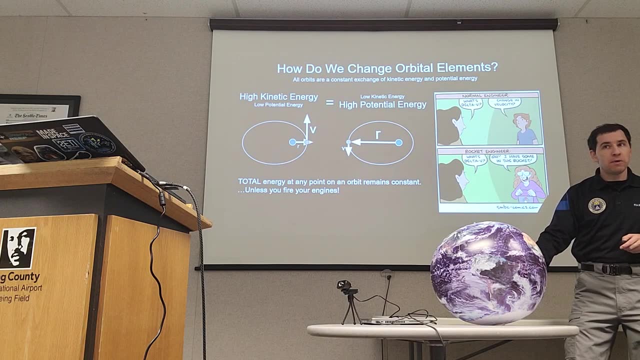 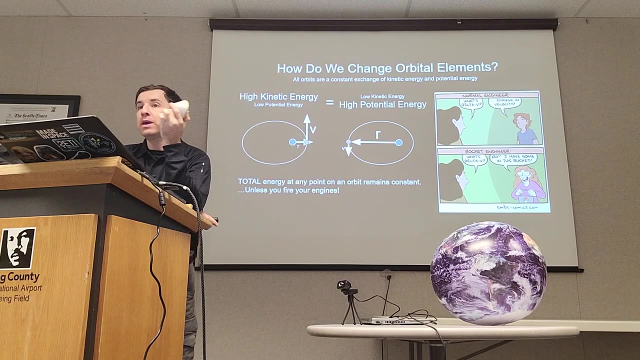 that we capitalize on when we change the orbital elements. So what if, when we're swinging by perigee, we fire our engine's program? We're now adding energy to the system. We're converting energy from our propellant tanks into kinetic energy of the vehicle. 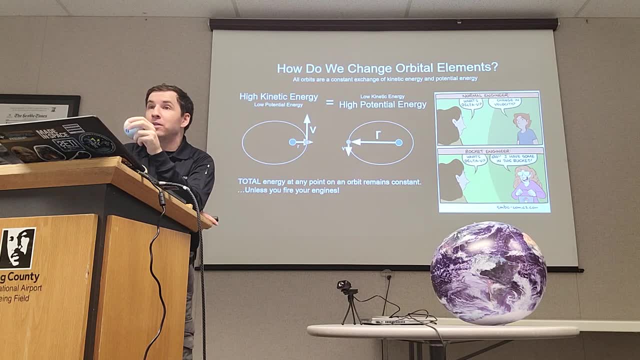 which is going to change the orbit elements, And this is why you hear aerospace engineers typically talk about maneuvers and maneuvering budgets in terms of delta-v. Delta-v is a spacecraft's capability. How much, excuse me, how much capability does the spacecraft have? 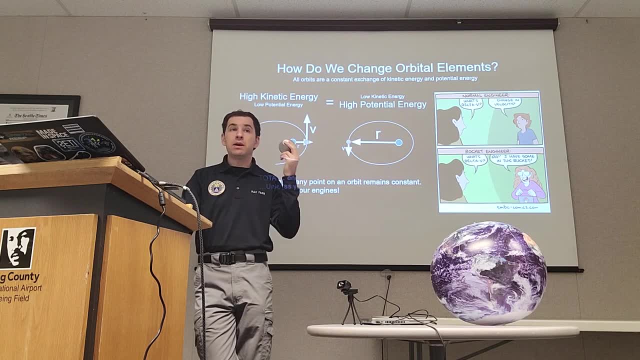 to affect a change in velocity, Because by changing velocity you're changing your energy, which means you're changing your orbital elements. So you'll hear engineers talk about delta-v like it's something we can consume. You'll hear us talk about it in the same way. 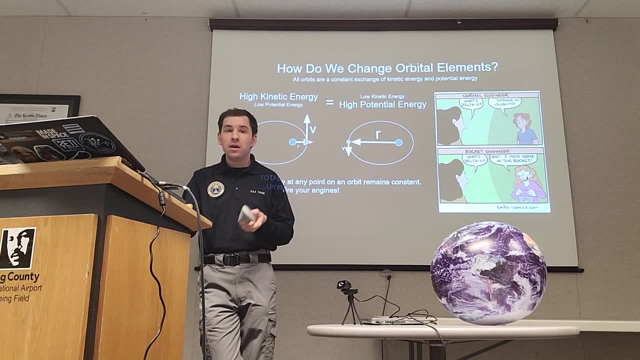 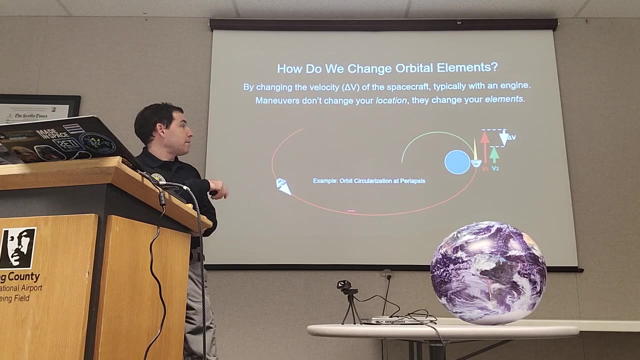 as pilots would talk about gas, budgets or fuel. It's the currency of exchange. in astrodynamics is usually spoken in terms of delta-v, So an example of that maneuver might be: let's say we're in a high orbit and it's time to come back for entry, descent and landing. 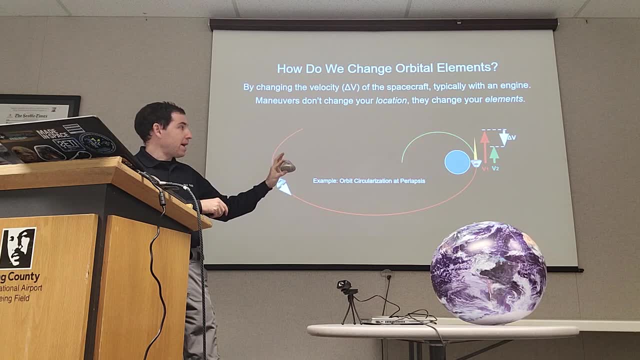 The vehicle is coming in on a highly elliptical orbit. We pass by our perigee, We fire the retro rocket's retrograde That's going to reduce our velocity from a high velocity to a low velocity, the difference being the amount of delta-v we affected. 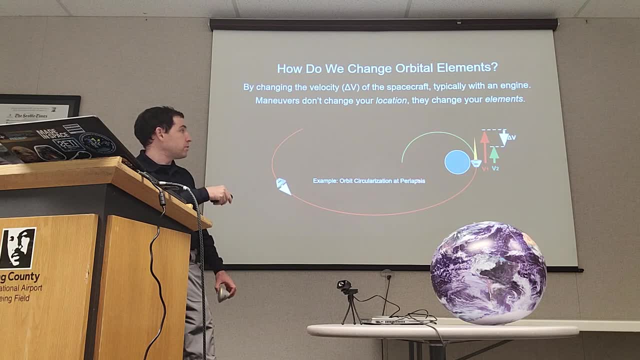 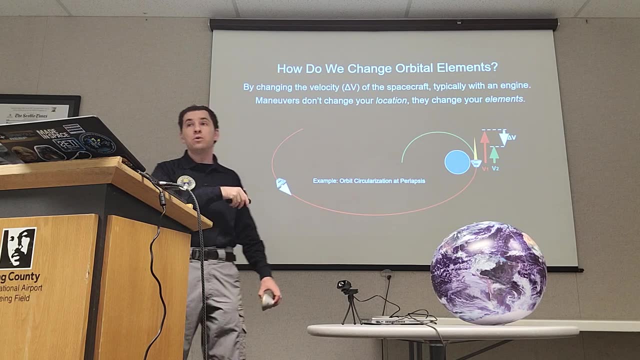 And the result is going to be moving from a highly elliptical orbit to a slightly less eccentric orbit, And then, if we do it again, we could break into a circular orbit. If we did it even more, we could break into an orbit that intersected with the Earth's surface. 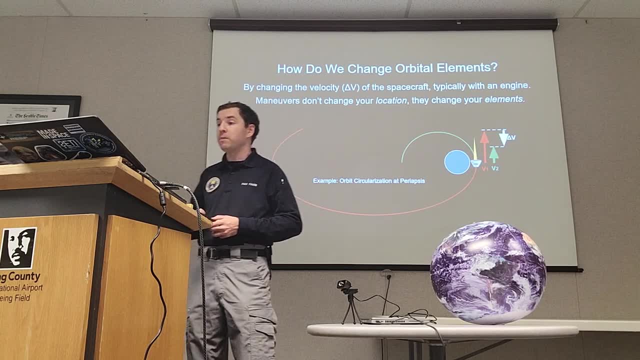 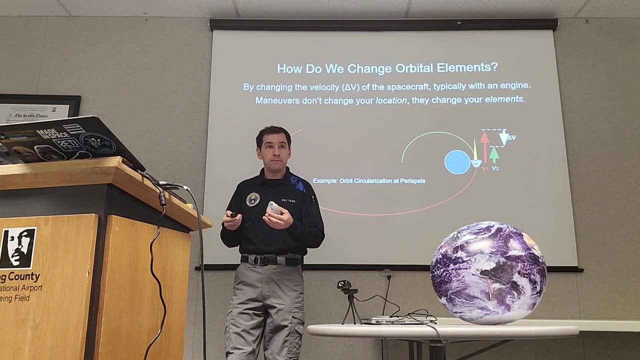 which is what we want to do when we're trying to come back from orbit. So the easiest way to think about this is the way to change your elements is by changing your velocity. Fire your engines, change your energy, change your velocity, change your elements. 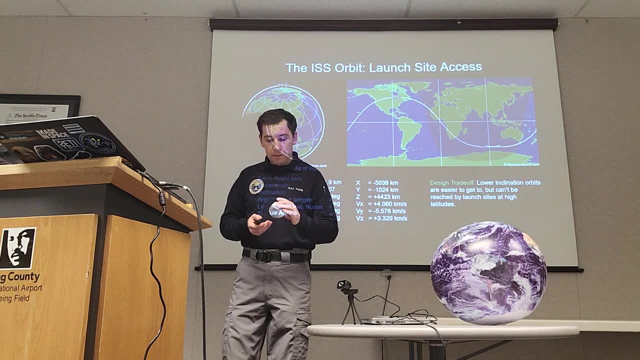 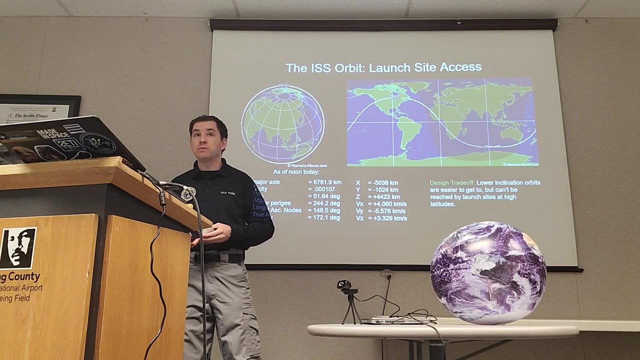 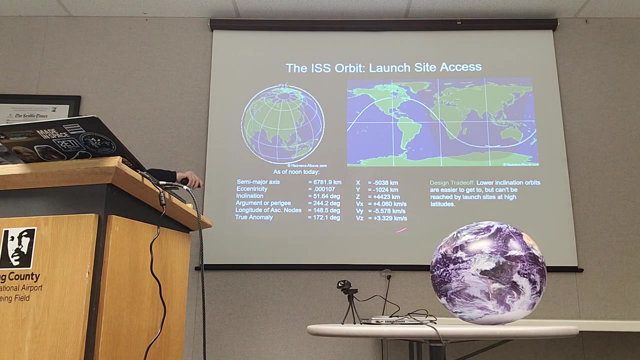 Change your elements, change your orbit. So the exchange between delta-v and how they affect our orbital elements is very important for mission planning. An example which I can show you here is the International Space Station. So I have here the conventional elements of the International Space Station. 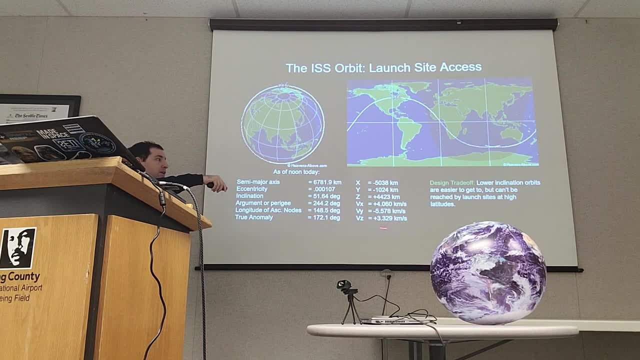 You can see, though, this isn't really very useful. This isn't really going to tell us anything, because in 10 seconds, all of these are going to be different, But if we convert them to the Keplerian elements of the ISS? 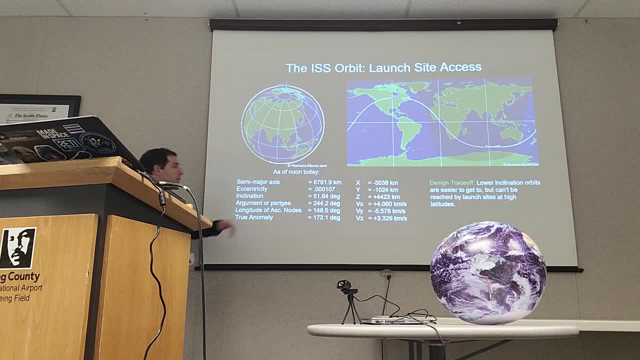 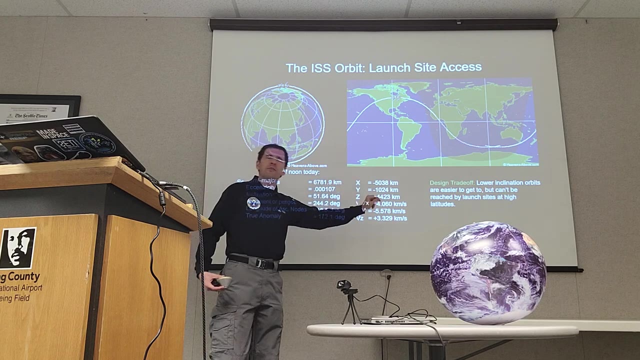 they tell us a little bit more useful information. So, for example, the ISS has a setting major axis of 6,782 kilometers. Who knows what the radius of the Earth is? roughly? No, It's 6,770.. Sorry, it's 6,370 kilometers. 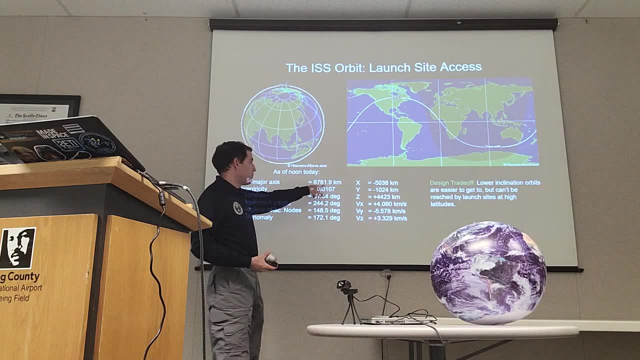 6,370 kilometers. So if the Earth's radius is 6,370 kilometers, we know the ISS here is about 400-and-something kilometers high, So that tells us something useful. This wouldn't really tell us that because you'd have to do the Pythagorean theorem. 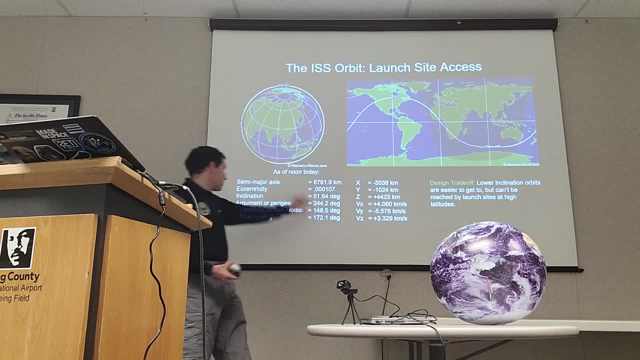 with these three components to figure out the actual radius of the Space Station. The eccentricity of the ISS, very, very small, tells us it's in a roughly circular orbit, which is good. The inclination, 51.6 degrees, is a historically picked number. 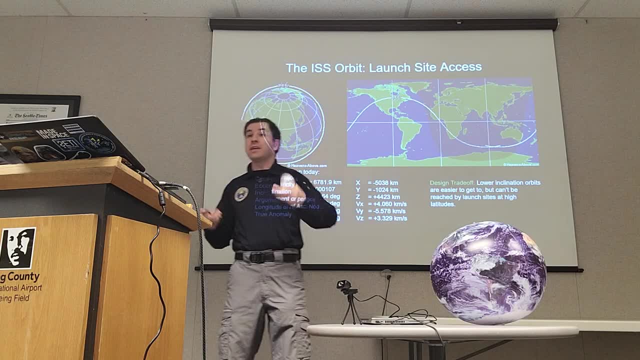 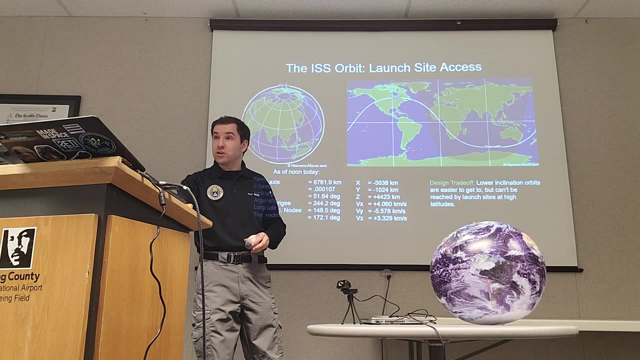 So lower inclinations are easier to launch into because you can launch due east and capitalize on the rotation of the Earth. But the International Space Station is an International Space Station. It's right there in the name. It's not just assembled out of Cape Canaveral. 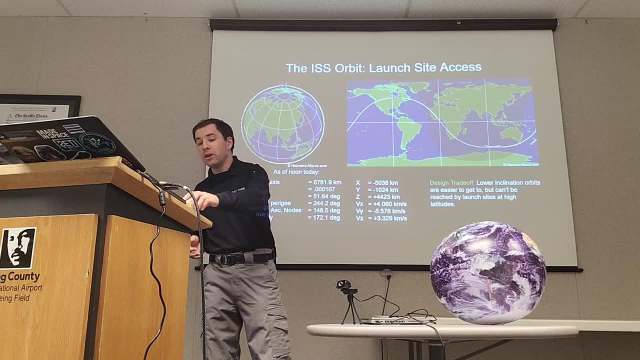 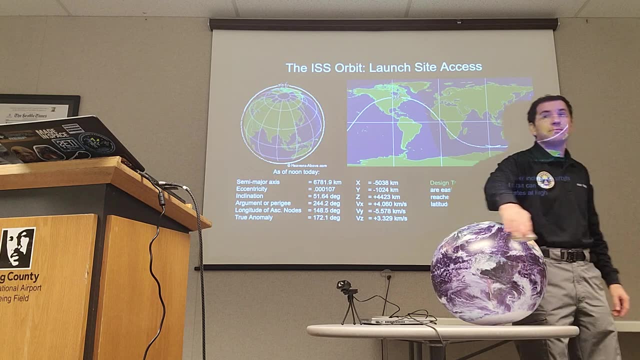 There are components of the International Space Station that needed to be launched from Russia, And an orbit with a low inclination that always stays over the equator is never going to pass over Russia or the Soviet Union at the time when this planning was done, So it was necessary to increase. 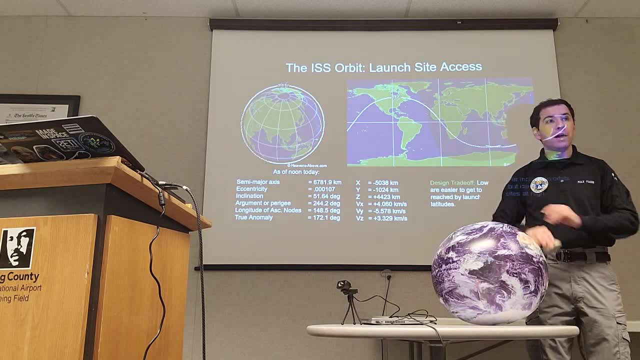 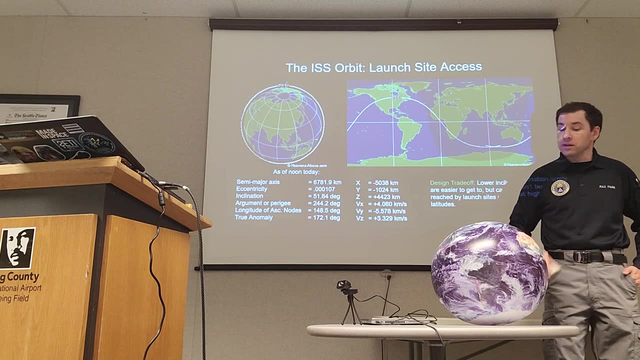 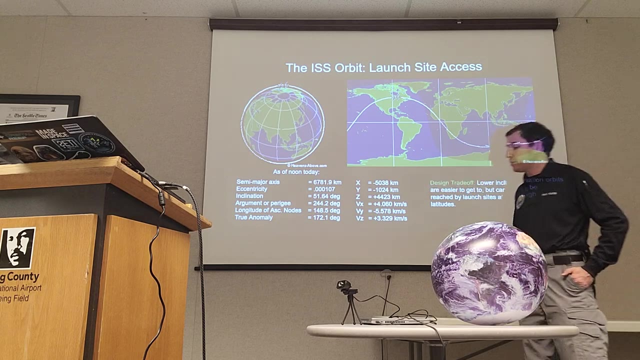 the inclination of the ISS, so elements that were launched from the Soviet Union could reach it. Otherwise there'd be no way for the Russian elements to get up there, And inclination changes are incredibly difficult afterwards- They're as expensive as launches. So once the ISS was in this 51.6 degree orbit, 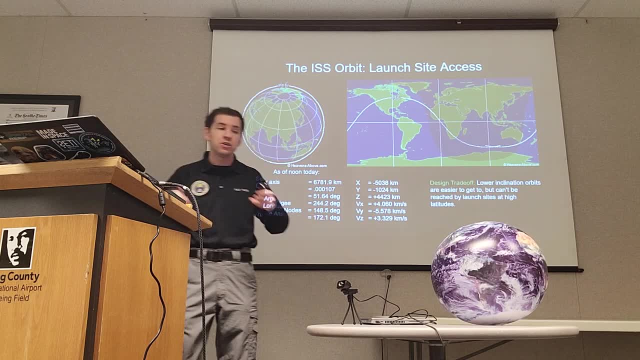 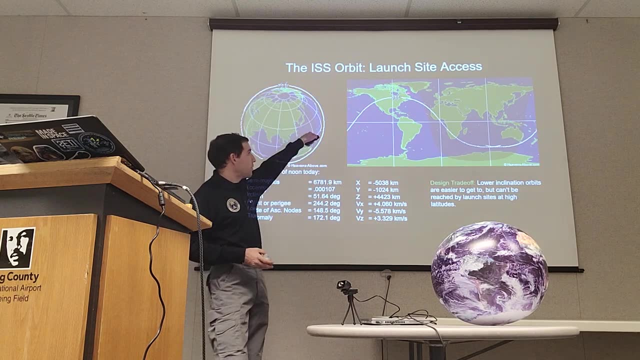 there's really no reason to move it off of that. It would take as much delta-v, as much rocket power as it did to launch all of these elements in the first place. So the orbital inclination of the ISS tells us something about how high latitude 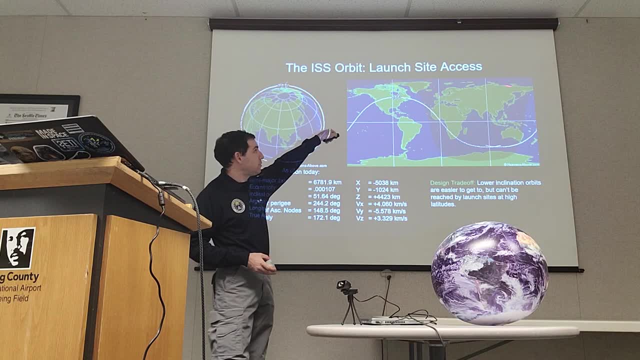 north and south it will go. You can see, it goes to a high enough latitude that it crosses over a significant portion of the Soviet Union, which is how they launched to it out of Baikonur and Kazakhstan, which is right here. 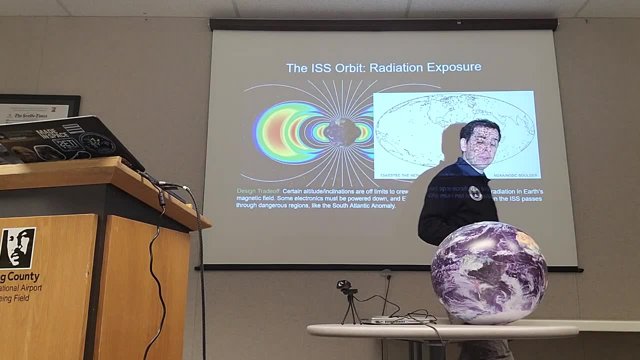 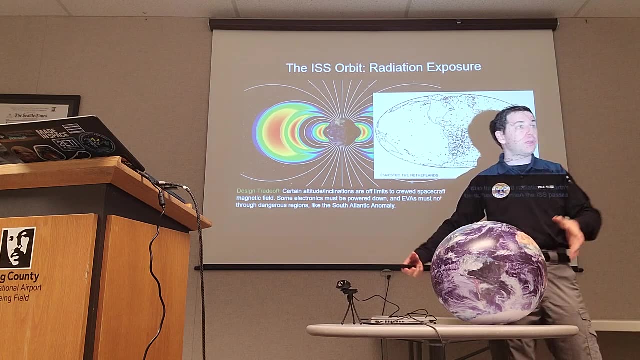 Radiation is another factor that's impacted by our selection of orbital elements. The Earth has two significant radiation zones called the Van Allen radiation belts, one of them kind of at low inclination, low altitude, and another one at higher, at a wider inclination band and a higher altitude. An orbit with a low inclination is going to spend a lot of time inside these belts, whereas higher inclinations will kind of get out of them for a significant period of time. Of course, if you're at a very low altitude, you're never touching the belts. 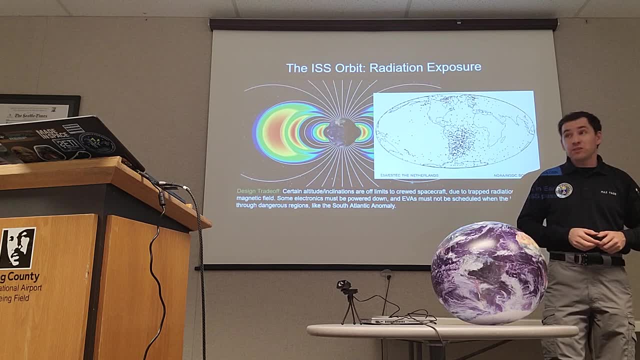 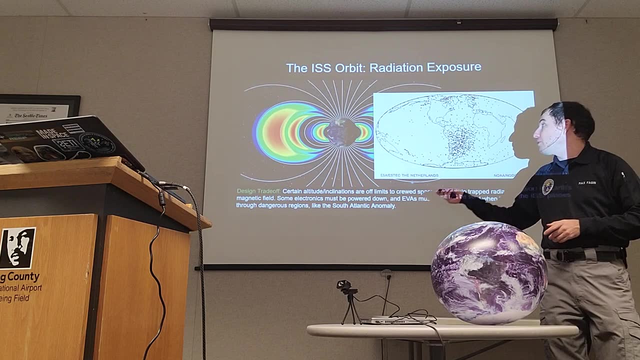 but if we go up much above 1,000 kilometers or so, that's a lethal dose for astronauts in a matter of weeks to months. So it would be very unhealthy for astronauts to hang out inside the Van Allen radiation belts for an extended period of time. You could fly through them just fine, like the Apollo astronauts, for example, only spent a matter of hours inside the Van Allen belts, but you wouldn't want to set up a space station at a high enough altitude that it impacts the Van Allen radiation belts. 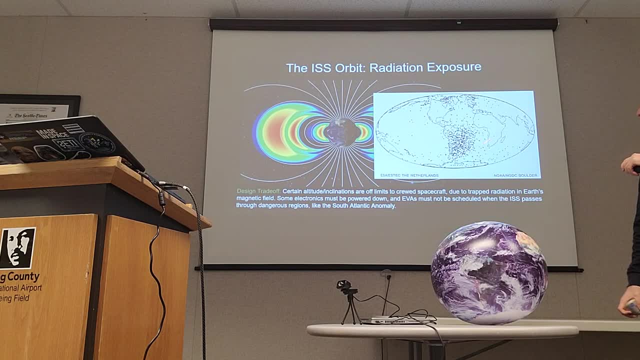 It matters for computers too. This is a kind of fun map. This is a map of all of the locations that a flight computer on board a spacecraft suffered a single-bit upset. So this is a kind of error that computers will encounter when they're bombarded with intense radiation. 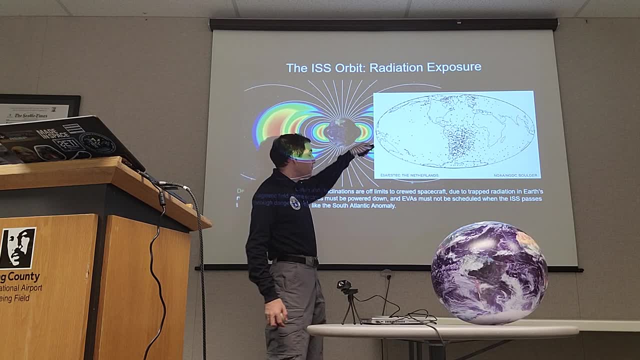 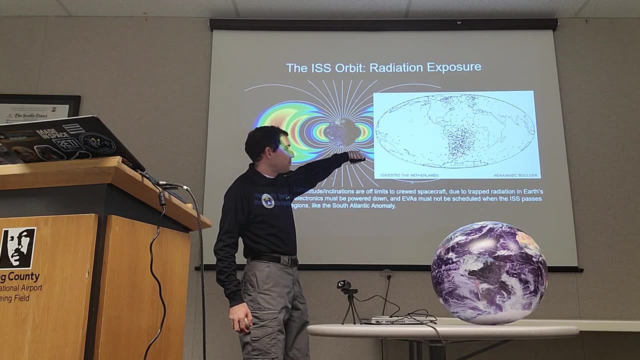 And you can see that if you put a dot everywhere where there is a single-bit upset, we get this cluster of them over South America. We call this the South Atlantic anomaly and it is a known hole. it is a known region in the Van Allen belts. 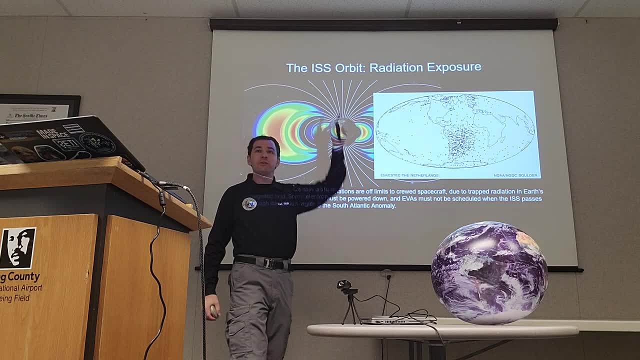 where the radiation dips down to a much lower altitude, And any time a spacecraft is passing through the Van Allen belts, it can take a radiation exposure four to five times higher than it would the rest of its orbit. For operations on the ISS, we don't schedule EVAs. 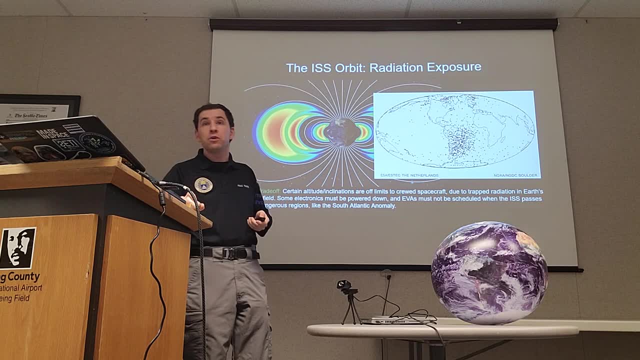 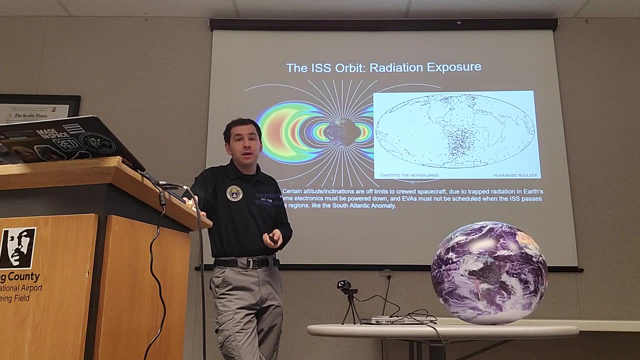 when the ISS is going to be passing through here. in order to keep the astronauts' dose low, It's important not to schedule really critical operations when you're passing through the South Atlantic anomaly. Lots of important changes need to be made in order to avoid that radiation dose. 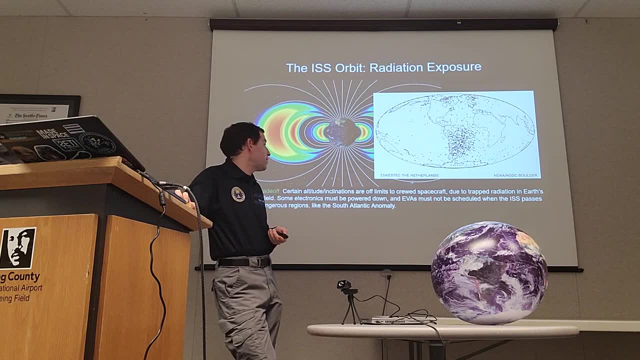 And by proper selection of orbital elements you can minimize the amount of time that you're going to spend inside the South Atlantic anomaly. Is there an impact on aviation as well? I want to say yes, but I'm not aware of any data that indicates. 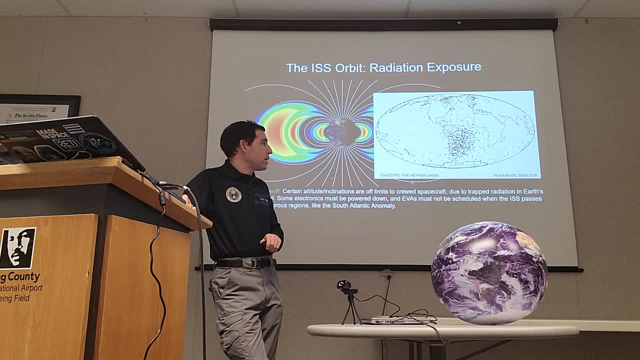 it would be the case. But, yes, the radiation dose would be marginally higher off the coast of South America than it would elsewhere. I just don't know if it's high enough to impact aviation operations, because we have 150 kilometers of atmosphere between us. 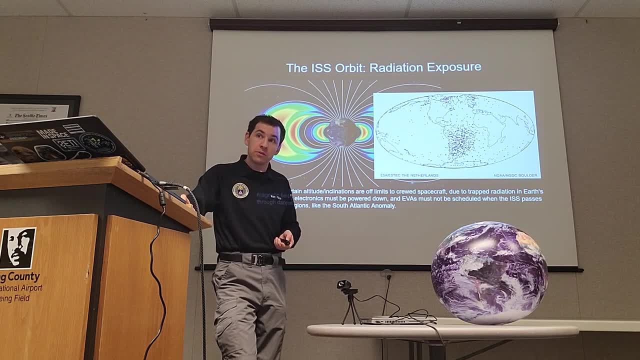 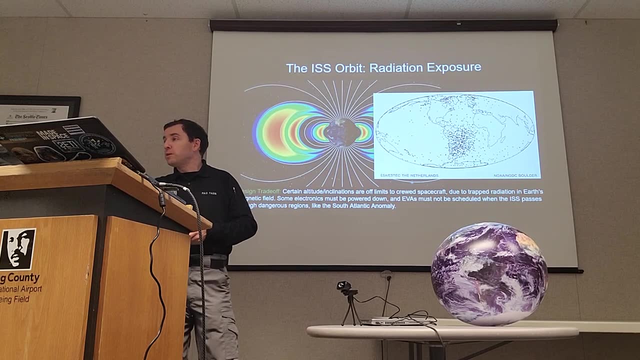 which stops the majority of space radiation. regardless of the Van Allen radiation belts, There are ozone limitations, which I don't know if that's related to the Van Allen belt, That's separate. yeah, The ozone limitations are entirely due to our atmosphere. 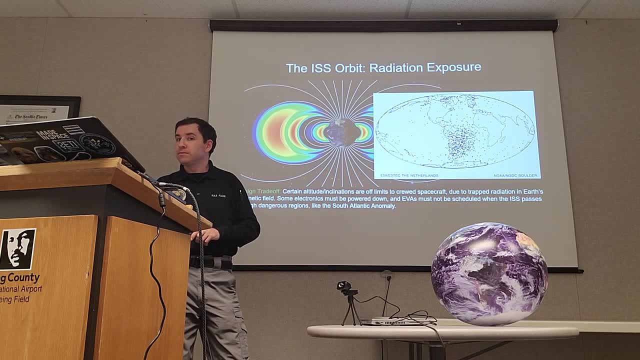 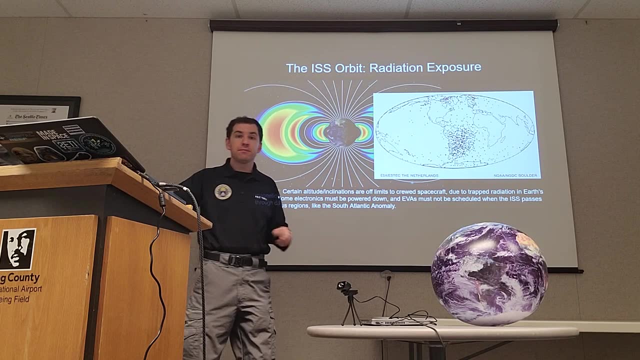 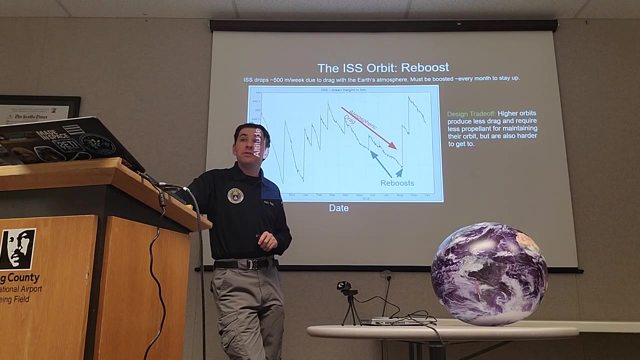 They're limited to time, altitude and latitude. Is it time of the year? Altitude selection is important from a propulsive perspective because it matters how much propellant is going to be allocated to reboosting the vehicle. So this is the altitude history of the International Space Station. 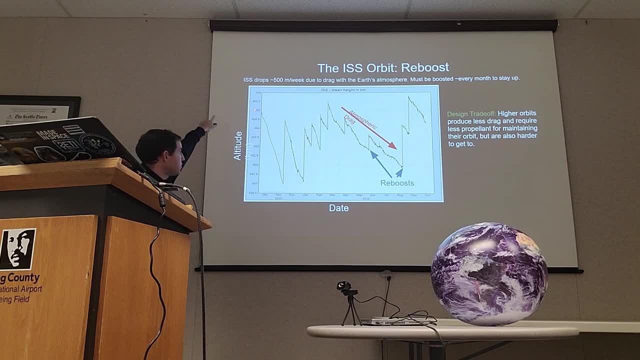 over a period of about two years. Now you notice the vertical scale is highly exaggerated here. It's a difference of 400 kilometers to 406 kilometers. So the surface of the Earth is way, way down, way, way off-scale here. 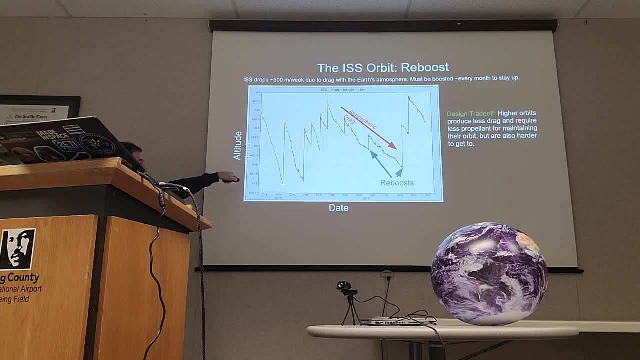 But you can still see that over a period of time, over about two months, the space station loses five kilometers in altitude due to atmospheric drag, And then every so often it needs to burn its engines again to reboost back up to a higher altitude. That's what these stair-step functions are. right here. This is the ISS firing thrusters for a few minutes to gain some altitude back. This falls off, though, with higher altitudes. Every hundred kilometers of extra altitude or so is about a factor of five. reduction in atmospheric drag. So if you don't want to expend propellant keeping your spacecraft aloft, it's good to send them higher up. Yes, Is the propellant replenished? It is not. No, We have studied very out-there concepts of spacecraft that can refuel themselves. or at least refuel their oxygen by collecting it from the ionosphere. But no one has yet found a way to make it practical or worth the time. So the lifespan of the orbit is a function of the propellant they can launch with Yep In most practical applications. that's the case Much above 600 kilometers or so. the drag is so low that you can have a lifetime of decades to centuries without reboosting. But down here, where the ISS is at about 400 kilometers, if the ISS stopped reboosting, 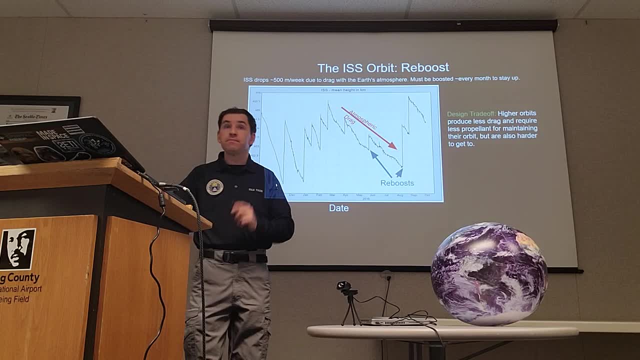 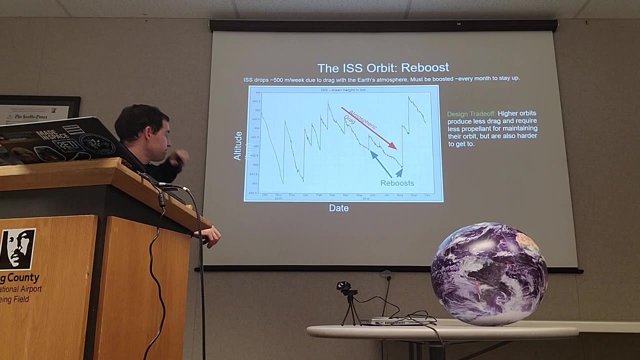 it would de-orbit in about three to six years. I was wondering about the phenomena of you've got the two significant drops in that late 2015, and they let it go for a couple of months before they reboosted, And so it does look like there's this pattern now. of. we're going to reboost more frequently, But still, if you get to like February, March of 2016,. and then they wait a while, but it doesn't lose as much. what explains that? So the altitude at which we reboost. is driven by a lot of operational considerations. One of the most common ones is: when is the Soyuz going to be coming up to visit the Russian Soyuz? The Soyuz likes us to be at low altitude. It's not a very high delta-V vehicle. It's much easier to do fast rendezvous with the Soyuz when the ISS is lower. So if we know that there are going to be multiple visiting vehicles coming in pretty soon, we'll just let the ISS get a little bit lower and make it easy for the visiting vehicles. 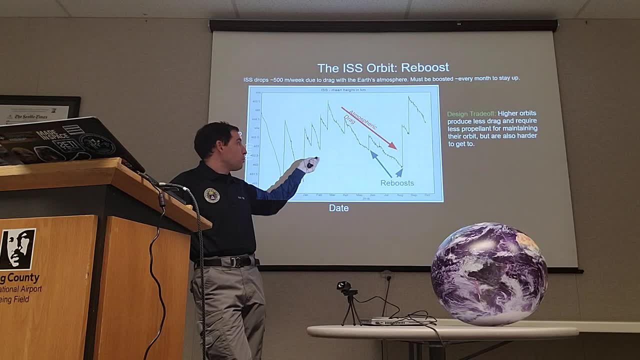 But it also matters we want these reboost periods. they disrupt the microgravity on the space station. A key selling point of the International Space Station is we can offer researchers extended months with minimal interruption to their microgravity environment. But when we turn this on, 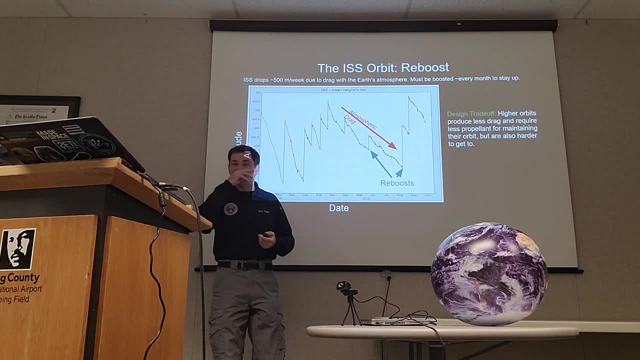 things start falling to the backside of the spacecraft. It's a very small acceleration, but you can still feel it. you can sense it. So that's going to be a disruption to all of the things on the ISS that require zero gravity. We don't want The best time to do this. the best time to do these reboosts is actually when a visiting vehicle is on station and the visiting vehicle can push the ISS. That doesn't require tapping into the ISS's propelling budget. 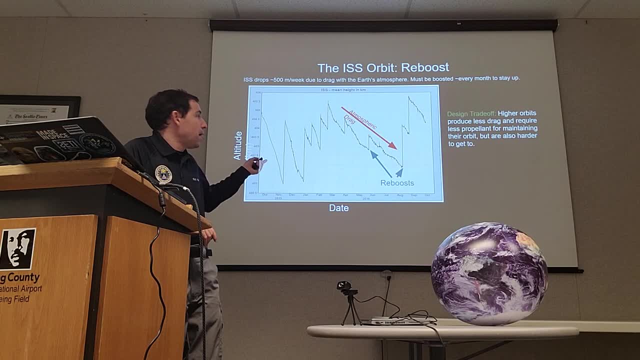 So when these reboosts happen, it's a combination of multiple operation factors, with dozens of team leads getting together and deciding when the best and least disruptive times for them are, But that's why they're not regular recurring periods. That vehicle is also a culprit, too right. Because that vehicle is adding mass. right, It is, but it's still much easier for the vehicle to do the reboosting because it doesn't require transferring any propellant onto the ISS. If the visiting vehicle can do the reboost, we always let the visiting vehicle do the reboost. Because the alternative is: the vehicle has to dock with the ISS. we have to unload propellant, take it across the hatch, plug it into the ISS's propellant tanks and then have the ISS do the reboost. And that's a lot more effort than just letting. 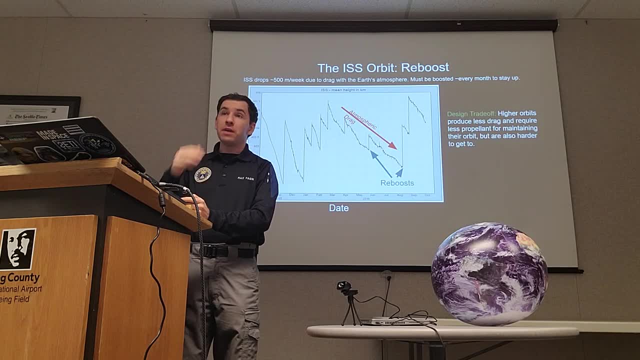 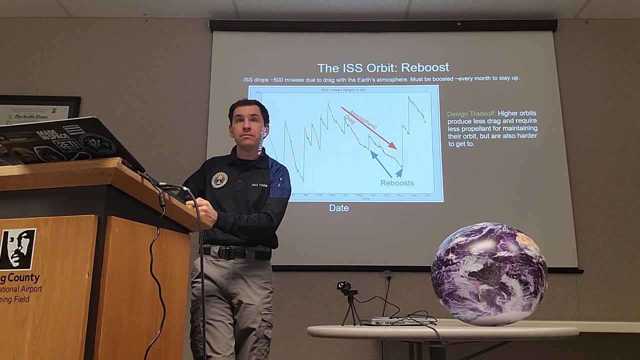 the vehicle do the pushing. But yes, a visiting vehicle can change the space station's mass by two or three percent, and that's something we need to calculate. So you talked about the disruption caused by the thrust. That was actually a project I worked on at NASA. 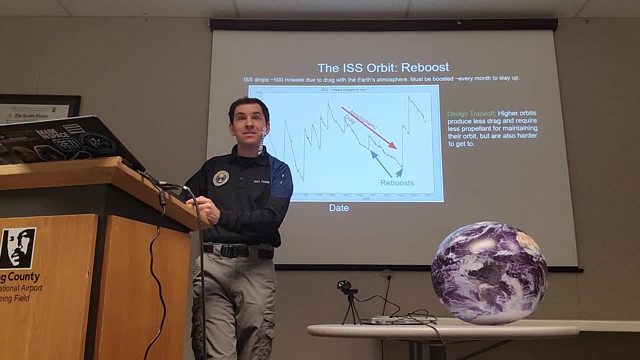 Oh really, It was a pilot control experiment and someone talked about it at another time. I really would like to hear about that. But yeah, we used an active control system and electromagnets to keep everything stable. Fun, Yeah, I'd love to hear about that. 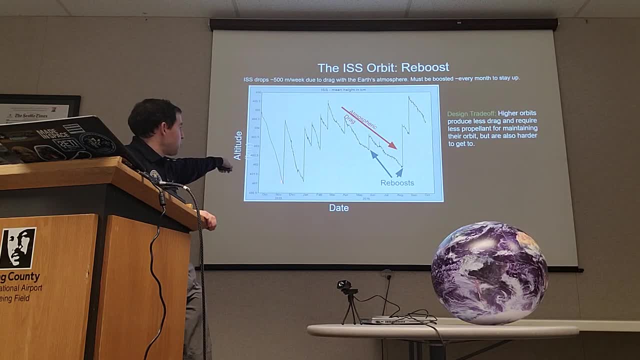 Now the second part of your question is: why is the ISS coming down? Why is the ISS coming down so much quicker here than it is here? You can see, this is about call it five kilometers every two months, whereas this is more like five kilometers. every four to six months or so. Yeah, this year it changes. Yeah, this year it changes. This was 2015,- 2016.. 2016, the sun was on the downswing of its solar cycle. The sun goes through 11-year solar cycles. and when the sun is at low activity. during periods of low activity, the atmosphere, the thermosphere and the ionosphere actually cools down, shrinks and causes less drag, And when the sun is active it bombards the upper atmosphere with radiation. with thermal radiation, The upper atmosphere heats up, swells up and the atmosphere starts to drag more. So we actually have to. it is a huge variable. It can change. The amount of drag on a spacecraft at a given altitude can vary by an order of magnitude. 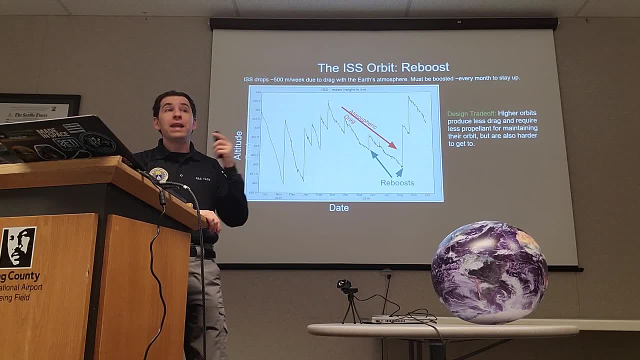 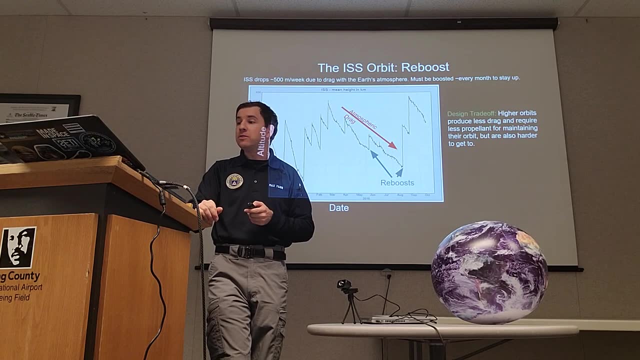 depending on whether it's solar minimum or solar maximum. Right now we are entering a. we just came out of a pretty deep solar minimum and it's starting to ramp up now. It'll peak sometime in the mid-2020s and then start to diminish around 2030 or so. 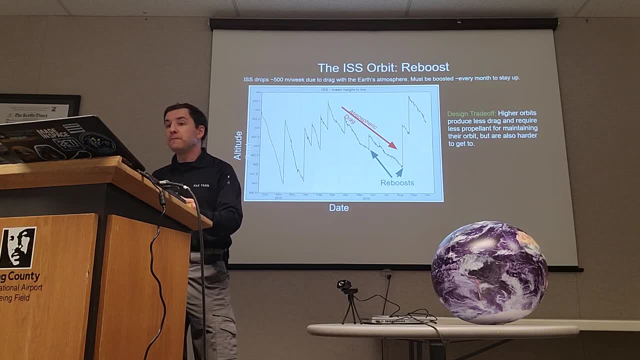 and then start to ramp up to 2031 or 2032. But yes, this is an order of magnitude effect on how hard it is to keep a satellite up there, depending on what the solar cycle is doing. Communications is another thing that is impacted by our orbit selection. 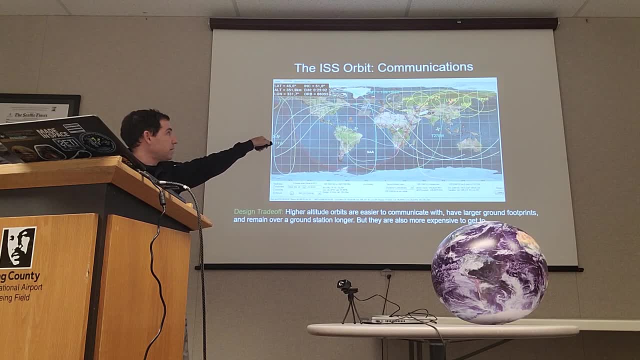 Every one of these, every one of these circles right here- it is a circle in a globe projection, but it's going to look slightly warped elliptical in a Mercator projection here- Every one of these is a ground station for the International Space Station. 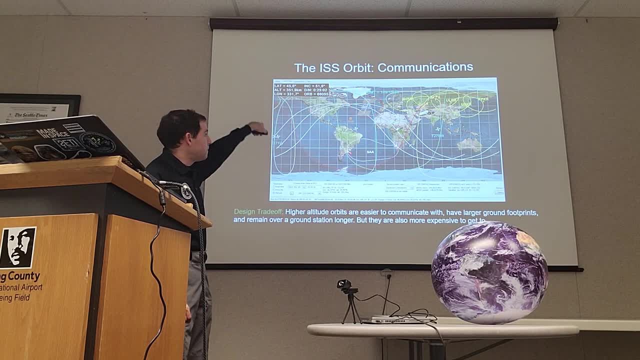 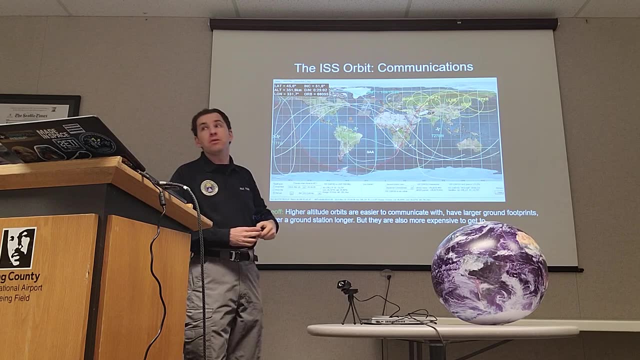 These big blue circles right here are regions that are covered by TDRS, by satellites in GEO. When we are passing through these regions, the ISS is capable of more communication than it otherwise would be, so our orbit selection matters there If we have a commercial satellite. 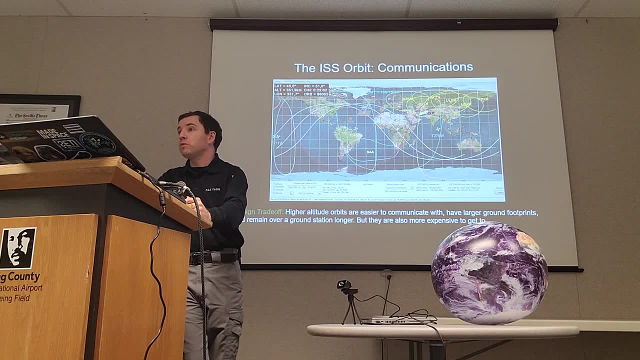 that needs to downlink all of the data. When is it going to be passing over these comm sites? How long is it going to be in sight? How high above the horizon is it going to be? All of these things are affected by orbit selection. 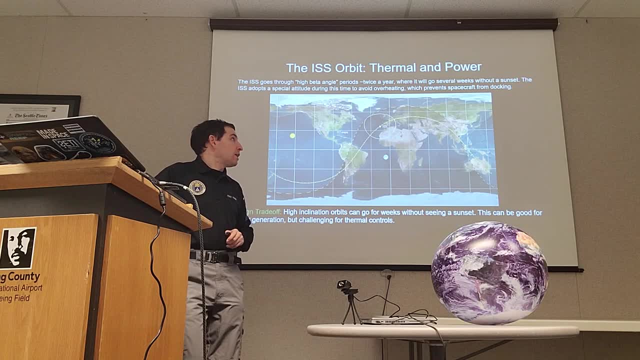 Thermal and power is impacted by our orbit selection. Right now, actually just as of yesterday, the ISS entered what's called a high beta period, where the ISS actually does not experience any sunsets. It will be that way for about another three or four days. 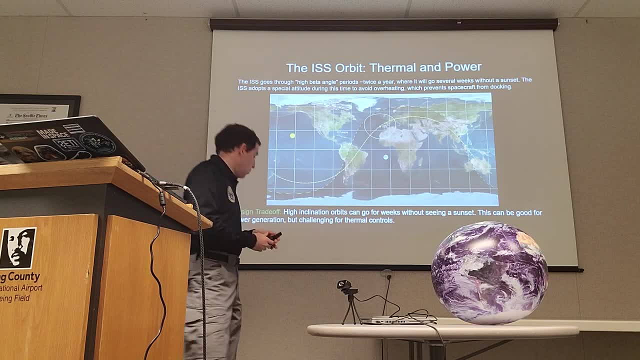 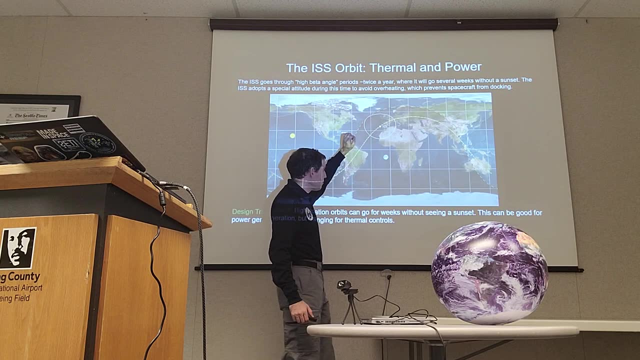 There are going to be no sunsets on the ISS because its orbit has lined up very closely here with the terminator, with the day-night terminator on the Earth, And, as a result, the ISS is going to be going through periods of full sunlight for several days. 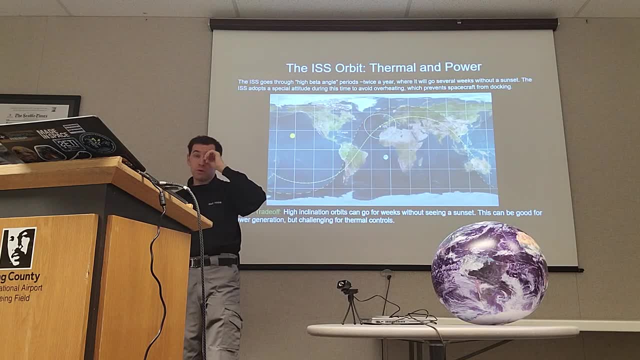 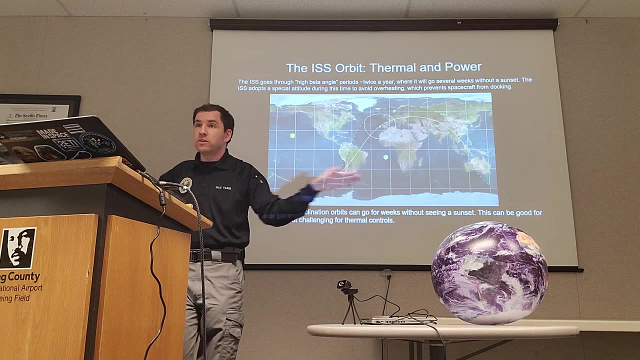 This is a thermal problem. The ISS can't operate normally during this time or else it will overheat. It's unusual for there to be visiting vehicle operations during this time. The space station sometimes has to yaw to a completely different attitude and then kind of fly sideways. to avoid overheating. It's very annoying, but it's an artifact of the fact that we need it to be at a high enough inclination to access Baikonur in Kazakhstan. We can fix this by going to a lower altitude, but lower altitude, more drag. got to launch more visiting vehicles to keep the station. Of course, sometimes we can capitalize on this. There are sometimes spacecrafts that you want to always be in the sun. If you have something that needs a lot of power needs permanent sunlight. if you have a solar telescope convenient to be able to locate it in an orbit that always has sun, then you can do that. Those are called sun-secretness orbits. Like every branch of engineering, everything I've told you here is shorthand for a lot of math. 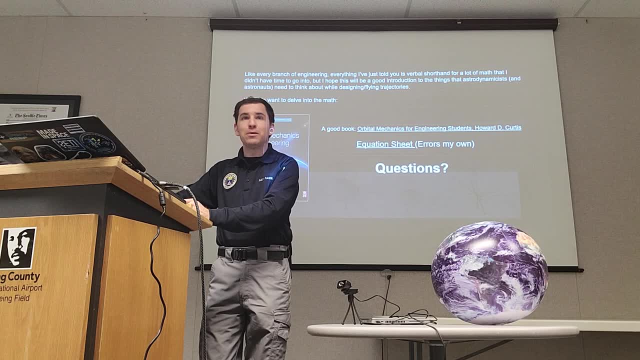 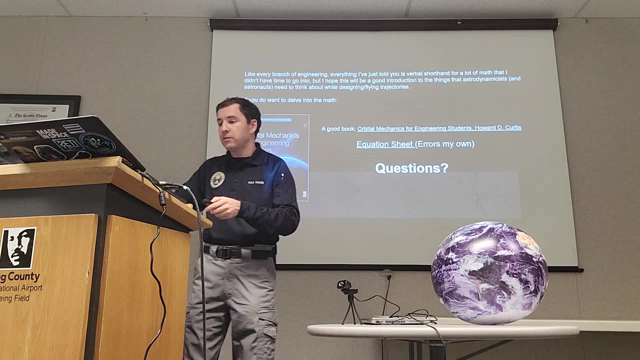 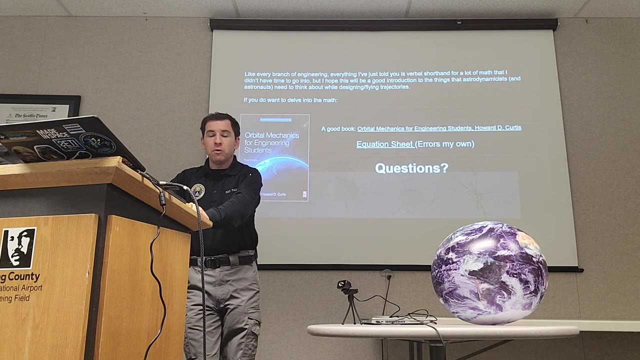 The way this is actually done is computationally, with custom software. Have you ever heard of STK or Free Flyer or anything like that? These are basically flight planners for satellites. They do the same thing that ForeFlight does, but for orbit design. 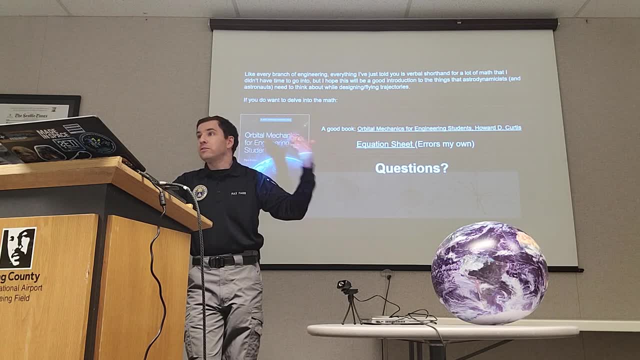 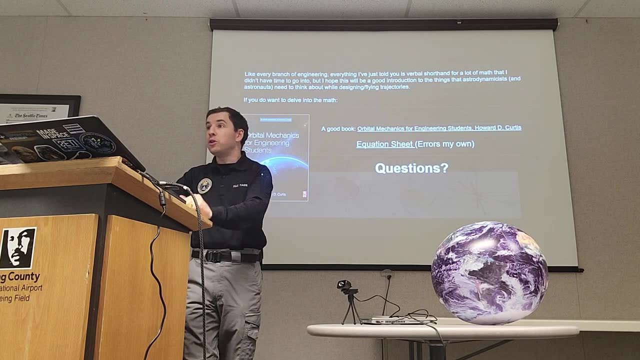 They'll answer all of these questions about communication, access, illumination conditions, perturbations due to bodies like the moon and the sun Shoves all of that math under the hood in a way that's very convenient to do and was something that people in the 60s and 70s 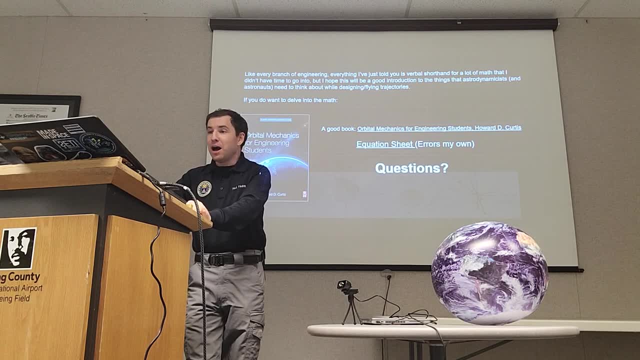 who sent us to the moon would have very much appreciated having. It's still important to have a good intuitive sense for this when you're doing trajectory design, so you know what knobs to turn and what to do And what buttons to press. So yeah, it's a fascinating field of study. and there's a lot of great resources online if you want to learn more about astrodynamics, because it's a fun perspective changer- especially when you have a mind for airplanes and you start thinking in terms of spacecraft- Kind of extends your mind to the possibilities that are out there. 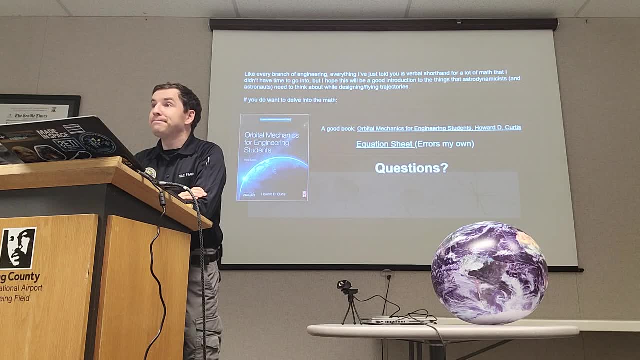 Are there any questions? Two One: I'd be fascinated to learn more about the discussions of how they came up with the six numbers. You said it took a while. There must have been a lot of back and forth. Yep, Is there a? 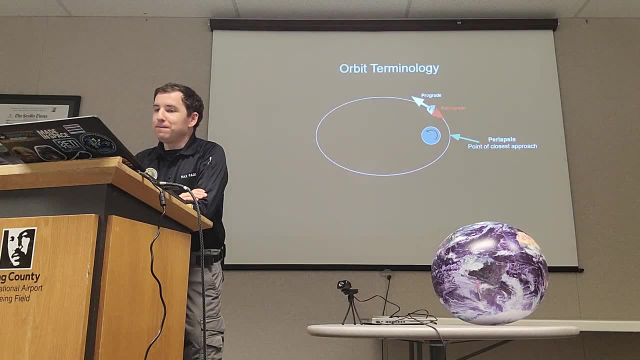 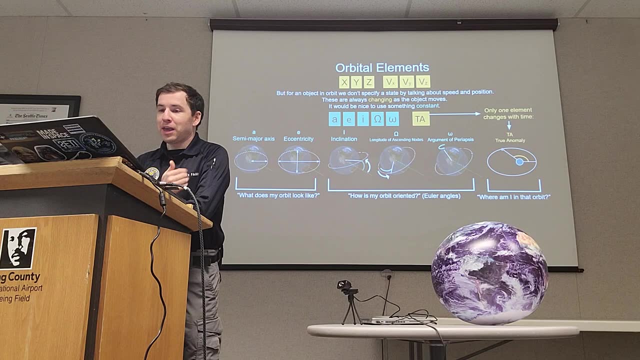 just you can point to like a sort No, it's just try and find it. Nope. And if I was to point you to the source, I would be pointing you towards Kepler, Towards Kepler and all of the astronomers whose legacy we are inheriting right here. 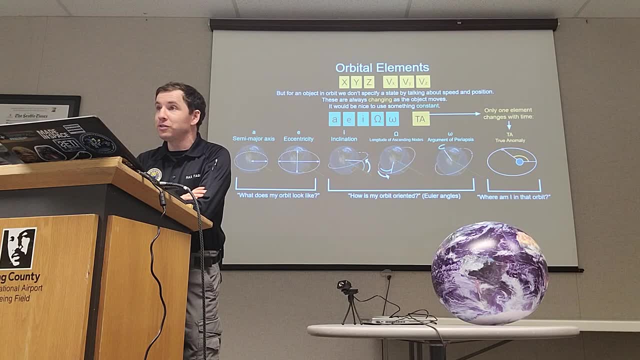 because there are not just six orbital elements, There are many combinations. You said they arrived at those. Yeah, we kind of just come to these by trial and error, back and forth, and Darwinian evolution. The papers that use these were the most. 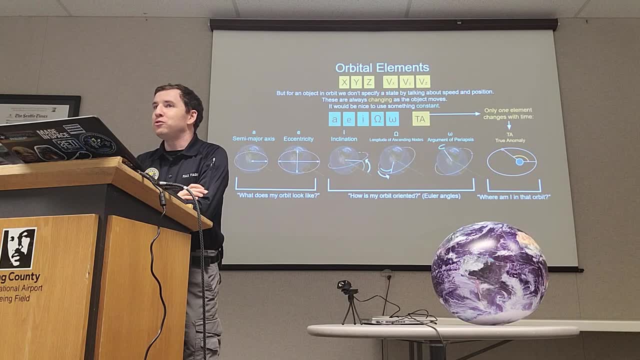 were the easiest ones to understand, Easiest to educate our students with How we came to it. And then do spacecraft still have the what I would call it an attitude indicator? We do, yes, We do Now the way we talk about attitude. 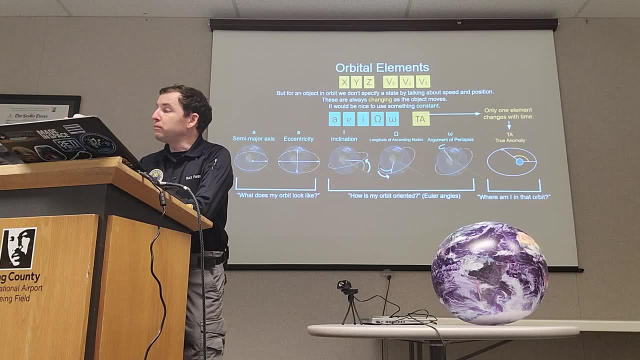 can depend a lot on what kind of spacecraft you're talking about. So a lot of spacecraft, like the space shuttle, for example, fly like an aircraft. They need to have the conventional aircraft inputs, pitch, roll, yaw, etc. Not all spacecraft, though, is. 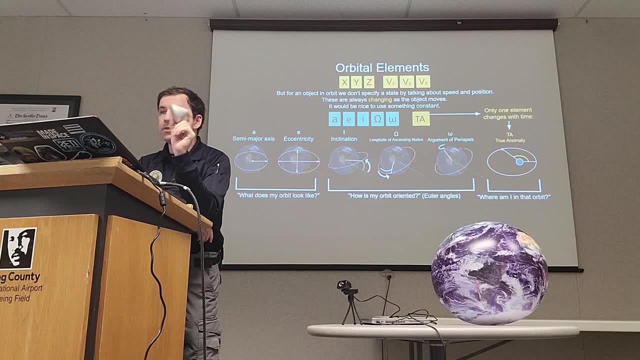 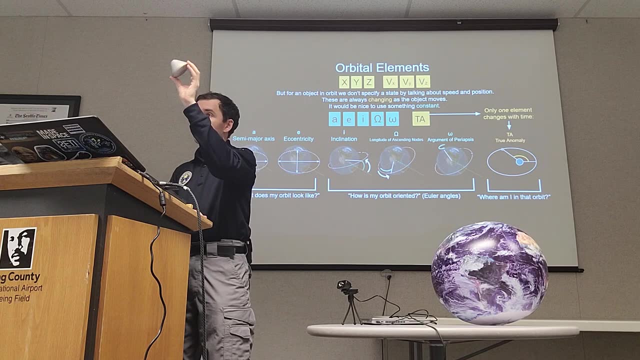 for not all spacecraft. is that a convenient way to think about, For example, a capsule like this? a capsule: when it takes off, it's flying like this nose into the wind. When it's pre-entering, though, it's basically flying backwards. 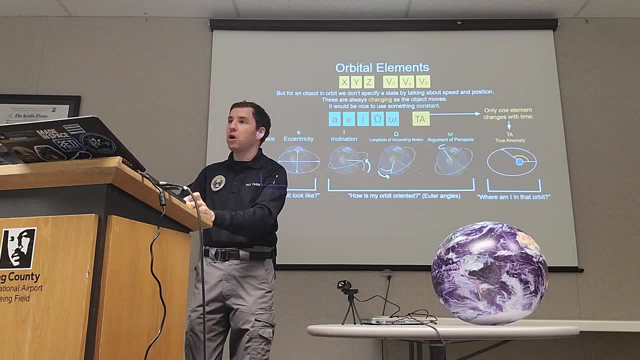 So in many cases thinking about conventional pitch roll yaw is less useful. It's more easy just to think about things in terms of flight path, angle, angles of attack and roll. But yes, most conventional spacecraft here. let me even show you the one on Orion. 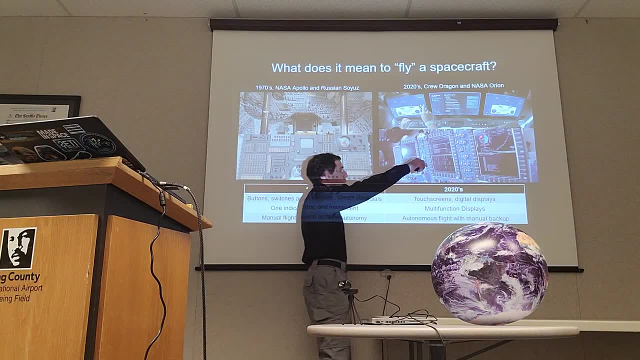 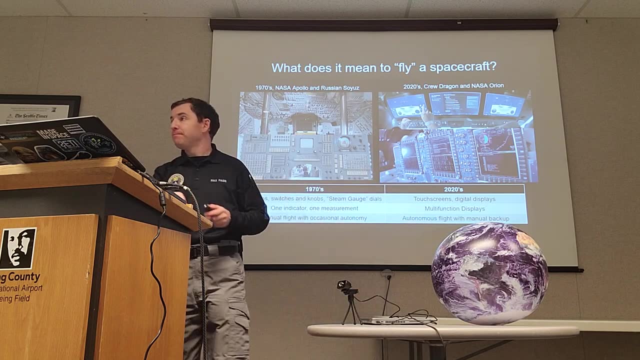 Right there. Yeah, You can see it's a digital version of a gyro. Yes, On a historical note, following up on that question, there at the Udra-Hazy Center you know they've got a big space section and you can check out all of the vehicles. 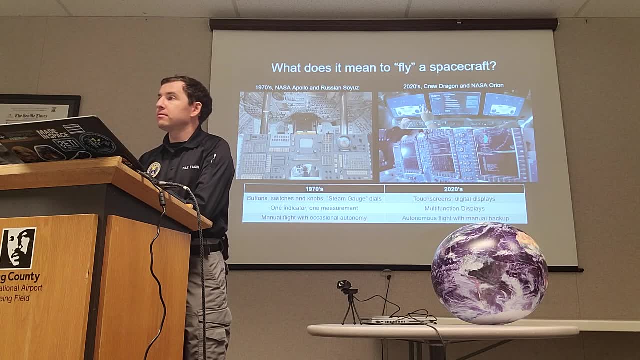 or a lot of them anyway. At one time they had a Mercury capsule. probably still have it, it's probably still there. But the first time I looked inside that thing, you know, they had the hatch open. you can stick your head in there. 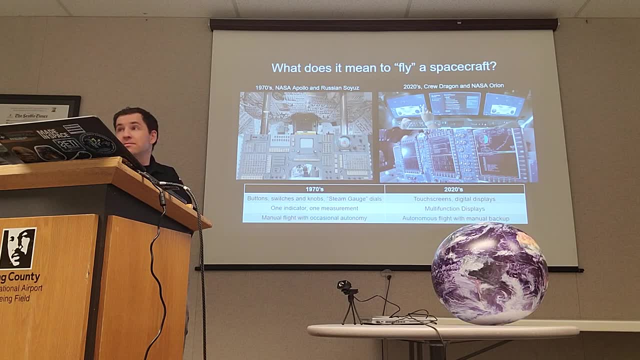 So you know they had a Mercury capsule. probably still have it, it's probably still there. But the first time I looked inside that thing, you know they had the hatch open. you can stick your head in there. It had the exact same attitude, gyro. 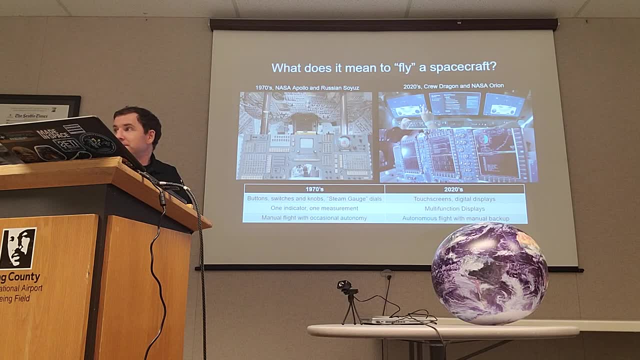 that my A-4 had. We called it an AJB-3 Alpha. I thought, seriously, These guys went, you know, went to friggin outer space with the same attitude indicator I'm planning. Well, so this right here. 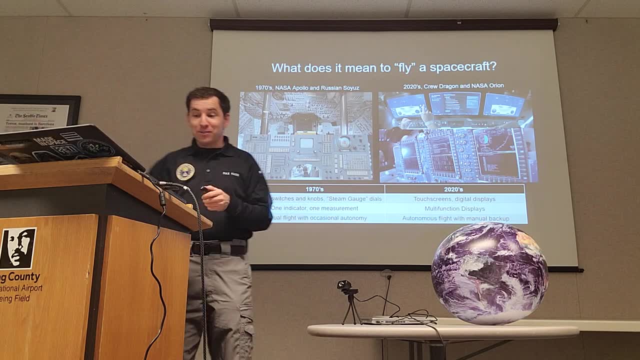 if you're looking at the Soyuz cockpit, you might be inclined to look at this and say that's the attitude indicator. It's not. That's an actual physical globe that they use to select the landing site. So if the Soyuz needs to do something, 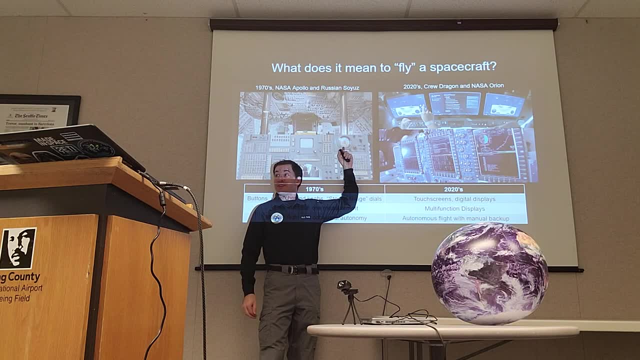 you know, you can look at this and say that's the attitude indicator. It's not. That's an actual physical globe that they use to do a manual abort and you need to select which landing site You can turn this globe. it's like a globe. 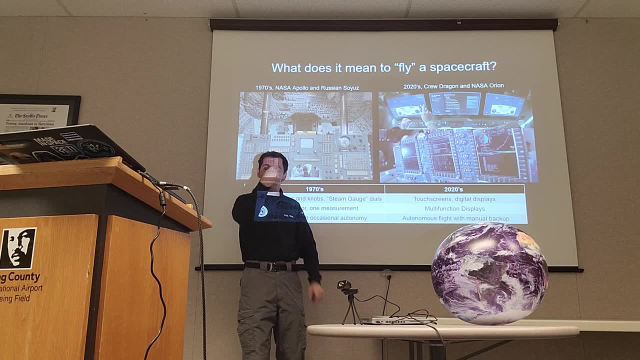 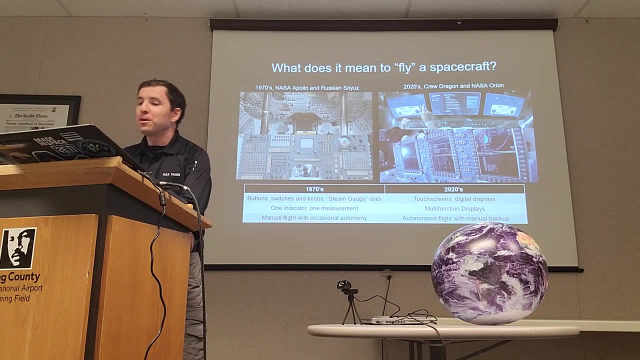 like the size of my moon globe. back there You turn it to put a crosshair physically over a three-dimensional globe in order to select your landing site. So yeah, it is a early space programs had a very had a very hardware-intensive. 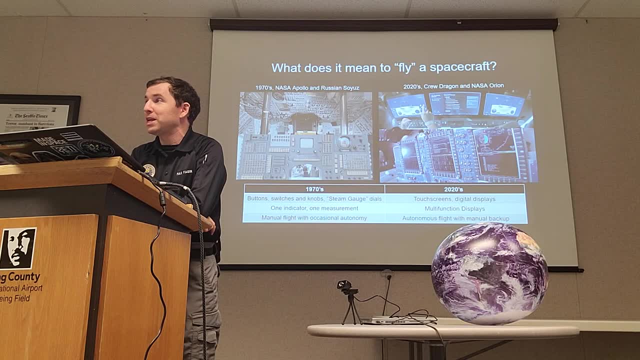 avionics setup. That's true for Mercury, that's true for Gemini, that's true for the Soyuz. When you do this, you're going to be able to do what's called the speed of light. Yeah, It's just a. 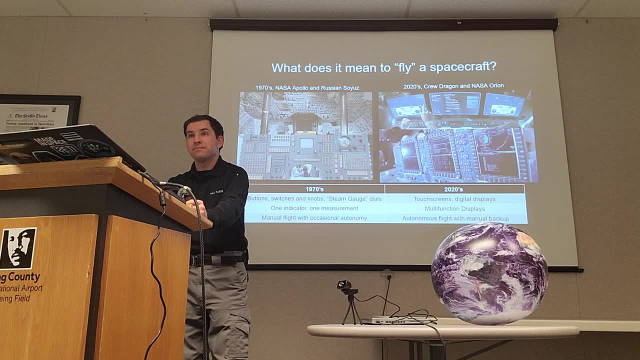 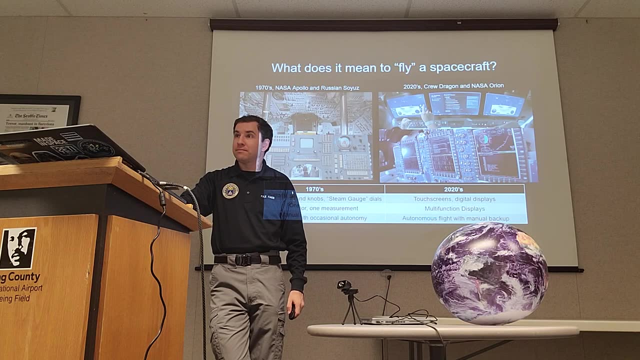 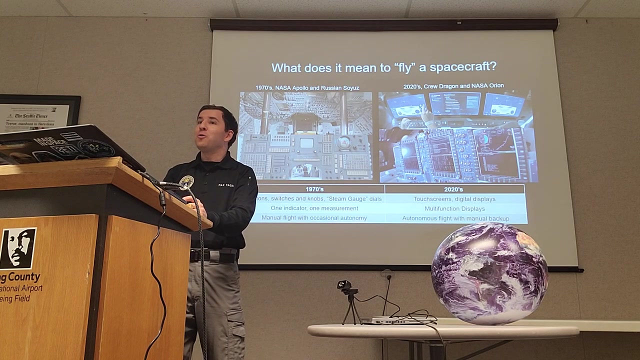 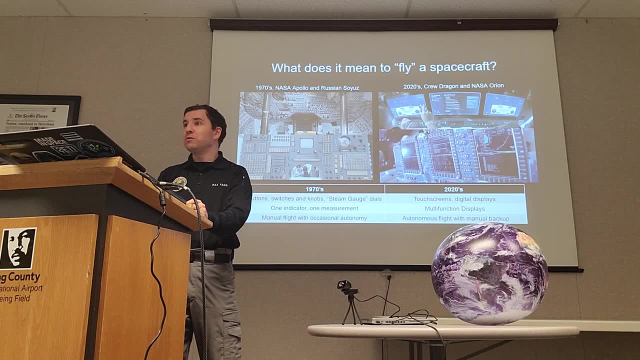 um. so for most of these situations, if you had a human fly that fly completely manually, it's likely we would exhaust our propellant budget. doesn't mean doesn't mean that we've given up on humans controlling them. it just means we understand that this is an emergency. only the majority of the 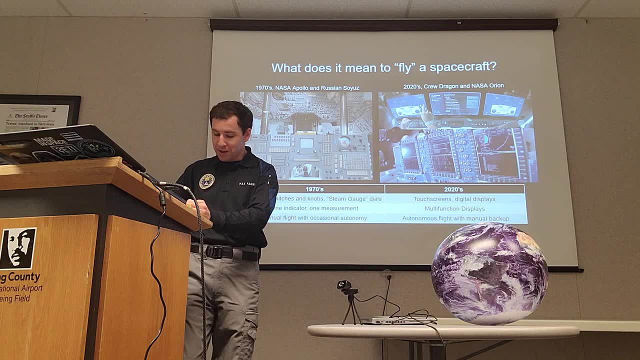 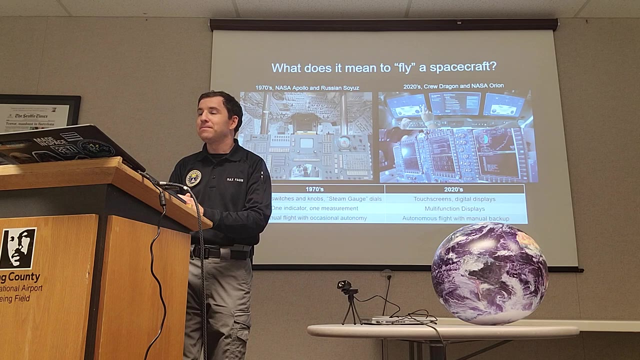 flight is done by computer, because computers are just way better at squeezing um, squeezing out that last tenth of a percent of optimization out of a, out of a propellant budget that already only has five tenths of a percent of margin in it. so most missions are probably planned that with that margin. 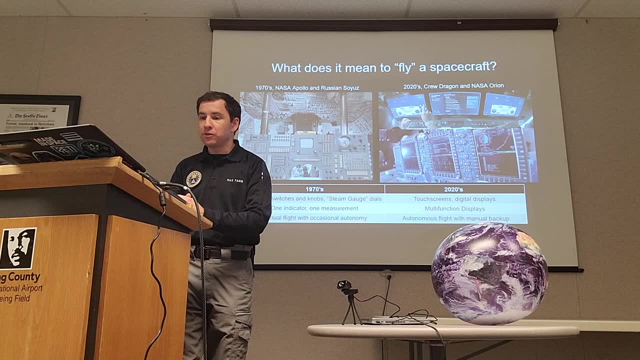 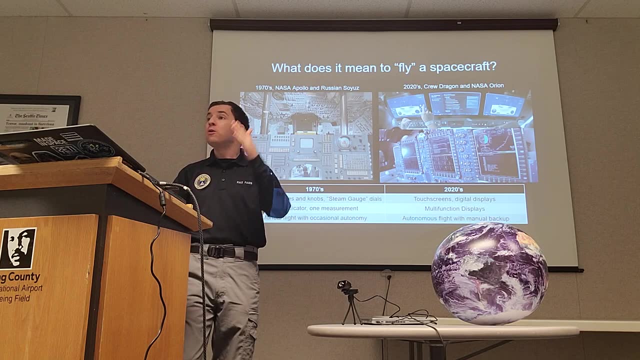 and yep, yep, and over the last, over the last 60 years, we have developed standards about what is a fair margin to carry into this. you know, the same same way, where we have rules about 45 minutes of endurance flying before you have to land, we have the same rules about propellant. 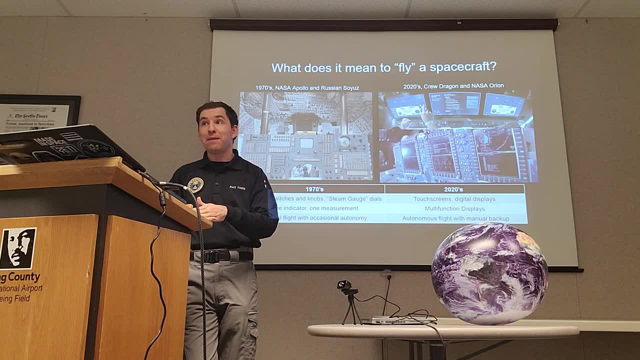 margins and propellant budget budgets. but it's not, it's a. it's not that big, it's not as big as we're used to thinking. with propellant budgets in um, in uh, in aircraft we are talking a conventional mission budget. um has margins of a few. 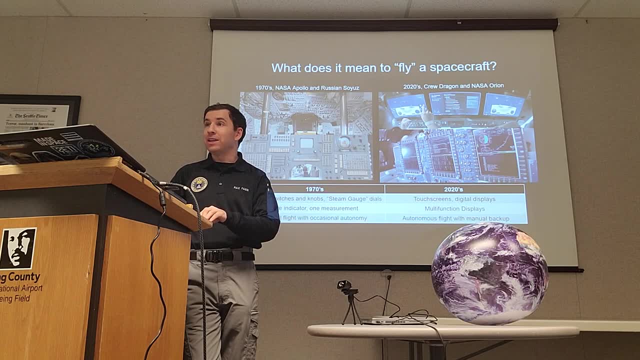 percent. if that i mean the apollo 11 landing with 30 seconds of fuel left, that's still characteristic of the amount of margin that we put into a typical mission. just because every kilogram is a killer, the, the, the nature of the rocket equation is such that every little bit of mass that you can shave out of your payload is going to save hundreds of kilograms of mass down the line on your launch vehicle. so we are strongly incentive, not incentivized enough to carry anything more than we absolutely need. any other questions. it's counterintuitive that changing the inclination takes us. 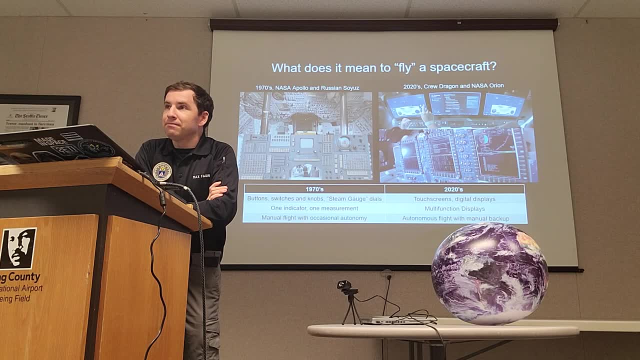 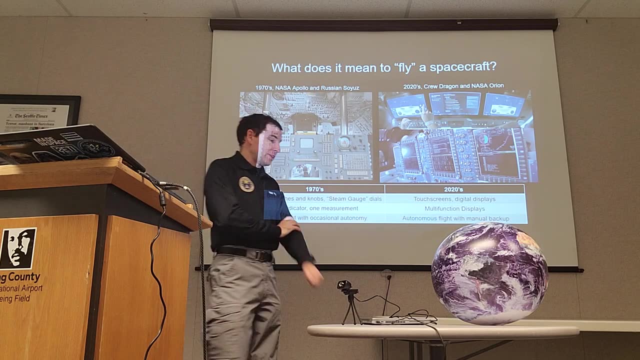 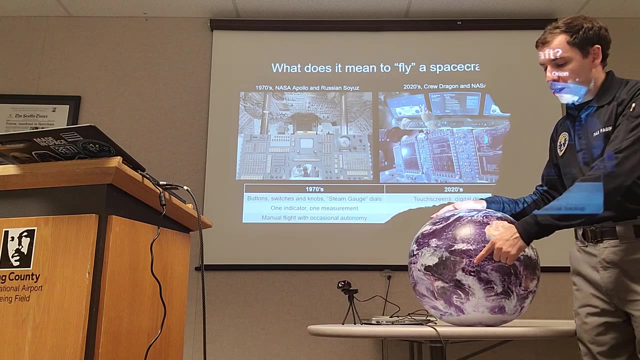 much energy, because what i'm thinking is you just apply a delta v, like that you do across the surface. you do, but it is because of the momentum. you're changing, also your momentum vector. i would say so let's think about a spacecraft in an equatorial orbit. 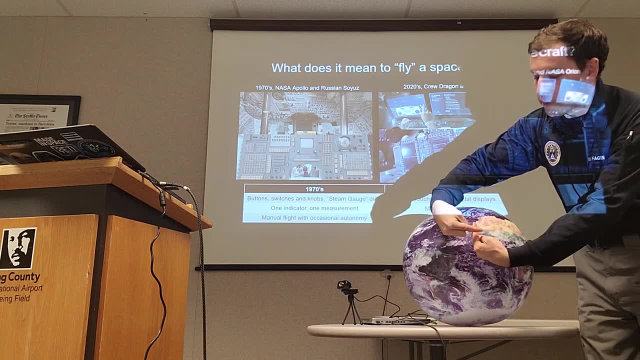 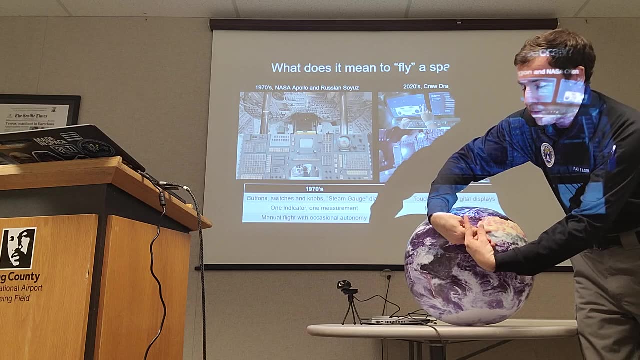 and a spacecraft in a polar orbit when they cross, when their orbits cross right here. think about their velocity vectors. one of them has a velocity of seven kilometers per second due east, and one of them has a velocity of seven kilometers per second due north. To go from an equatorial 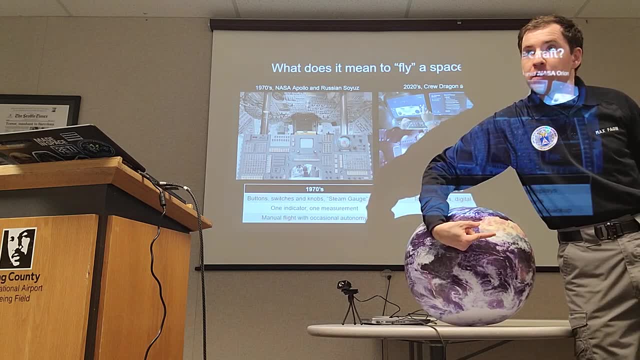 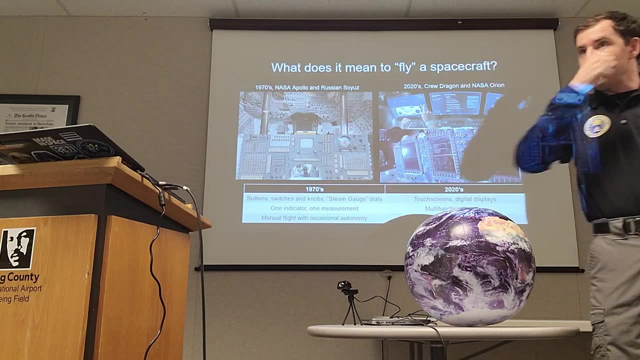 orbit to a polar orbit. you need to take your 7 km per second velocity vector and change it to a 7 km per second due north velocity vector. Think about how much energy it takes to take something that is going this way, at 7 km per second, and turn. it until it's going 7 km per second opposite. like that, It's a delta v of square root of 7 squared plus 7 squared, Which is why it's so expensive. It turns out, actually, that the delta v required to take something from an equatorial orbit. to a polar orbit is about the same delta v as was required to launch it in the first place. So taking something from stationary on the surface to an equatorial orbit, do that again and you can take something from an equatorial orbit to a polar orbit. Which is why the ISS hasn't changed its inclination by even a tenth of a degree since it was launched. It changes its altitude all the time, But not its inclination. To what extent are the Russians still involved in all this? Very involved, For no astrodynamics. 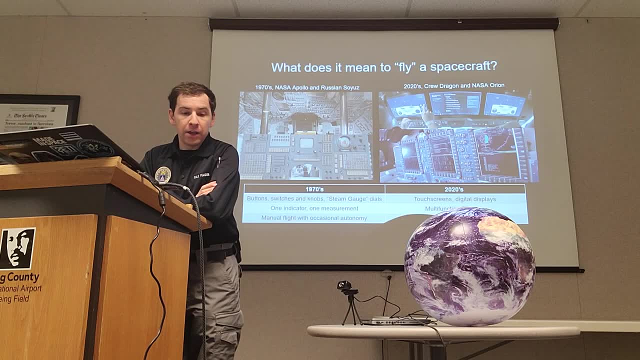 reason, but for programmatic reasons. the ISS was designed to make it pretty much impossible for any partner to leave on that terms. The Russians have made a lot of bluster and noise about saying they're going to leave the ISS program. No one is assuming it's going to happen. It's not technologically possible for them to leave without the consent of the other partners, As it would be impossible for the Americans or the Europeans or the Japanese to back out without the consent of the other partners. If I was able to put money on the subject, I would bet an enormous. amount of money that the Russians are going to stay with the program until the ISS is retired in 2030.. No matter how bad the political situation gets. The program was designed to be immune to political squabbles, No matter how evil one of the partners gets. 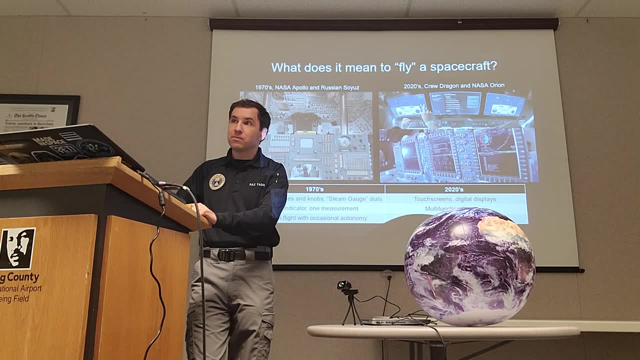 Isn't the Soyuz the only boosting capable craft? No, It was for a time, but currently we have that ability back now with the Cygnus, with the Northrop Grumman Cygnus, But most of the reboosting is still done by the Russian Soyuz, although when it's uncrewed it's actually called a Procress, not a Soyuz. So what sort of teeth to put in the agreements then? So the International Space Station is physically built? 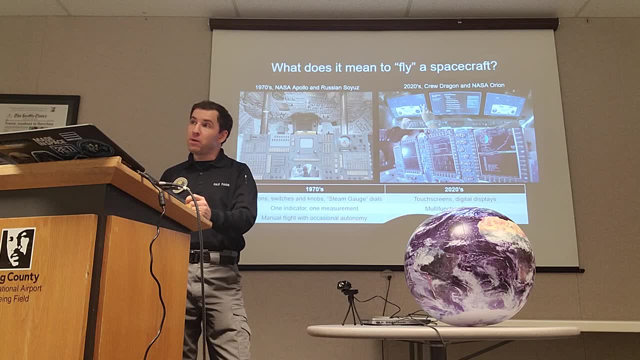 So that the power and thermal comes from the US segment and the propulsion and guidance comes from the Russian segment. So one partner can no more lead than you can keep flying your plane without its engine or without its yoke. It's still very. 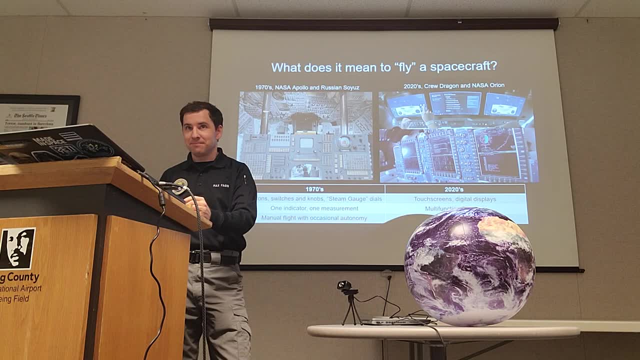 impressive, though, that they were able to craft it in a way that so far has been kind of bulletproof. I'd be curious to read it. That's a diplomatic Yep, I mean, if you actually start listening through the steps of what would have to happen. 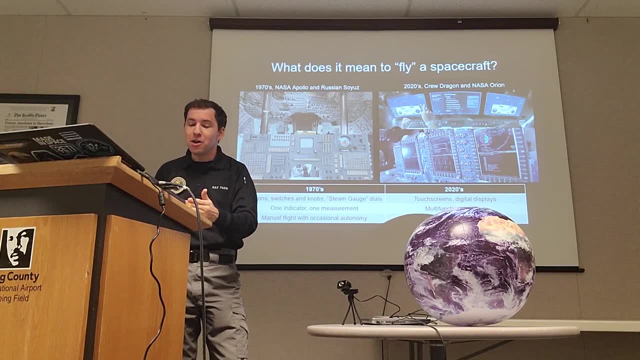 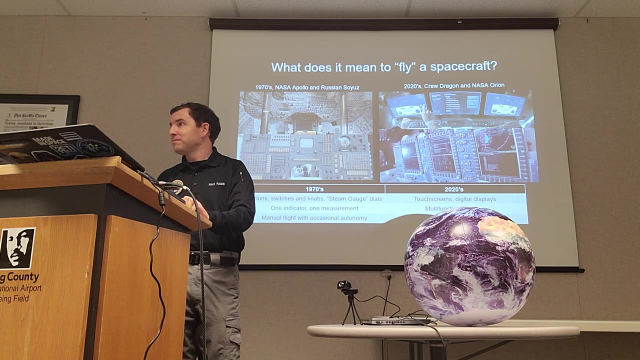 for the Russians to depart the Soyuz, to depart the ISS, you very quickly come to steps that require the participation of the other partners. They can't just close the hatch and press undock. That's assuming the ISS still stays viable. Yes, 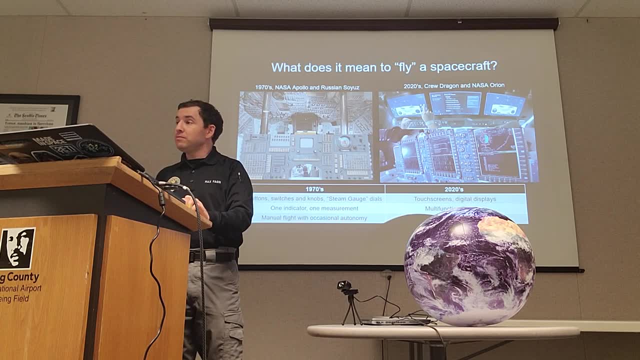 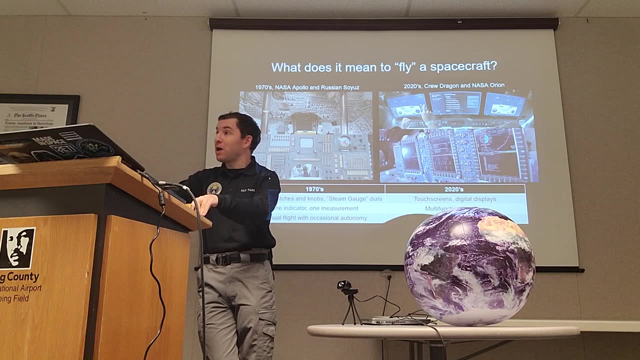 When the Russians decide they don't give a rip anymore, they're gone. That's just it, They're absolutely gone. The Russians leaving would take down their segment as well. They would have to be willing to abandon their segment as well, Statistically speaking. 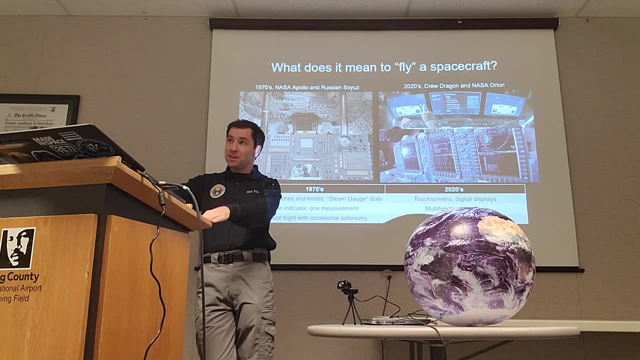 statistically speaking, that's probably the Pacific Ocean. After the Pacific Ocean, it's probably the Atlantic Ocean. After the Atlantic Ocean, it's probably Russia. I'm loading on the Kremlin. Why mess around? Bringing the ISS down in a precise, controlled manner is actually a very large problem that NASA is not yet entirely clear on how to solve. The beginning was the mid-90s. This was very much a future problem, but the ISS partners have put out a request proposal right now, for here are the requirements of a vehicle that can de-orbit. the ISS. Who would like to build this for us? It is a surprisingly difficult problem. It's not something the ISS can do on its own. It's so complex. You can't just. you can start de-orbiting it as it's completed. 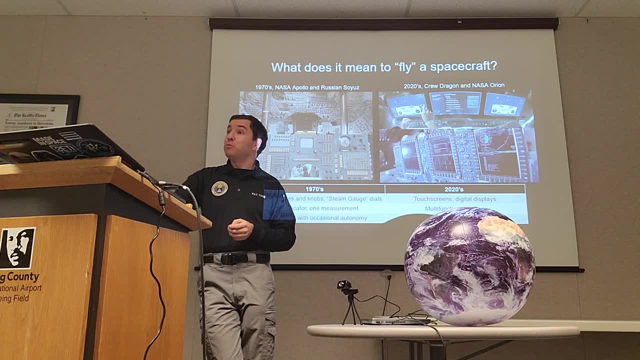 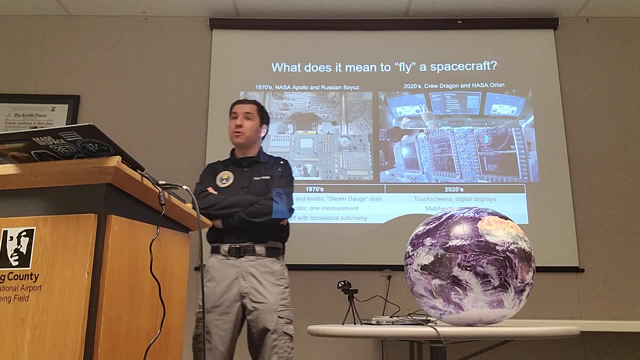 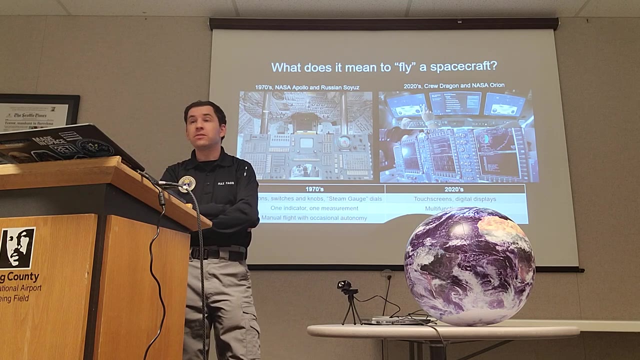 The physics couldn't figure it out. It will come back, but it could come back anywhere between 52 north and 52 south. That's the China way to do it. It comes back, It comes back. But we're confident that the ISS components on orbit as is. can last through at least 2030.. NASA, officially, is not planning to start retirement operations in 2030. And, if we're being realistic, there probably will be an extension. We're talking about the Chinese one. It was like two years ago, right? They let it go. Yes, that was Tiangang 1. And they did this. The Chinese default position for upper stages is to not have an active de-orbit mechanism. Under the international pressure, I suspect that will change in the upcoming. years to decade There is even without an accident. they are rolling the dice every single time And it is not a good look if your nation crashes something on another nation. So the Chinese have just recently reached the primary assembly stage of their spacecraft, their space station. 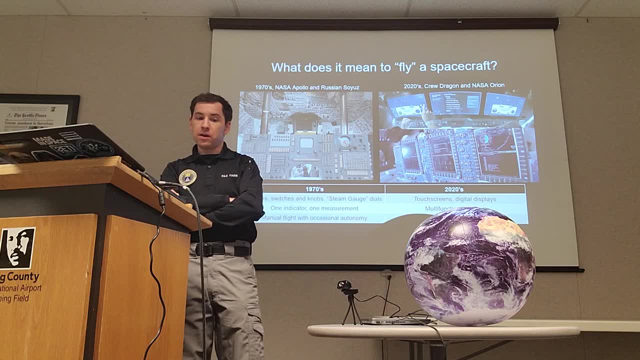 Tianzong. The second one, The second one. yes, There are three taikonauts on board right now And I suspect in the near future they will, you know, cave to the international pressure of, if the 21st century. 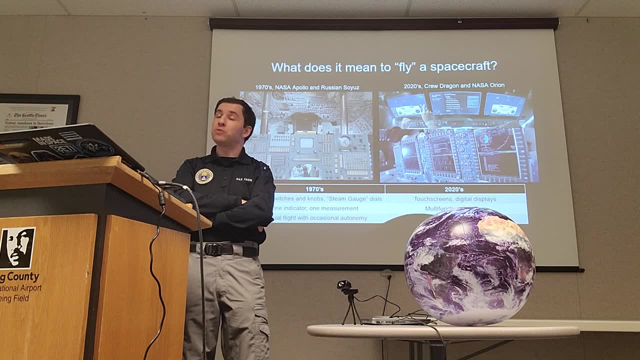 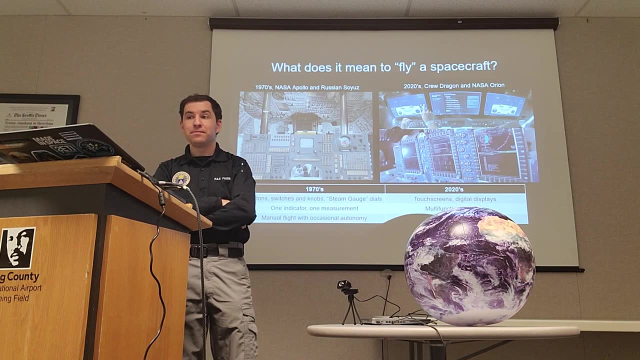 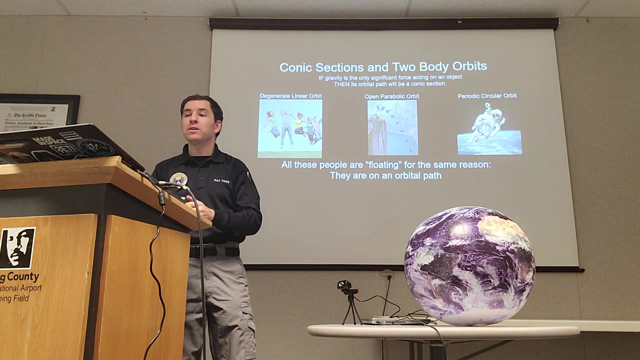 stopped crashing your rocket bodies at random points on Earth, But it's going to take time. I'm still sorry. on Mars They don't have a plan for space station, Never did. We'll deal with it when we get there. We know what a vehicle has to be capable. 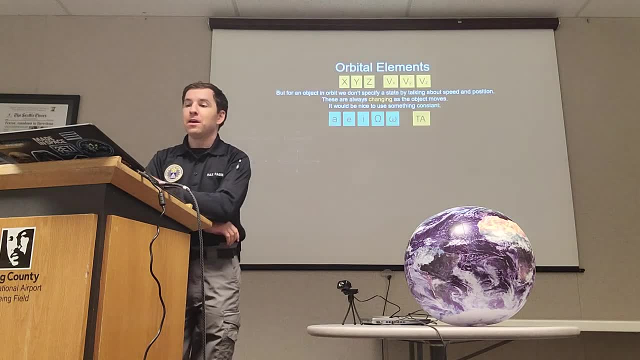 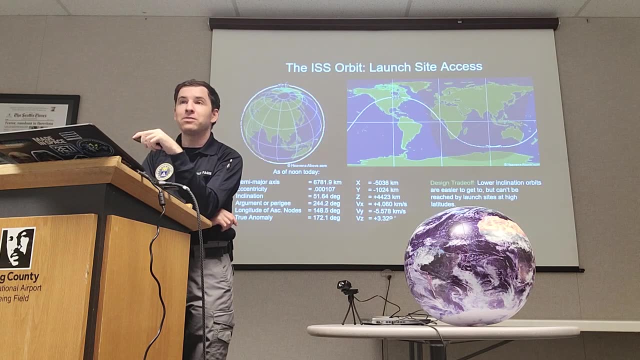 of doing in order for the Earth to be able to come down here, Right? So like statistically even bringing it down in an ocean Right now, if we completely passively deorbited the ISS, it's a three out of four. it's coming down. 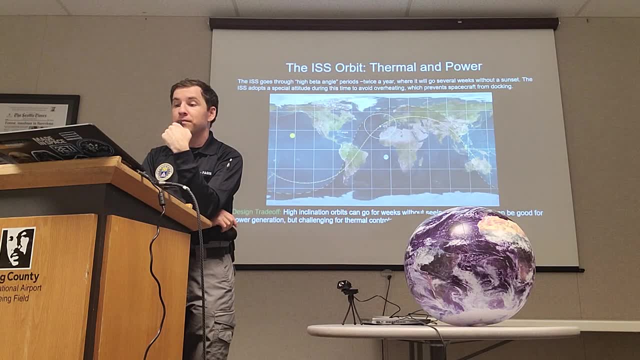 in the ocean, But one out of four it could come down somewhere on Earth. But in a large organization everyone wants to do something cool and neat and exciting. And who wants to take on the lead of deorbiting the space station 30 years from now? They're going to be sitting in a little. 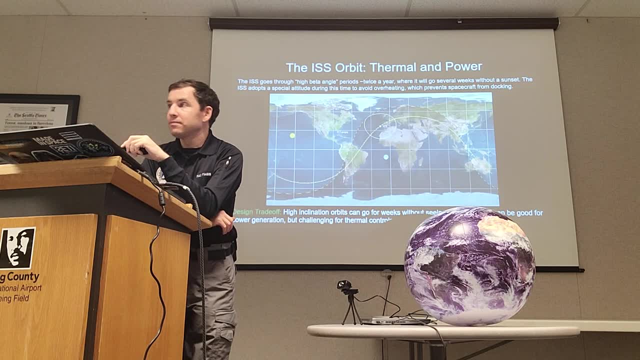 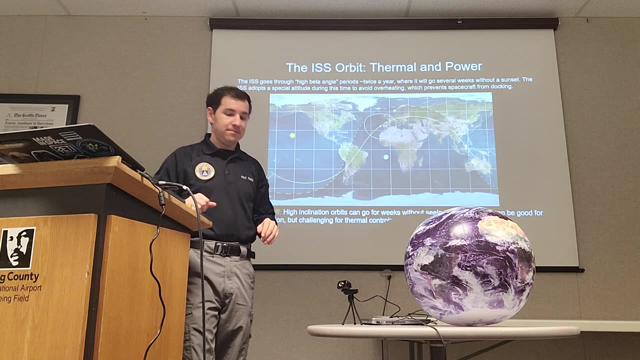 office in a corner and talking to no one. No, no, I want to do something else. I see it more as like: do that all the time? I mean, look at the hand for like nuclear and say, well, we've got to build this. 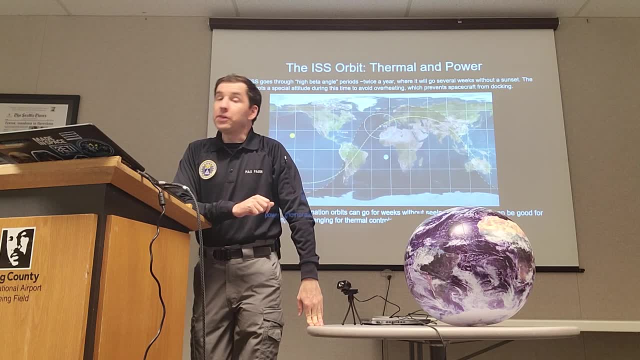 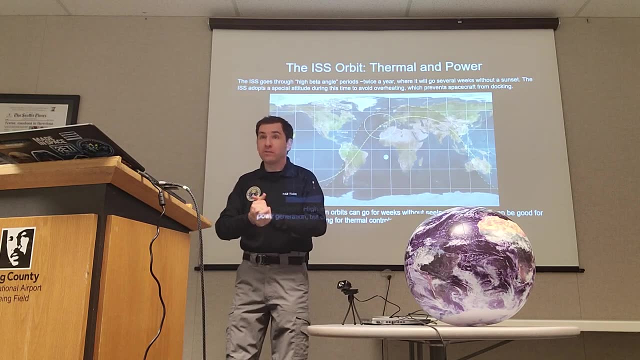 Yes, that's true. But this is why we hope to build Orbital Reef and all the commercial LEO destination competitors, not just Blue Origin. That's why we're intending to build Orbital Reef, So we can transfer all the stuff that's on the ISS, all the experiments. 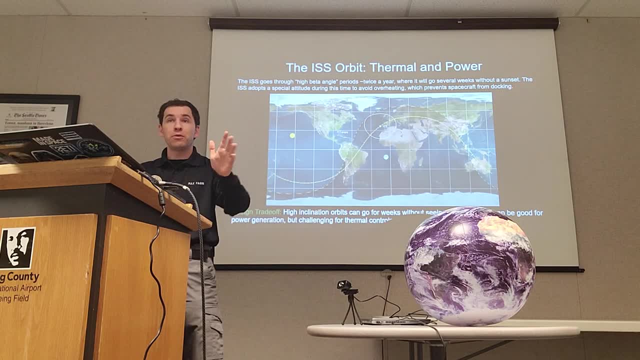 that don't want to be interrupted. We can transfer those services and distribute them to commercial space stations. so NASA can feel free to deorbit the ISS, So all the partners can feel free to do it. Orbital Reef is the name of Blue Origin's proposed space station, But we're not the only one. Axiom has its own space station, Nanoracks has Starlab, Northrop Grumman has basically a LEO version of Gateway. There's multiple commercial space stations being proposed to take over for the role of the ISS's. 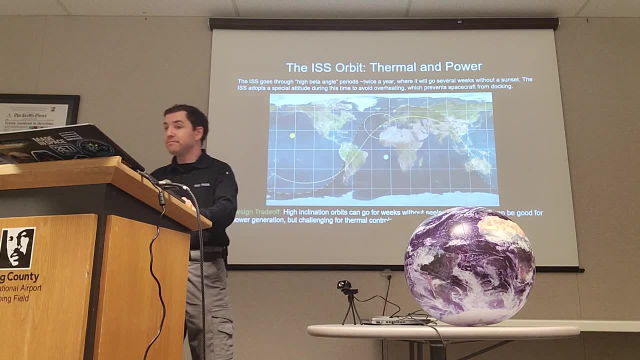 drill exit in the next 30 years? Go ahead. I have another question. So you're saying that if I've got a true mission, I have. effectively it's a collection of, and then you basically have events where you transfer from one world to another. Pretty much. Why so, instead of running the engine sort of odd for a short period to change, why not just distribute it and just have a lot of for a really long time and just effectively average it out? Is that even possible? Because then you stop microgravity. 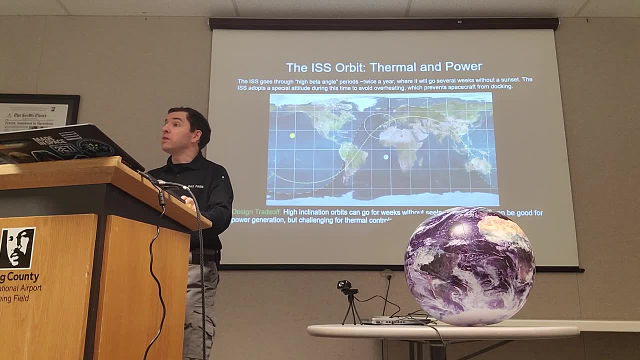 We can and do do that. We don't do it on the ISS, But any spacecraft, any satellite that's gone to GEO in the last 20 or 30 years has done something like that with an electric engine. So those types of engines are very low thrust. They're very high performance. They can do the same thing for one-fifth of a propellant. But they have thrust measured in fractions of maneuver. It's a very, very small thrust. So it takes them a long time. It takes them a long time.